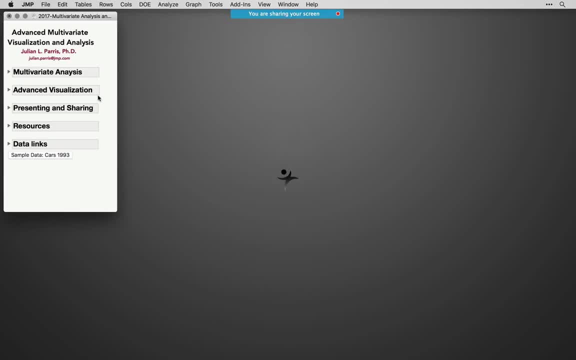 meaning of those analyses, and especially when you're trying to communicate the meaning to new students, And so, of course, this is a webinar in our academic series, and so I expect that many of you will be teaching these concepts, And so I definitely want to put an emphasis on visualizations. 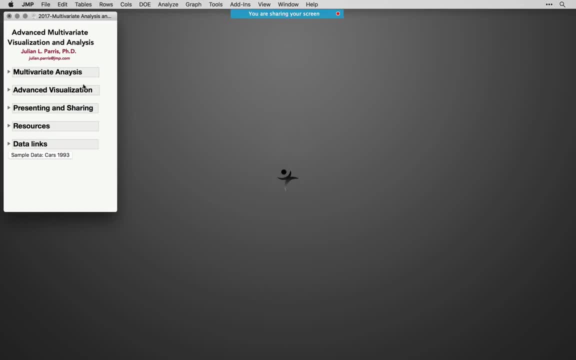 that are great for explaining the concept behind analyses, And so let's take a look at which analyses we're going to be talking about, And so I'm going to take a look at some of the analyses. I mean, I'm going to be talking about analyses that live under the multivariate platform. 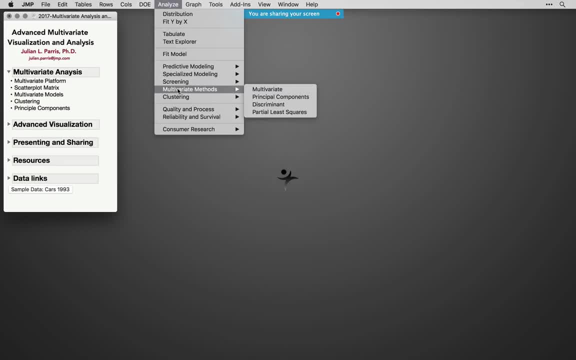 If you're new to JUMP, that's going to be under Analyze- Multivariate Methods- And that will encompass a number of things such as correlations, in fact, even principal components we can get to from inside of multivariate. We'll also see visualizations come about just by using the 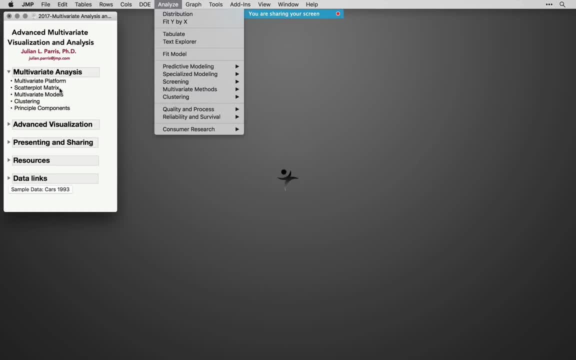 multivariate platform. We're going to look at the scatterplot matrix. it's actually under the graph menu and that gives us an option of producing scatterplot matrices in a specific way that I want to show In a way that I think is quite handy. 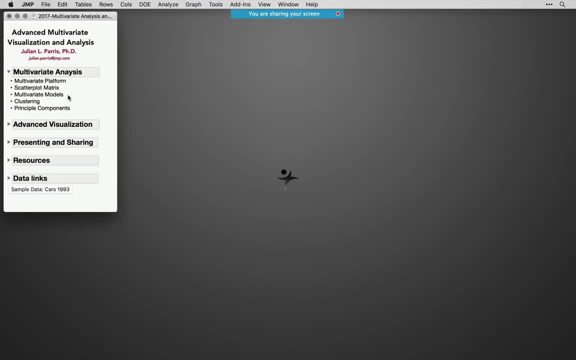 We're going to look at multivariate models, and so this could be things like a multiple regression, could be a multivariate analysis of variance. Many of these will live under Analyze Fit Model, and that's a place we go in JUMP often when we're working with more than two variables. 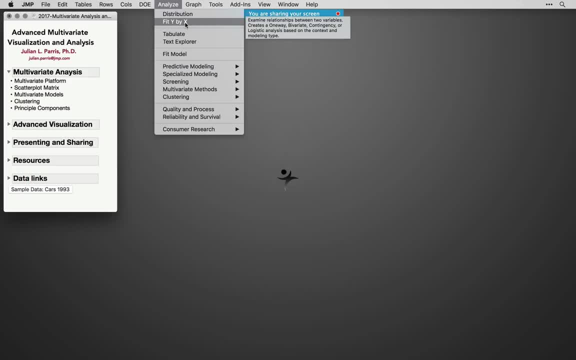 Many of you who are familiar with JUMP know that Fit Y by X is our bivariate analysis platform and Distribution is our univariate analysis platform. So Fit Model is a place we'll go for a lot of multivariate analyses And we even have some specialized multivariate methods that live under its own menu. 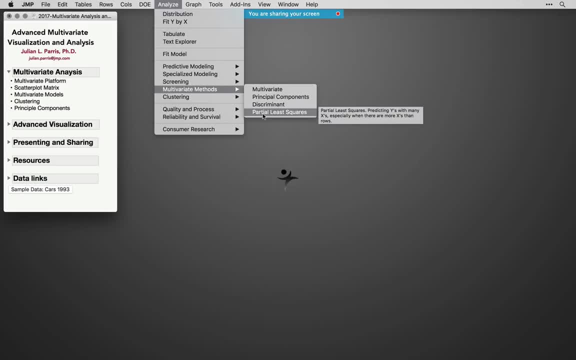 things like principal components, discriminant, partial least squares and even clustering, so methods of unsupervised learning where we can cluster rows in our data set, And so we'll look at those analyses and we're going to look at certain visualizations that come. 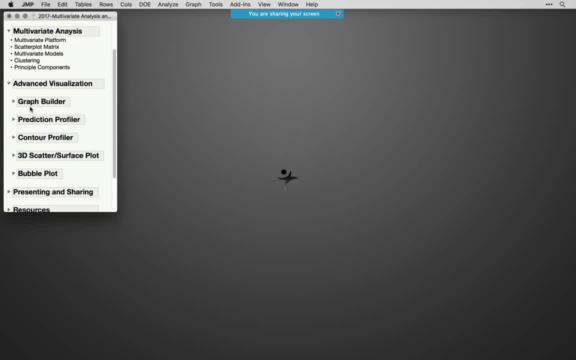 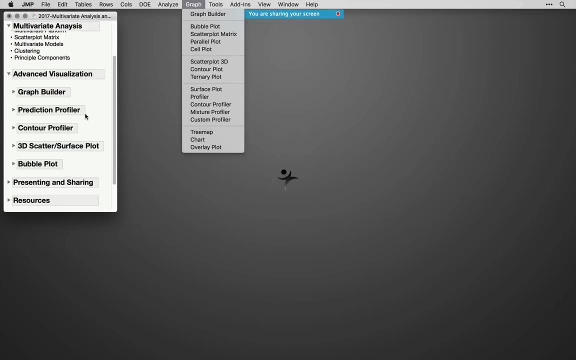 about by using them, And I'm going to show you how to create more advanced visuals using Graph Builder, a wonderful drag and drop graphing platform. under the graph menu, We're going to look at the prediction profiler, the one that actually comes built in with Analyze Fit Model analyses as well as profilers. 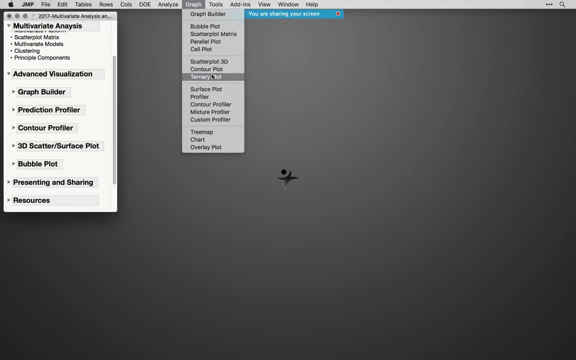 that we can get to directly under the graph menu, And so there's actually a bundle of them here. So the straight profiler, the contour, the mixture and the custom, And so we'll look at a few of those. I definitely want to show you the 3D scatter and surface plots. You know, 3D gets a bad rap. 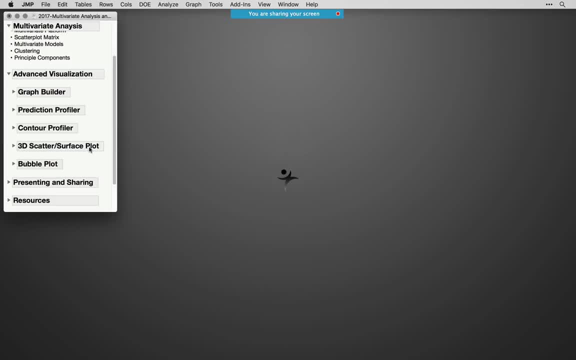 but in JUMP 3D, scatter plots are interactive, which really lends something to their ability to convey the meaning behind the data points. So we're going to look at those and then we're going to look at a really fun and really useful. 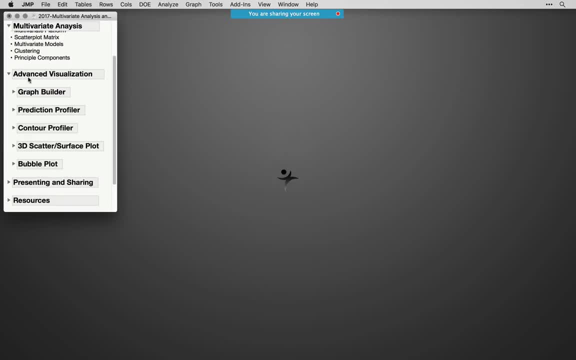 multivariate visualization technique called bubble plots, And so those are the visualizations we'll see. As I'm going along, I'm going to point out things that I think are very valuable for presenting and sharing your visualizations and your analyses. Specifically, we're going to combine some of our 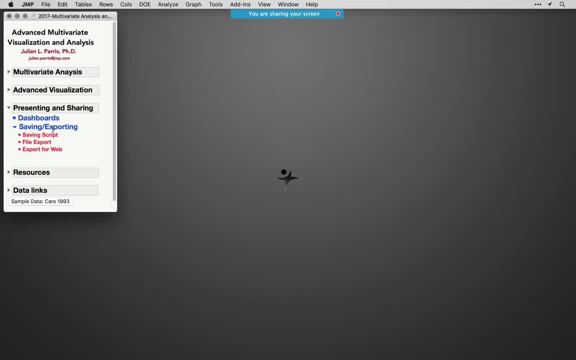 outputs together to make dashboards, and I'll point out how we can save or export particular visualizations and analyses, Because, of course, we're not simply creating these visuals and images for ourselves. usually We need to share them with others. At the very end, I'll point 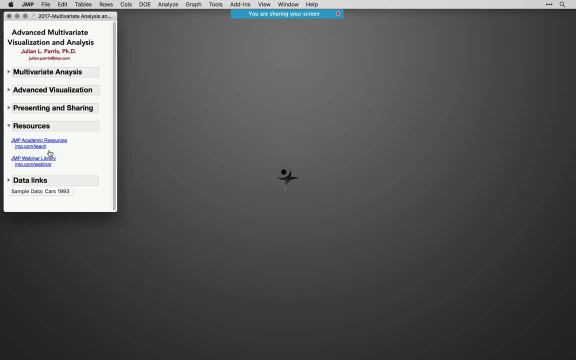 you back to resources, and even at the start I'll mention jumpcom slash teach, a great place to go with all of our teaching materials, and jumpcom slash webinar, which is the place you'll go to find the recording of this webinar and many other webinars. 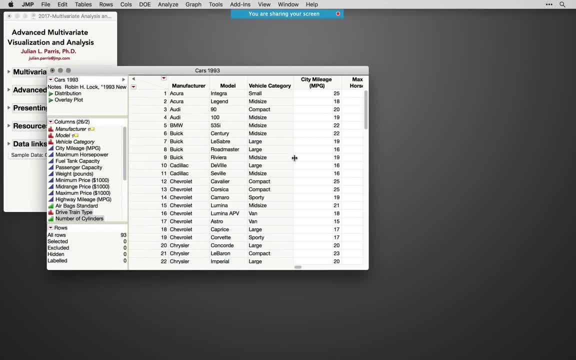 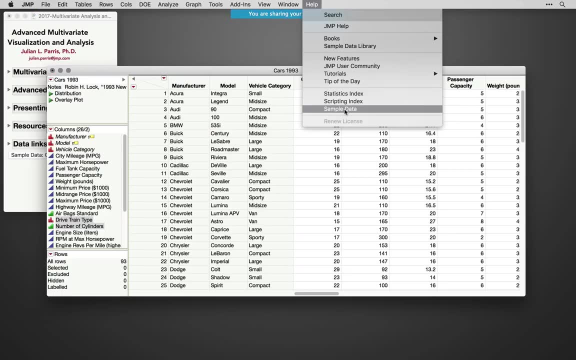 So let's get started, And what I'm going to use is a sample data set that I quite like in JUMP called CARS1993.. And if you're new to JUMP, you can get to all the sample data by going to the help menu and going to sample data. 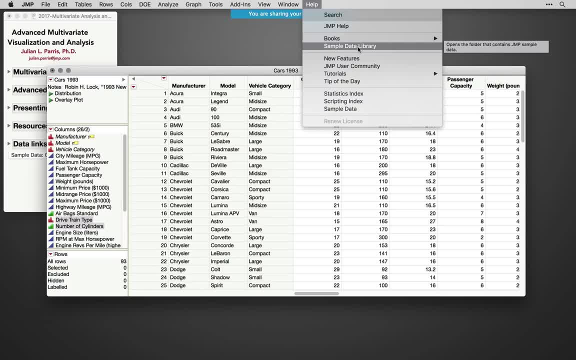 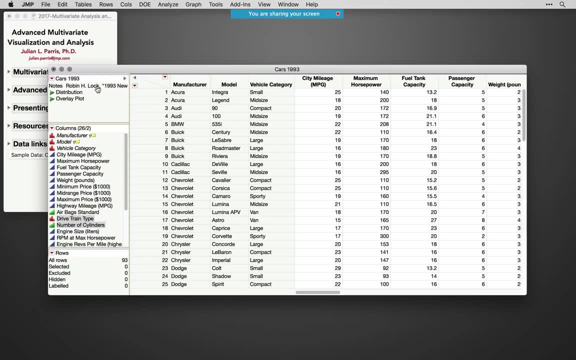 You can also go to the sample data library, which will open the folder that all the sample data lives in on your computer. So let's orient you to the data set first. CARS1993 is this data set from Robin Locke's paper in Statistics Education. and these are new cars in 1993. 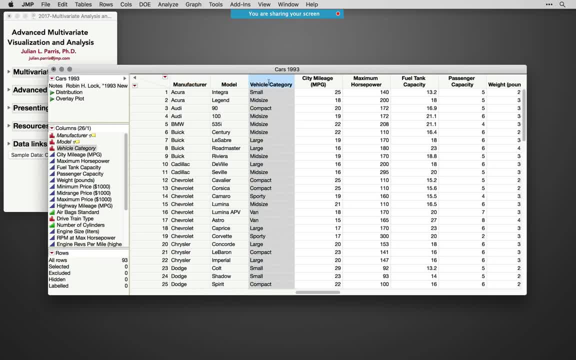 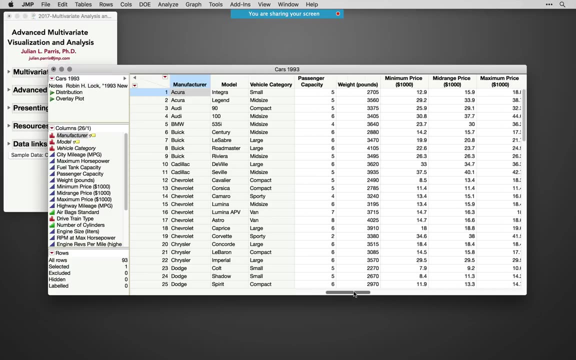 with many attributes of them. So we have things like manufacturer model, the vehicle category. We have several numeric columns: city mileage, horsepower, fuel tank. We have the minimum and maximum price of cars in that category. So for an Acura Integra, for instance, which is a small car, you can see that the minimum 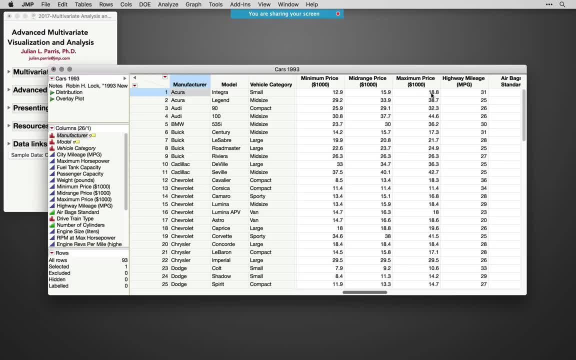 price in thousands was $12.9,000 and $18.8,000 for the maximum. So that's in the model class. So we have a good number of numeric variables that we'll be able to use when we enter into these multivariate analyses. And I'm going to emphasize numeric today, although of course 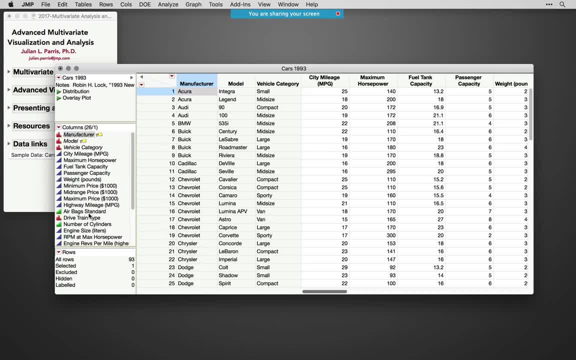 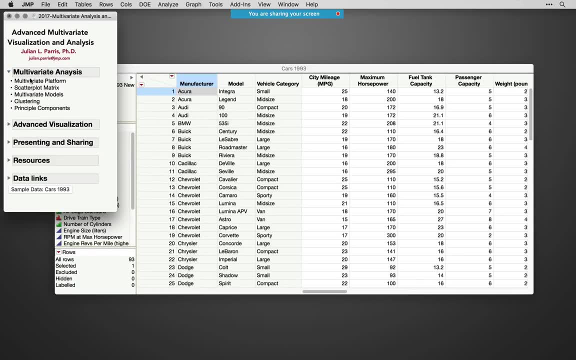 multivariate analyses can also incorporate qualitative variables- What we'll say in JUMP. but we're going to start with a platform that explicitly requires numeric variables, Variables that are measured using numbers and numbers that actually mean something on a numeric scale. So let's start off with the multivariate platform. I'll go to analyze. 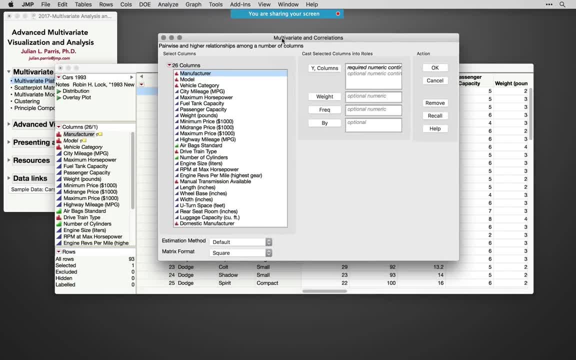 multivariate methods multivariate And you'll notice that I haven't even started out with any real predictions about these data. I'm not trying to model the outcome of anything in these data. The multivariate platform is really about looking at the multivariate relationships. 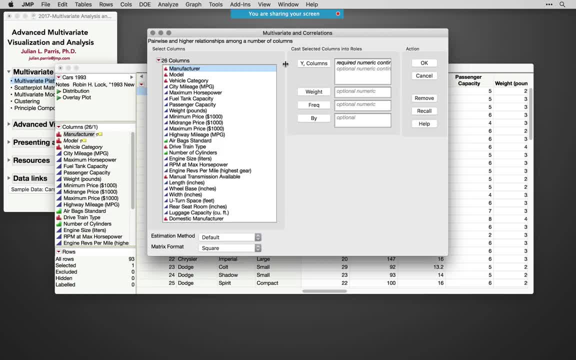 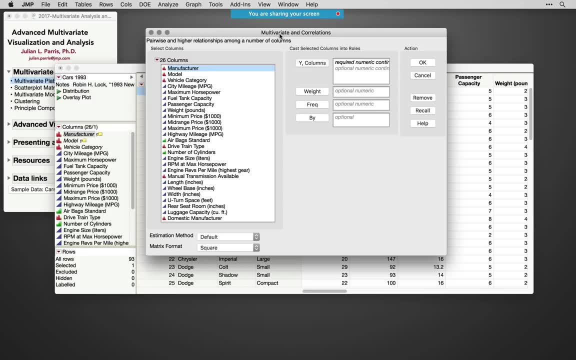 variables, And so not with an explicit eye on how to predict one thing in particular, but how the variables relate to each other And multivariate is an excellent place to start when you're investigating the predictor space in a data set. If we did have something, 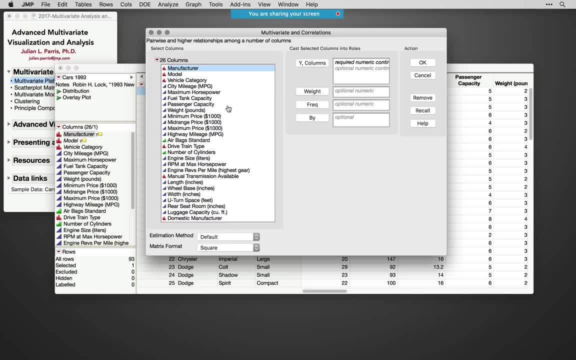 we wanted to predict. we could use it here as well. But especially if we're interested in how our variables just relate together in their own space, multivariate is a great entry point, So I'm going to start with the first five variables here. So the mileage and MPG that. 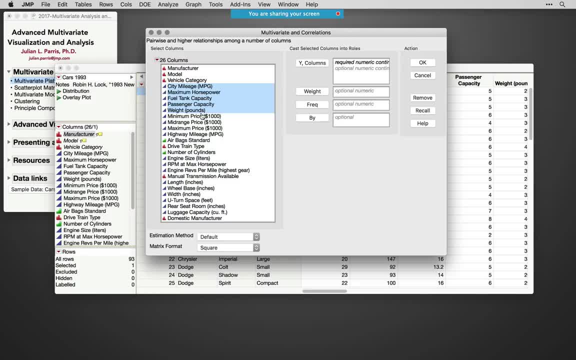 we're going to be looking at is the mileage, MPG, horsepower, fuel tank, passenger capacity and weight. To enter these into a role many of you know we can click Y columns. I could have also dragged them over. We have additional options we're going to come back to in a minute. 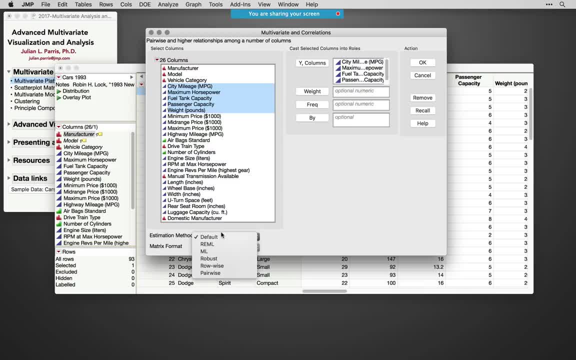 how we can estimate these multivariate relationships, especially when in the presence of missing data, and how we want the matrix organized. And so this is how the scatterplot matrix will be shown. I'll leave everything on the default and click OK. Jump starts out by showing: 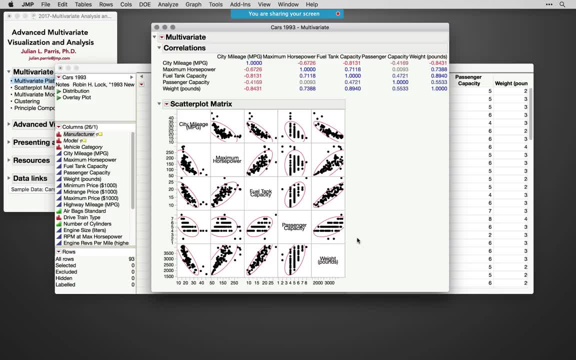 us the correlation matrix. So let's take a minute to look at our default and then we're going to look at other options we can get under the red triangles: one for scatterplot matrix and one for multivariate. So first the correlation matrix. If you haven't seen a correlation matrix before the diagonal. 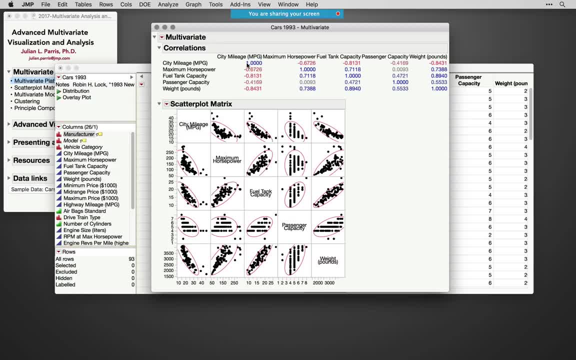 is showing the correlation of each variable with itself. Obviously it's going to be positive one, And the off-diagonal points are the correlation at that intersection. So negative 0.6726. here is the correlation between city mile and city and the maximum horsepower, and so a negative correlation indicating that. 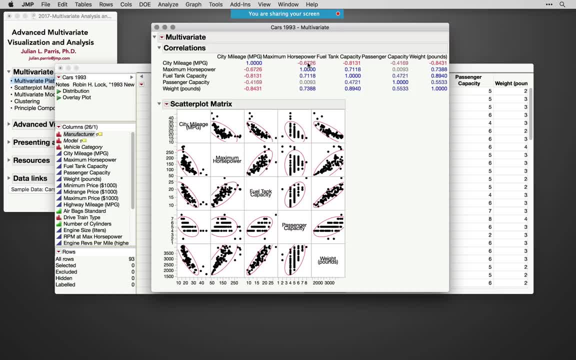 increases in one variable are tending to be associated with decreases in the other. so we can say, among these cars we've sampled, those cars that have more horsepower tend to get worse city mileage. okay, not a mind-blowing thing to find, of course, but that is actually the correlation coefficient for that. 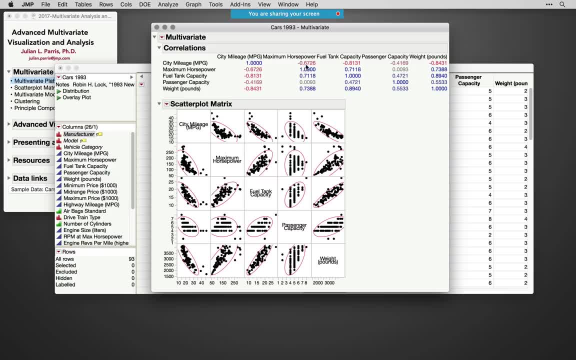 you'll notice that same correlation coefficient- negative point six seven two six- is here as well. negative zero point six seven two six. I saw an error on jumps part. it's just the fact that the intersection also occurs between horsepower and city mileage on this column, and so basically one side of the. 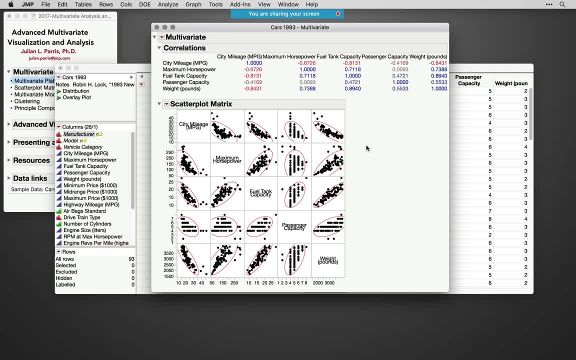 off diagonals is a mirror of the other, and that's just how correlation matrices read, and so if you've never seen them before, that may have caught you off guard. you'll notice that the values are colored by the magnitude of their correlation. positive correlations are blue, negative. 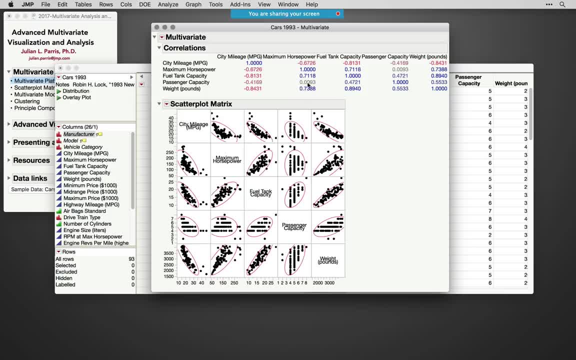 correlations are black, negative correlations are blue, and then the positive correlations are blue, negative correlations are red. so the Correlations are red and the degree that they are dimmed is relative to how close they are to zero. A zero correlation means no linear association between the variables, at least within the sample we have. 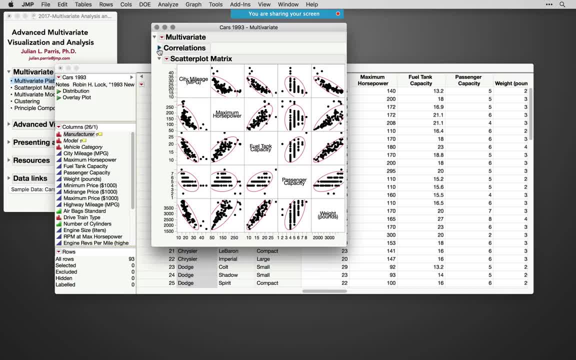 All right, so that's our correlation matrix. I'm going to minimize this temporarily, which I can do with the gray triangles, And let's look at our scatterplot matrix. So, as I had in the correlation matrix, the diagonal here is one variable with itself. 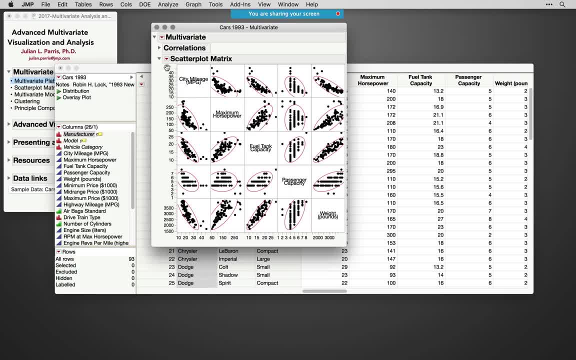 And there's actually nothing shown in that diagonal. If you like, you can turn on something there which I quite like, which is under the red triangle showing histograms, And I'll do a vertical histogram And so vertical histograms, and jump show for the axis on the Y those observations and where they occur. 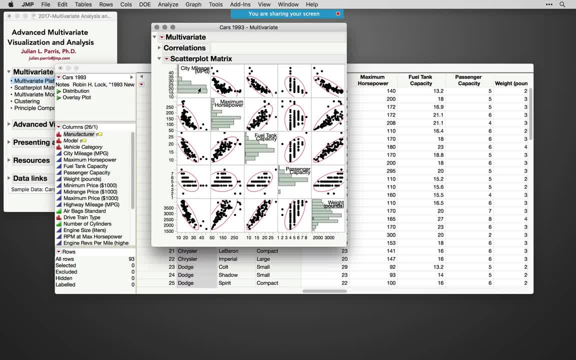 So you can see the city mileage is sort of skewed positively. Most cars have a city mileage around 15 to 25 and a few quite far up, And so that diagonal, since it would only show one variable with itself, this is a nice way of making sure that we have a diagonal. 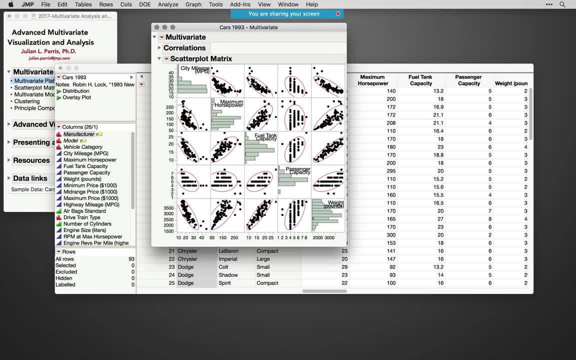 Let's check out the off diagonals, Just like we had for the correlation matrix. the variables will show in two places the same relationship, except it's going to swap the axis. So let's look at this right here. So city mileage is actually what's on the X axis here. 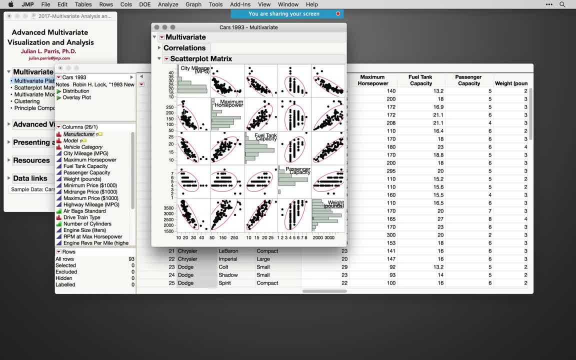 That's the scale right here at the bottom, And the Y axis is maximum horsepower. So this is the city mileage by maximum horsepower. scatterplot Up here. Even though These are the same data, Notice the axes have been switched. City mileage is now on the Y axis. 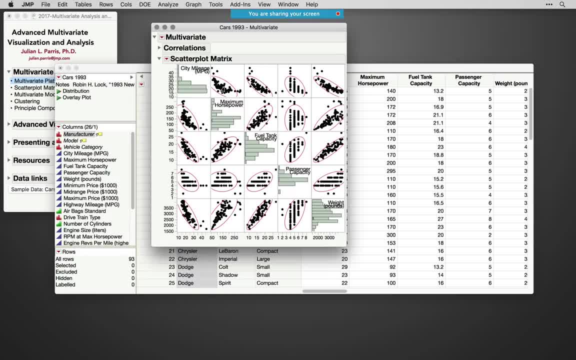 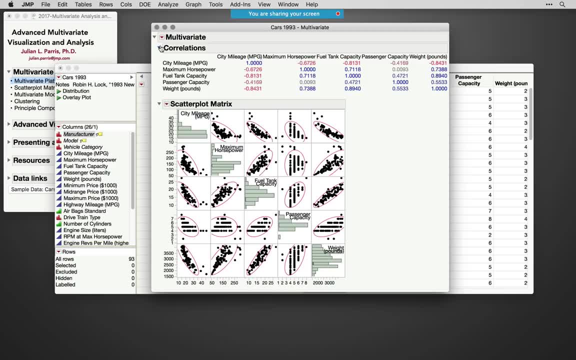 That's what these points are If you map them over to the Y and horsepower is on the X axis. So, like in the correlation matrix, we have somewhat redundant cells. However, in a scatterplot matrix they're mere images, that are, they're flipped in terms of the axes. 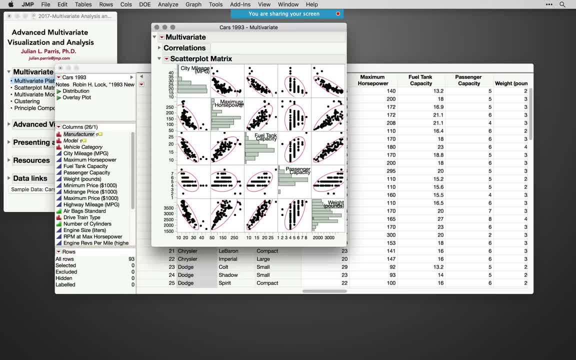 And I find this to be quite useful. Sometimes it makes more sense to think of one variable on the X axis than the other. Notice that we also have density ellipses. These are showing the relationship. again, just like the correlation, They're showing the magnitude of linear association between these two variables as the density ellipses get tighter. 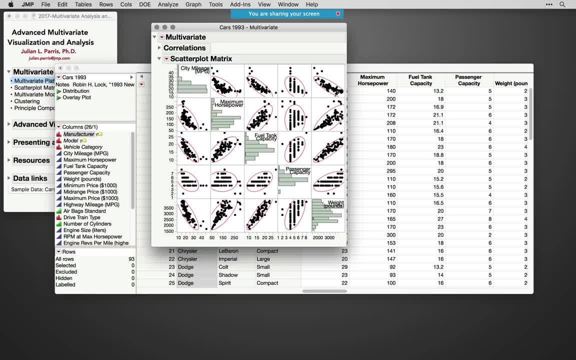 So the minor diagonal, as that gets smaller relative to the major diagonal, then this is a larger correlation, either more positive or more negative. Remember, negative correlations can be just as strong, but in the negative direction. So these give you a very quick way to assess the correlation between these variables. 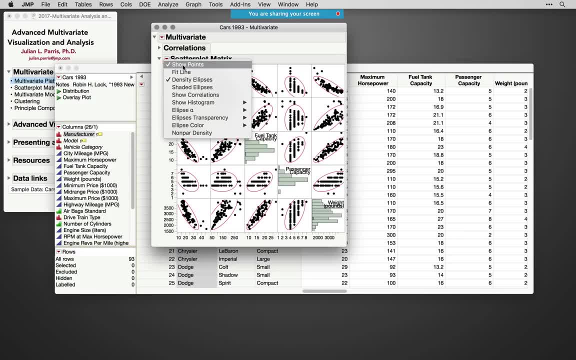 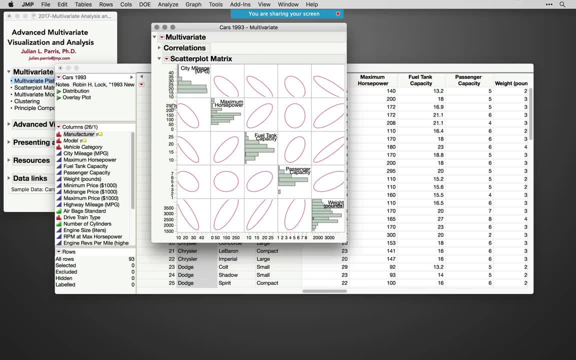 And, in fact, sometimes, when you have lots of variables, the points don't even add much, And so I can uncheck, show points And, as you're thinking about this, if you're building a visual, especially one that you may want to publish, there may be things you want to change. 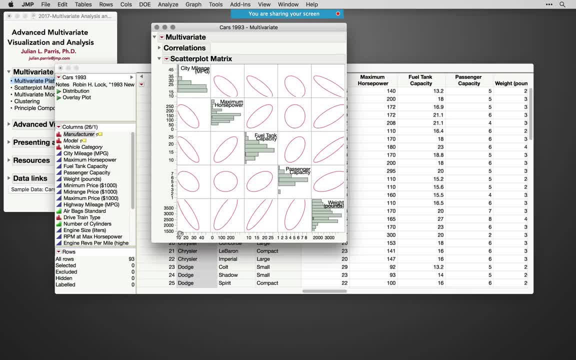 Notice I'm hovering my hand and moving the axes just to to get all these circles or the ellipses to fit on the screen. So our customizations here can play a big part in how we present our data, And so think about using these visuals- visuals even though they're part of an analysis platform. 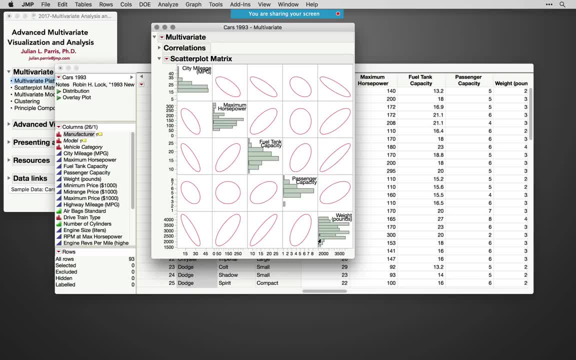 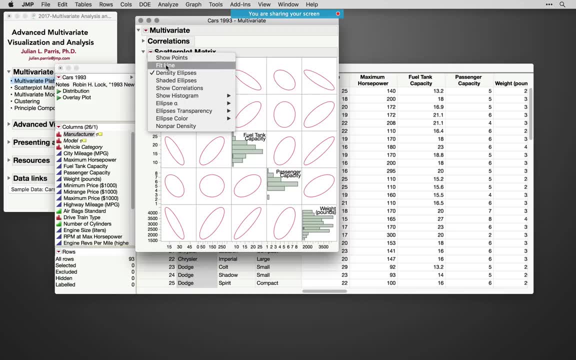 As a way of communicating relationships in the data. All right, So that's just the basic scatterplot output. Let's look again under the red triangle. There's some other things you may like fitting lines. If I fit lines for each of these and turn off the density ellipses, this is the linear regression of the Y variable onto the X variables. 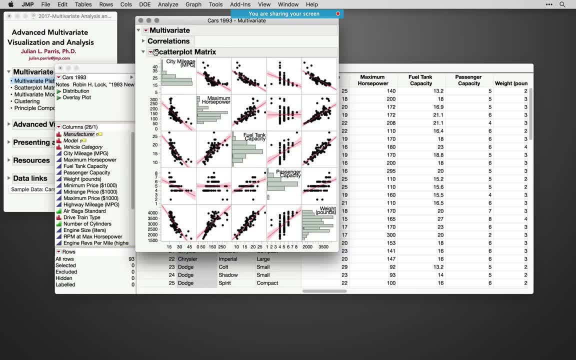 I could turn the points back on even and have those lines. You can see they. they go through the cloud of lines. You can show the correlations actually on each of these. This makes for another nice visual. So you can see the lines. So you can see the lines. 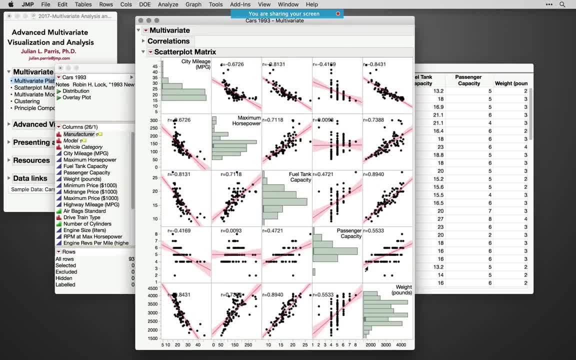 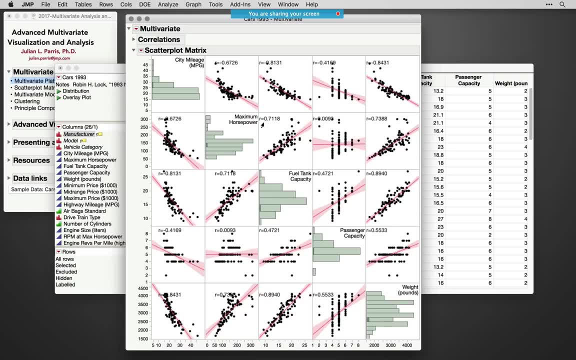 If I drag out the size of these boxes, remember they're all going to stay equal sized And so I can drag any one of them. I like to make them square, just to make sure that we have a nice square output here as well. 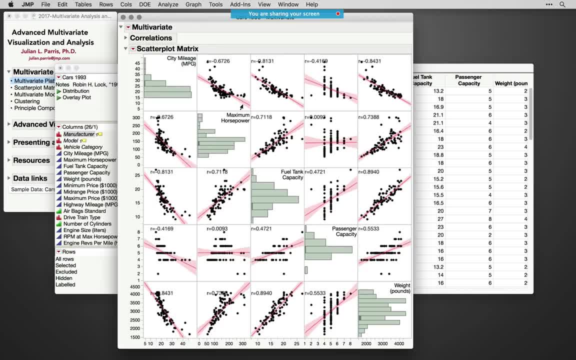 But this gets us to the point where this is actually turning out to be a pretty useful visual One we may want to show people, especially if we're reporting in a paper or showing in a class relationships among variables. So while we're keeping this open before we do anything else, I'm just going to hop ahead and talk quickly about how we might use this. 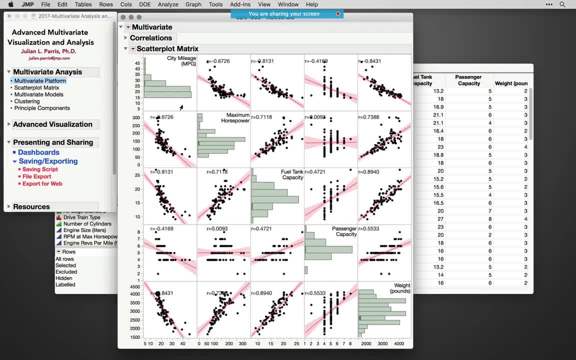 I'm just going to hop ahead and talk quickly about how we might use this So we might get this out of jump. Of course, this isn't the only place we might want to show this, And so of course, we can do file export on the Mac file. 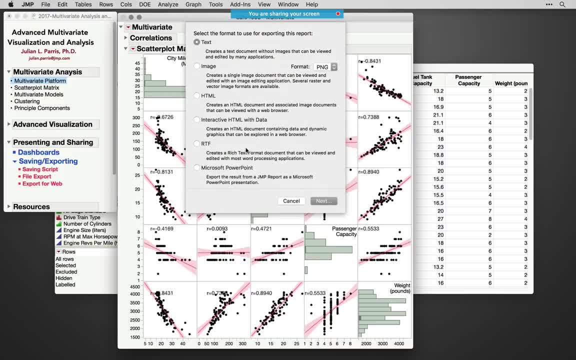 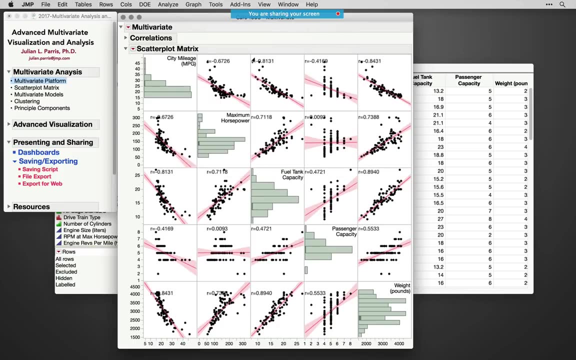 Save, as is what you would choose on the PC, and this will give us lots of options for how to get this particular output directly out of jump. We can even save it as interactive HTML, if we like, or simply as an image, And you have different image types you can export as. another option under your tools menu is to use the selection tool. 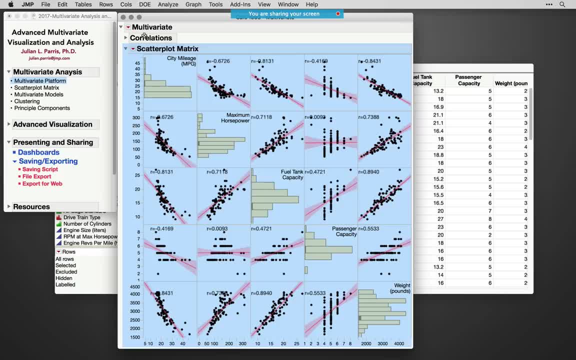 tool, and this is one of my favorites. you can simply click on a particular outline box or even the overall output, and that'll let you just use file or edit copy. when you do edit copy, this again then gets copied to the clipboard. if I were to go to Adobe Acrobat, or even on the Mac I can go to- 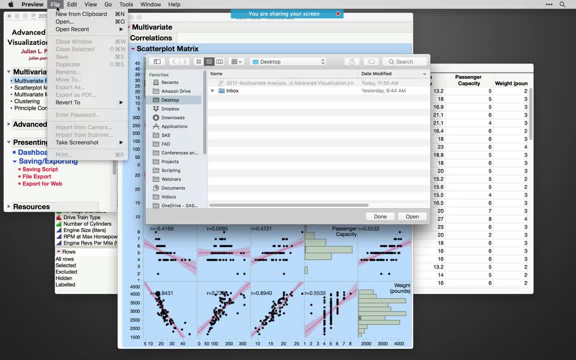 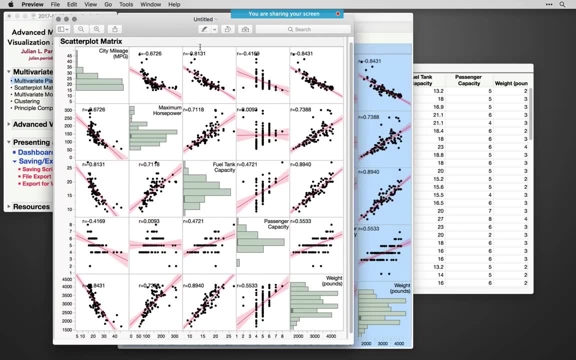 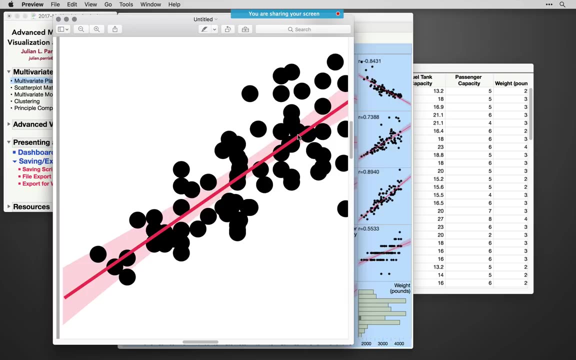 the preview app and do file new from. let me do file new from clipboard. this will actually open this up and now my preview app. so this is something I can save out. in fact, this is even saved out as a vector graphic. I can zoom in and notice that there are no pixels to be found. these: 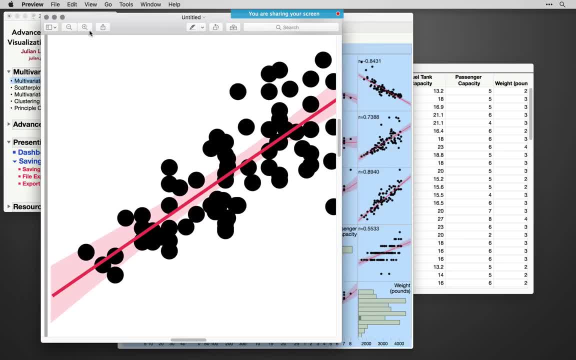 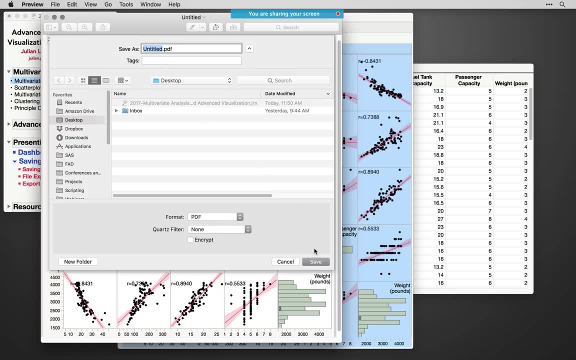 are actual little objects. these are objects that can be edited if you had a vector graphics program and so, as you're thinking about creating visuals here, I'll just save this to my desktop here. as you're thinking about creating visuals, remember that once you've created something in jump. 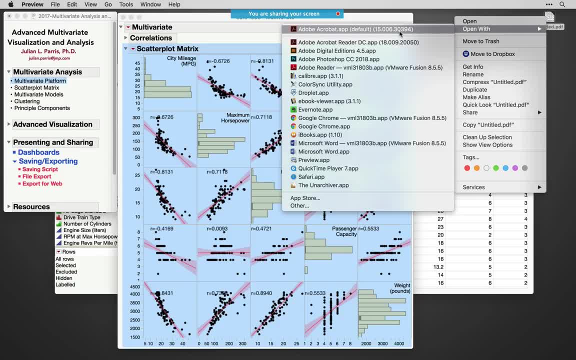 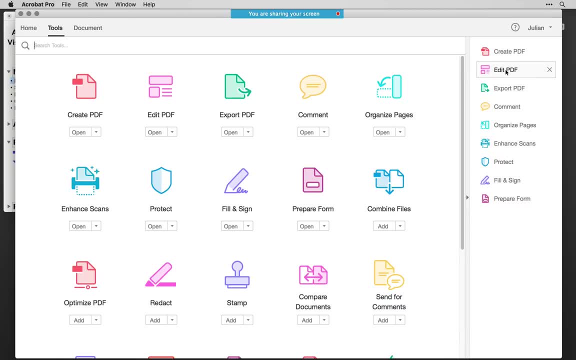 that's not the last place you can use it, and so I'll open this up in Adobe Acrobat. whatever your favorite editor is you can use, but I'll I'll. let me just go to tools here, click edit PDF and notice that these are all little objects. so if I 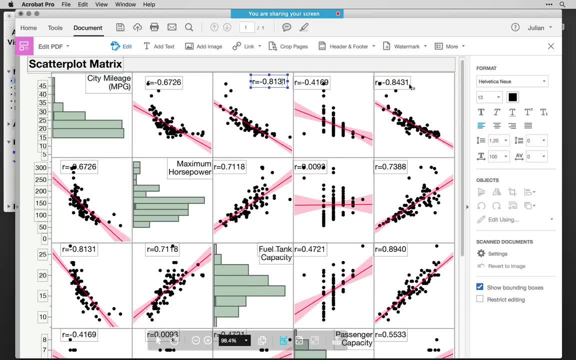 didn't like that. it put that correlation there. I can simply move it over. so every one of these is infinitely editable, and so keep in mind, as you're creating your own visual statistical software, whether it's jump or any other software- will only get you so far if you are customizing a graphic, for. 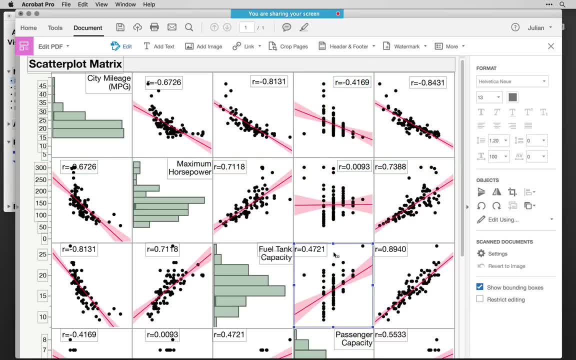 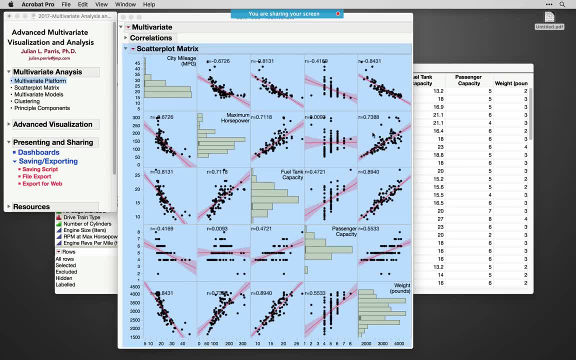 a very special publication or very important purpose, remember to go and make edits to customize it exactly the way you want it to be, and so that's what I'm going to do here. I'm going to go ahead, and, and so I'm going to go ahead, and. 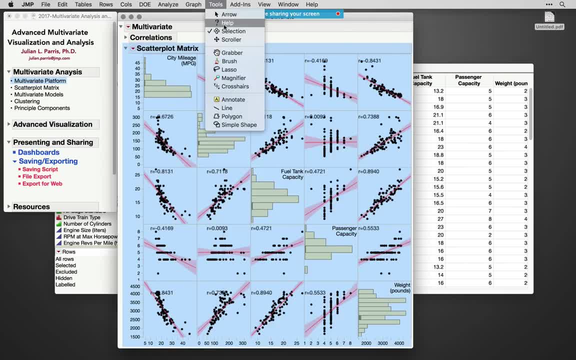 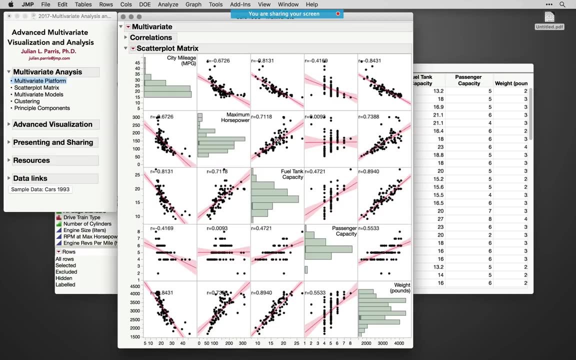 play around with them and see what happens when I want to take the options on. so again, just a back step to where I got, to that from using the Selection tool and jump selection. I simply copy that out from jump using edit-copy and I'm smart enough to take that out as a vector. wicked, so going backwards, the multivariate platforms so far give a sort of an insight into how these variables 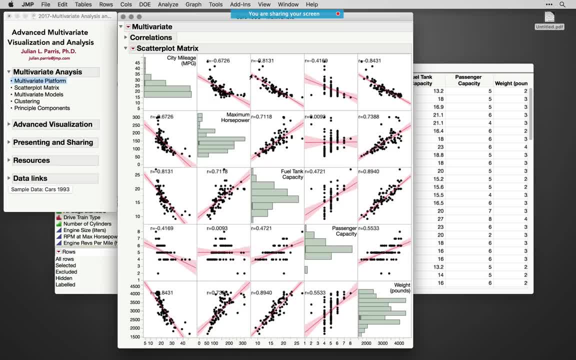 relate to each other and we already saw one kind of expect the relationship. cars with more horse power tend to get worse mileage. similarly, cars with bigger fuel tanks- while the big fuel tank sort of tacos- Yeah, with a slightly different impression of that- tanks tend to get worse city mileage. Probably that's because cars with bigger fuel tanks have more horsepower, They have to make up for the fact that they get poorer gas mileage, And maybe we see some things where we didn't expect a relationship. Cars with more passenger capacity don't tend to have more or less horsepower, Although there are a few points here of cars like the Chevy Corvette. 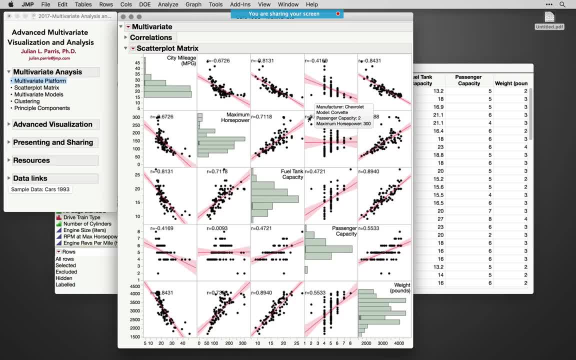 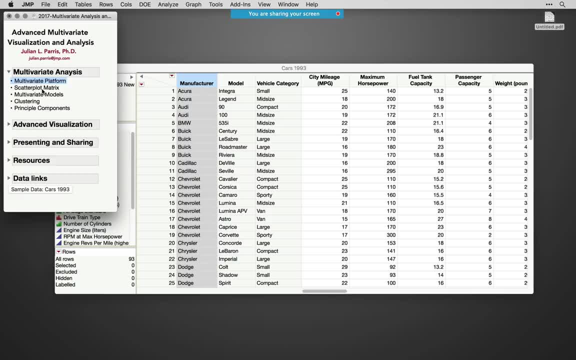 which has a very small passenger capacity and very large amount of horsepower. All right, so I'm going to just minimize this for now. We may use that in a dashboard. later Let's explore a scatterplot matrix version of this. So scatterplot matrix is a graphing tool. 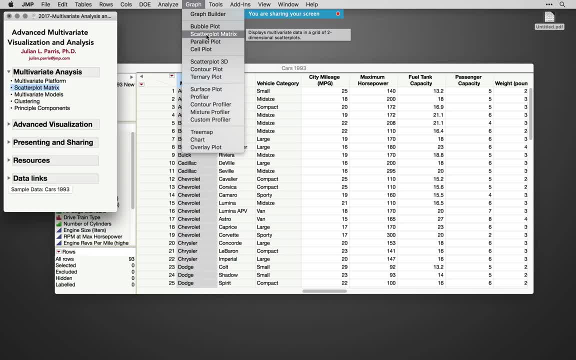 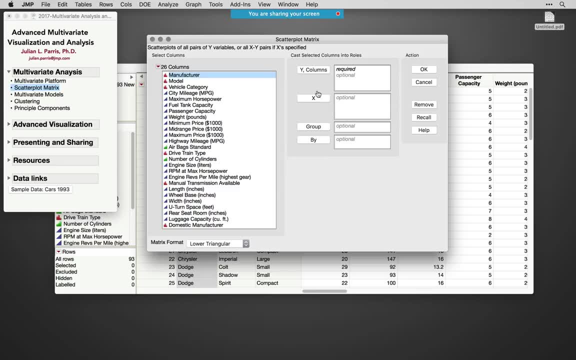 It's under the graph menu. It's not going to give us as many numeric options as the multivariate platform, but I want to show you how it can compare to what we just made in multivariate. I'll take the same variables. we used these first five. I'm going to click them into Y columns. 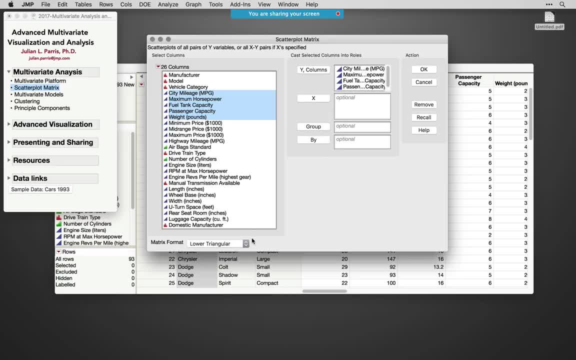 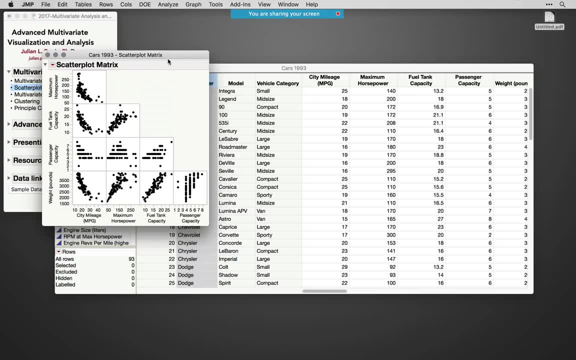 We'll come back and look at what X and group do, But notice that by default there's the lower triangle. So that's the matrix format that it's defaulted to When I click OK. I want you to see what this does And I'll bring back. 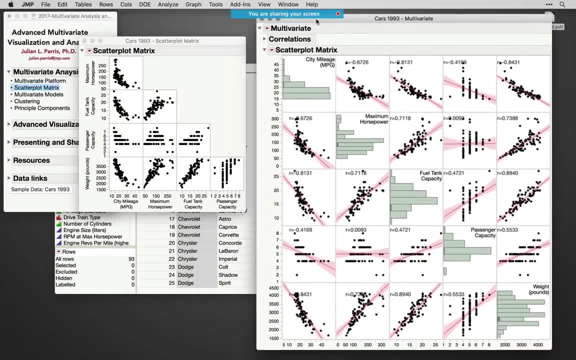 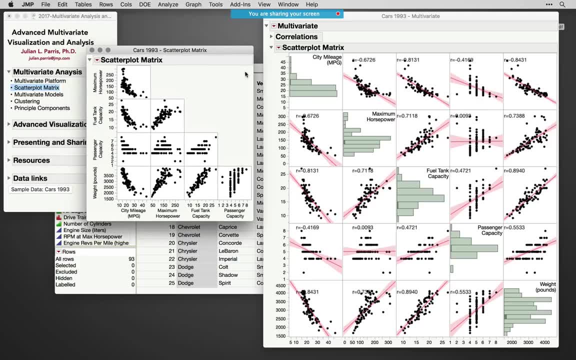 my multivariate output from the previous time we did this, And you'll notice there's a slight difference in how it's orienting the scatterplot matrix. Instead of having the entire square, we're eliminating the on diagonals and everything to the other side of that, And so we're basically. 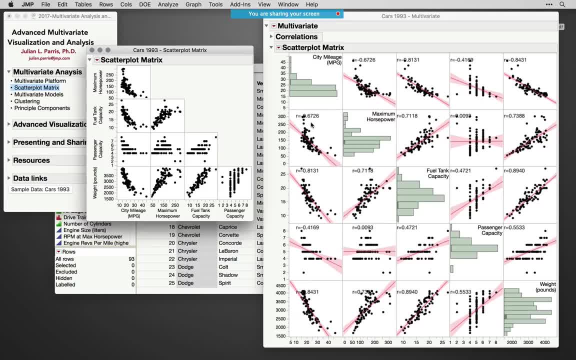 on the left-hand side looking at it, And we're going to take the same variables and we're going to just this lower section here. Now that ends up being just fine. The redundant cells for many people are just that: They're redundant, And so if what you care about is seeing just once those, 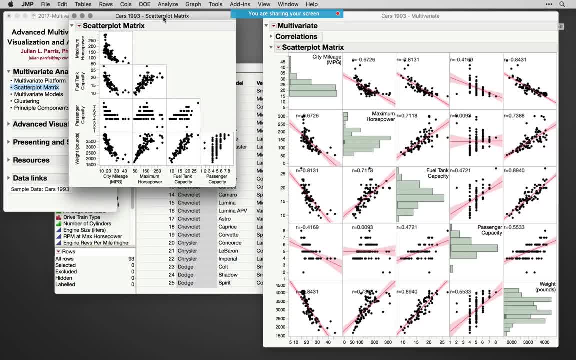 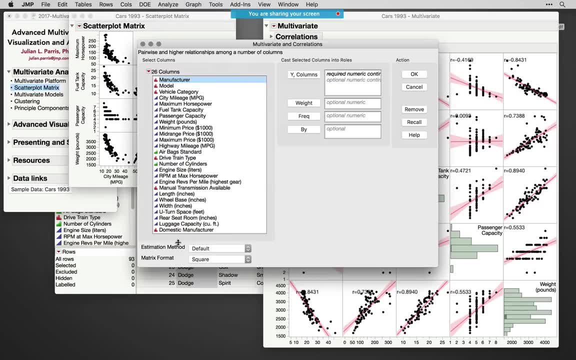 particular scatterplots. the scatterplot matrix gives you a nice way of doing that. It turns out that so does multivariate. If you remember when I invoked multivariate methods, multivariate at the very bottom- let me hit recall. That'll bring back the variables. 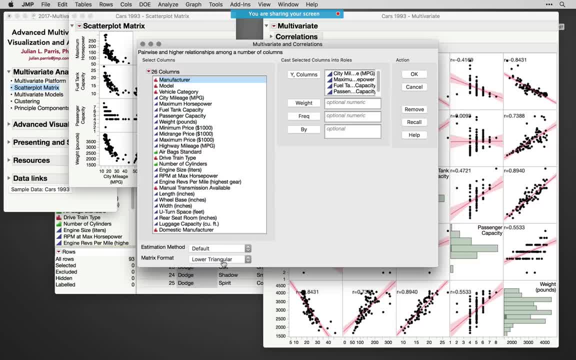 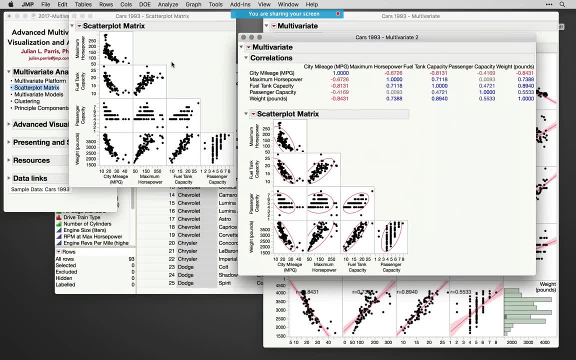 There is a matrix format here to use lower triangle as well. Obviously, upper triangle will do the opposite of that. I'll do lower triangle, just so you can see, And that ends up being really the same exact output. Now there is something important, though, And the reason I wanted. 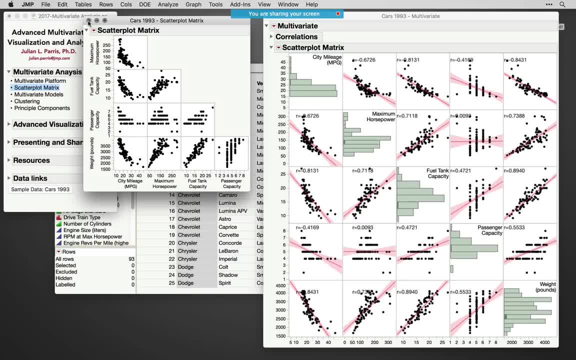 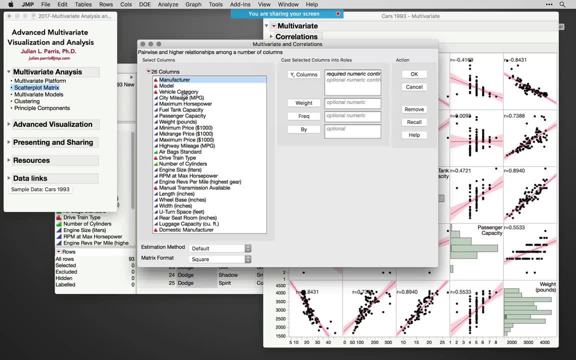 to show scatterplot matrix. there is a different thing you can do with scatterplot matrix than you can do with multivariate. If I go to multivariate and let's bring in those same variables we had before. let's imagine we wanted to bring in one additional variable. Is this a domestic manufacturer? 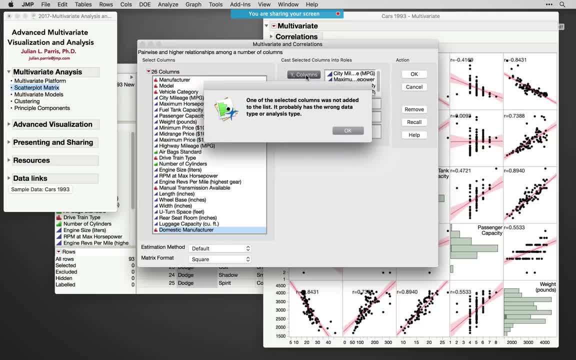 or is it not a domestic manufacturer? If I try to click that in multivariate doesn't quite like that. It says one of the variables in the list was not the right analysis type or wrong data type And that's because that is a. 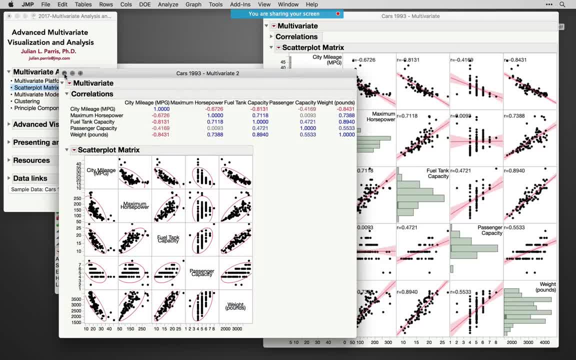 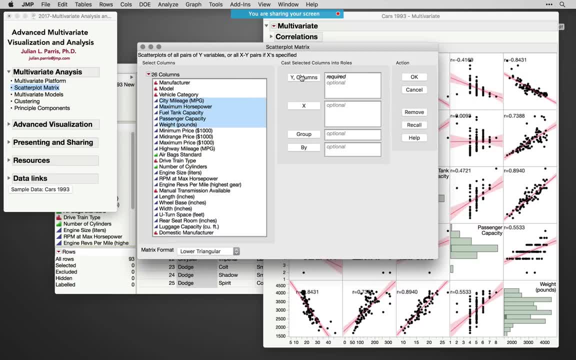 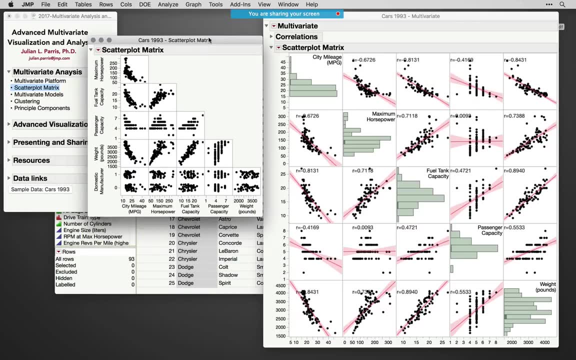 categorical variable right now Scatterplot matrix. on the other hand, under graph, scatterplot matrix actually will be okay with that. I can add in my variables. I'll take domestic manufacturer and also add that in. So notice it is in the Y column And the way it handles that is to make. 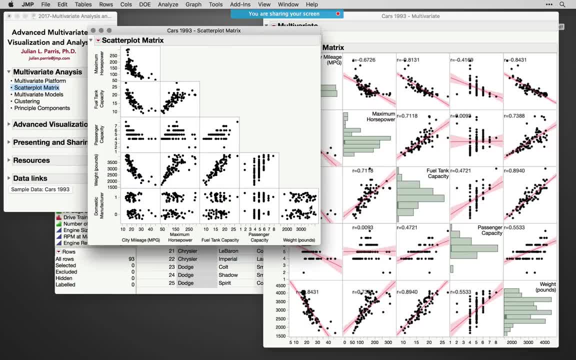 little variables. So I'll take domestic manufacturer and also add that in. So notice it is in the Y column And the way it handles that is to make little jittered dot plots And this actually works pretty well. You may notice, in this particular case there's not a huge difference for each of. 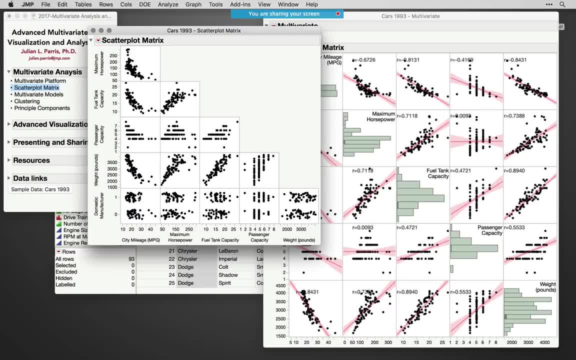 our variables between whether they're domestic or not, which you are noticing maybe in city mileage. There's a clump of them under domestic one who actually get much worse gas mileage, and a few that are not domestic that get quite good gas mileage. But this gives you a way of actually 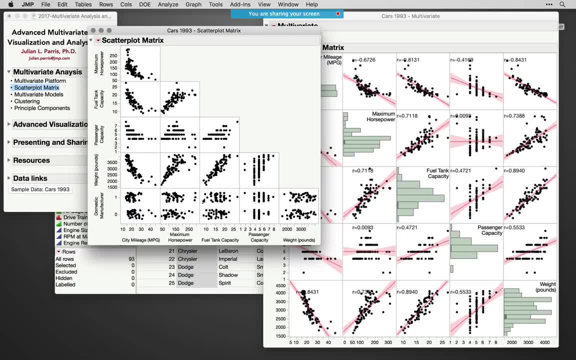 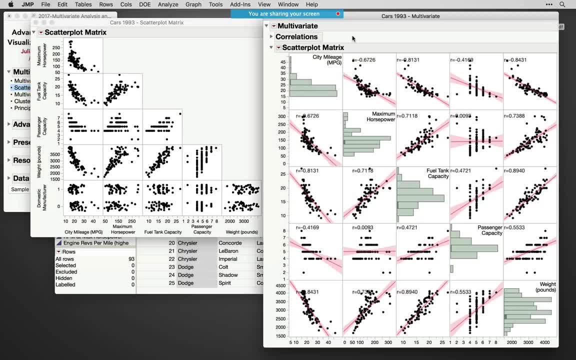 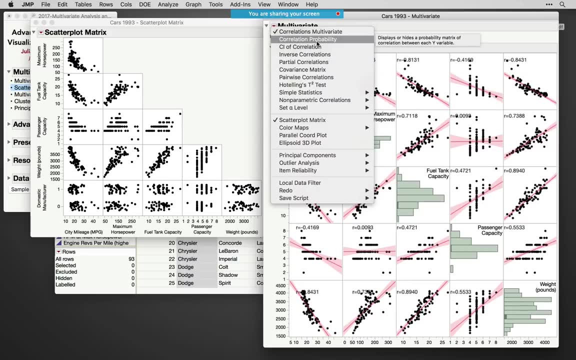 using and getting dot plots from variables that are not actually quantitative, And so scatterplot matrix has one little advantage there. The reason why multivariate disallows this is because multivariate methods requires the variables be numeric to do the rest of the numeric calculations. Notice, we got correlations. we can get confidence intervals on the correlations. 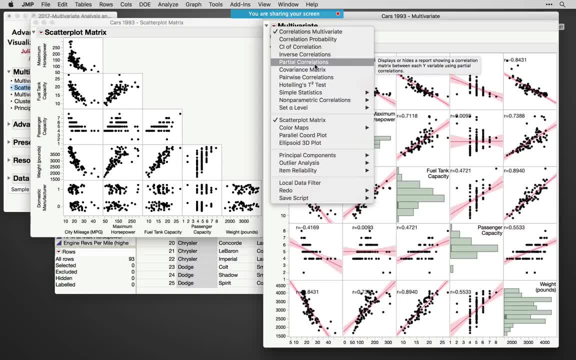 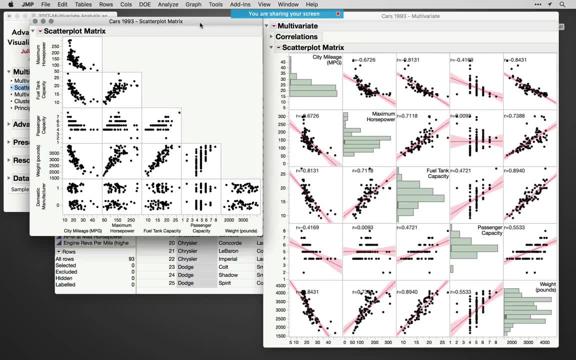 inverse correlations, partial correlations. all of these require that we have numeric data in order to perform those calculations. Since scatterplot matrix under the graph menu doesn't require that or doesn't perform those operations, it doesn't much care. So scatterplot matrix has 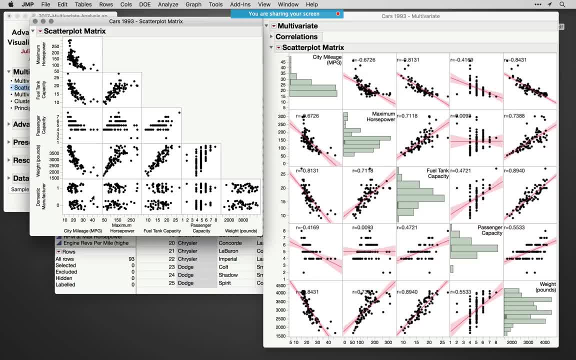 the option to compare if those entries or if those variables entered are fully numeric. There are a few additional options that you can get under scatterplot matrix. There's also the option for non-parametric densities. This is a pretty nice output. If I turn off the points, you'll see what it's done is. 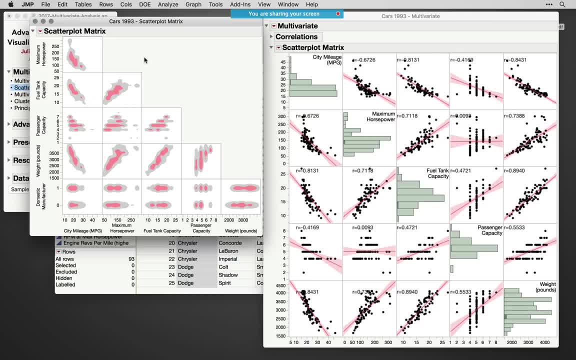 it creates little heat maps of where most of the observations are, And so this is a nice way, without imposing any sort of model, like lines are doing, but just seeing where the observations tend to fall. So be aware that scatterplot matrix is a nice way to see where the observations tend to fall. So be aware that scatterplot matrix is a 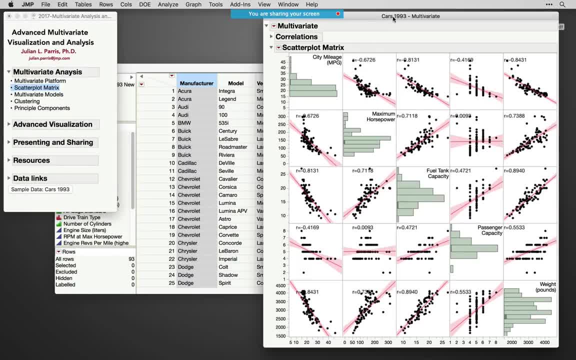 nice way to see where the observations tend to fall. So be aware that scatterplot matrix is a nice way to see where the observations tend to fall. So be aware that scatterplot matrix is an option and something that you can use in your your arsenal when you're creating visualizations. 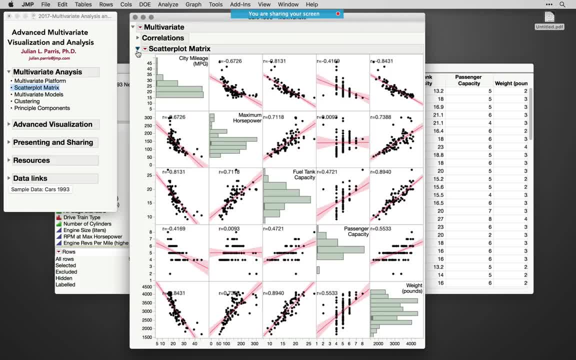 Alright, while we're still in multivariate, I want to point out a few other things you might find useful. Alright, while we're still in multivariate, I want to point out a few other things you might find useful. I'll minimize the scatterplot matrix and let's go back to the 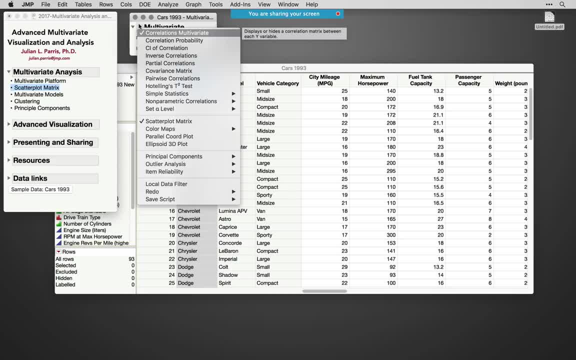 Top Red Triangle. When you have a large number of variables, your scatterplot matrices tend to be a little overwhelming. You have so many of those little sections with scatterplots that they don't become very useful to assess what variables relate to which other variables. What ends up being very useful. 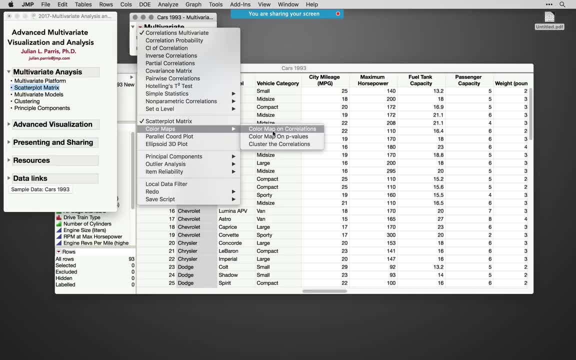 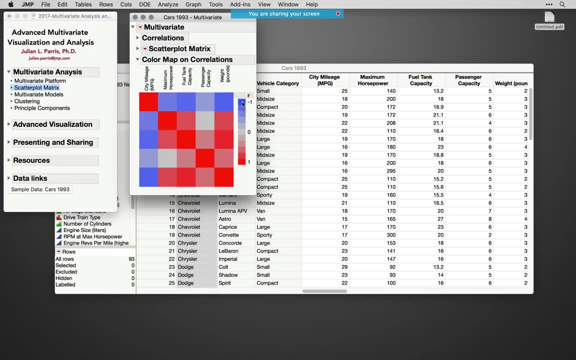 are the color maps, and so if I select color map on correlation, what we get is a color map where positive correlations are red, very negative correlations are blue, centered is zero. this is actually picking up on my default color gradient under the preferences menu and jump. I can actually set what my default color. 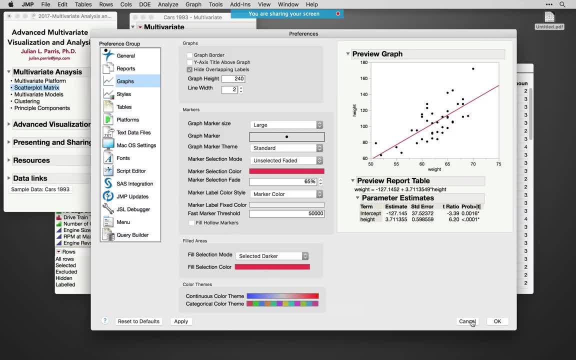 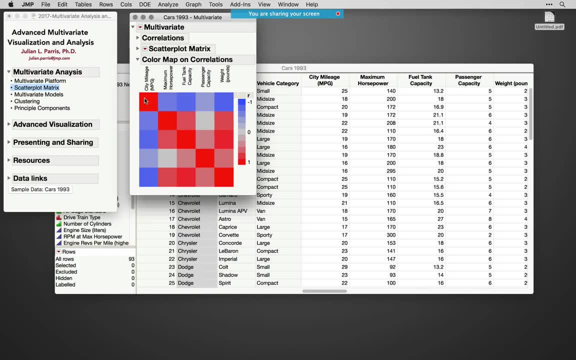 gradient is, and so that's my continuous color theme and so you can change that if you like, but this ends up working pretty well. the on diagonals all have a positive correlation of one. a variable with itself is positively correlated at one and you can see where the off diagonals are, so at a at a glance you. 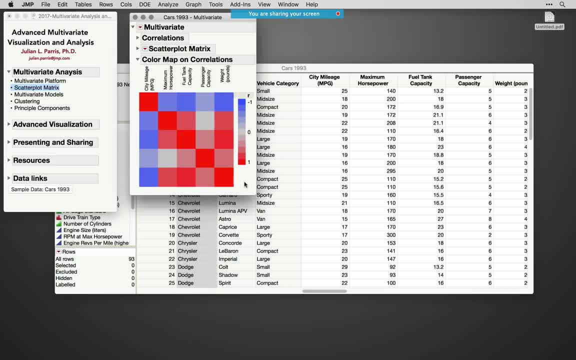 can see very quickly where are the places where there are very large positive or very large negative correlations. so we can see that city mileage is very negatively correlated with weight in pounds and so that kind of makes sense. very heavy cars probably aren't going to get very good mileage. 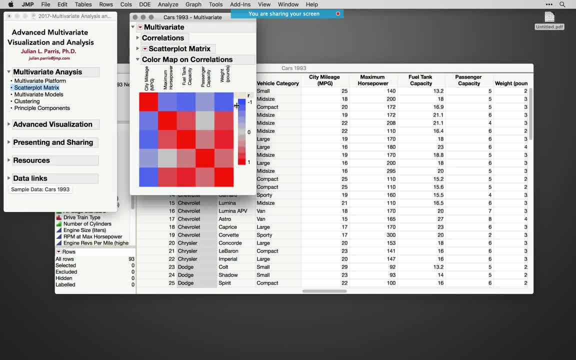 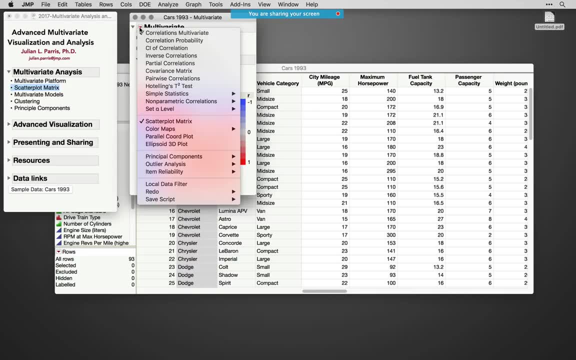 maybe that's because they're related to horsepower, but that's something we'll be able to figure out in the future, investigate with a proper multiple variable analysis in just a minute. so the color map on correlations is an excellent option to use. you can also color map on the p-values and cluster on the correlations cluster on. 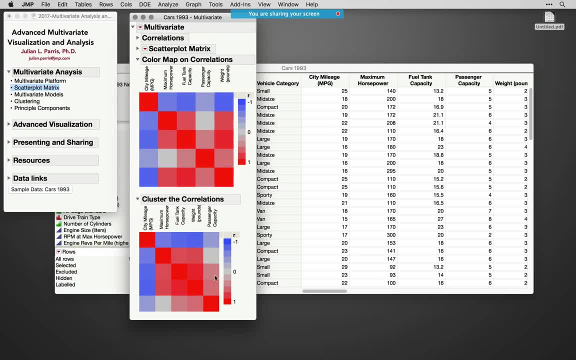 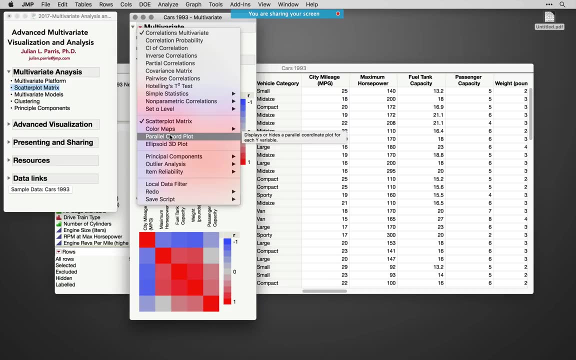 correlations gives us a slightly different variant of this where it's basically stuck all the correlations that tend to be close into the same place. that's reordering the the rows here. so, additional options that I like, parallel coordinate plots- we're going to come back to in just a minute. know that you can get to them from multivariate. I'll. 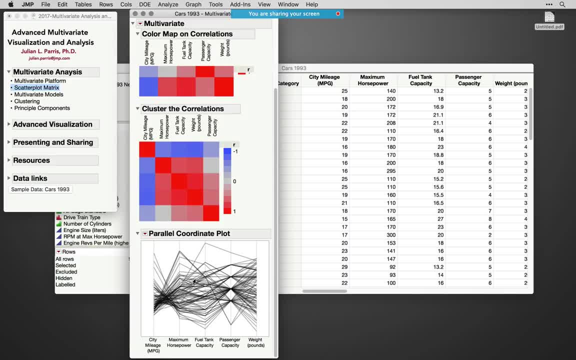 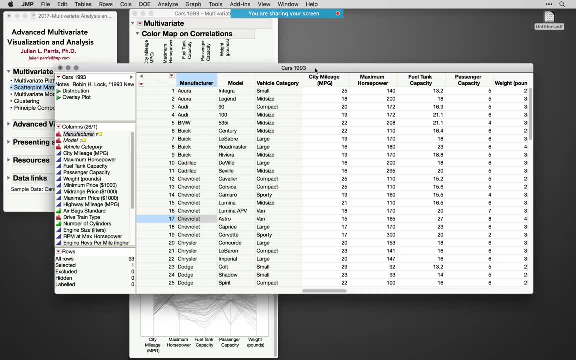 just produce one here. if you've never seen a parallel coordinate plot before, don't worry. we'll step through it in much more detail later. but just to give you a sense I'll click on one of these lines. that line will notice it is selected in the data set: the Chevy Astro van. what a parallel coordinate plot is. 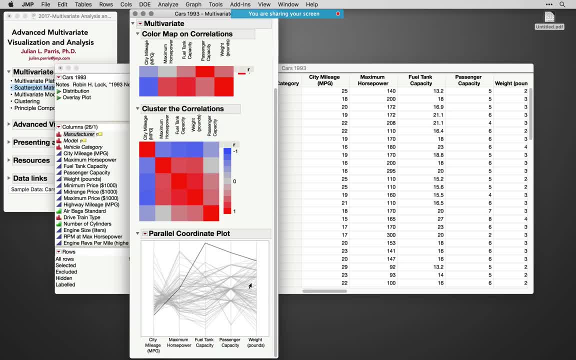 showing is the profile for these five variables of a Chevy Astro van. it tends to have low city mileage relative to the rest of the cars. it has a medium horse power, a large fuel tank, medium-high, actually very large, the largest passenger capacity and almost the highest weight. so what we're looking at 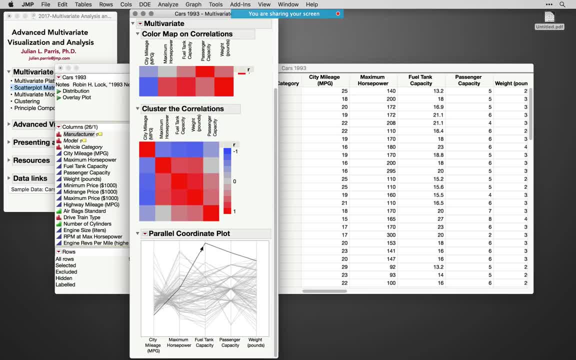 is in, in a kind of a standardized coordinate space, the profile of that car. and any car we pick will have a profile and so if we find the one with the best city mileage, there is right. the one with the best city mileage tends to have the lowest horsepower and fuel tank. which car is? 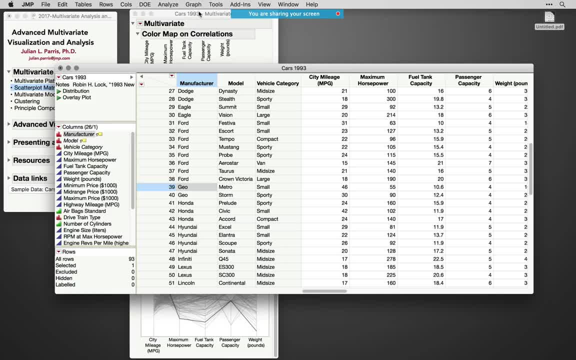 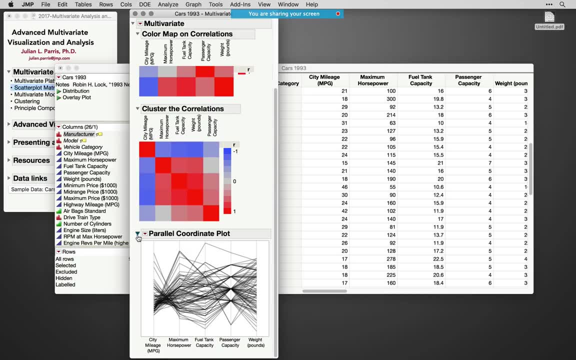 that this was the GeoMetro 1993. if you all remember, the Geo Metro was a car, So the parallel coordinate plot is another high dimensional visual. We're gonna see a different way of making it in just a minute, but this is a very nice thing you can get to. 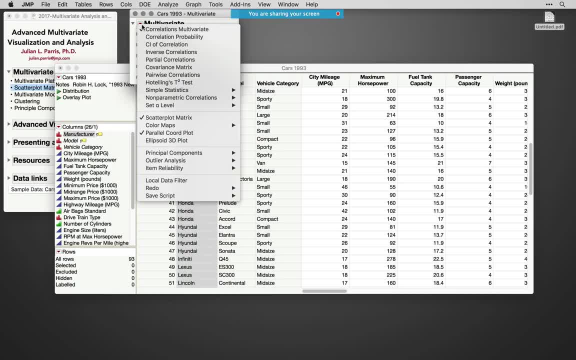 directly from the multivariate platform. Finally, there are some additional methods we're not gonna cover here, but some of my favorites live under the outlier analysis section. If you're performing analyses that require or use a lot of variables in the X space. 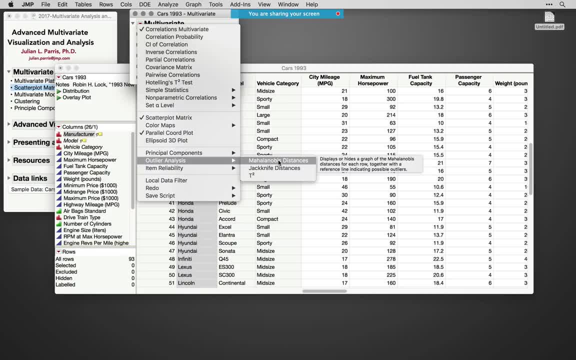 looking at whether there are outliers in that X space is really important. So I'm Halanova's. distance measures are really great for that. You can also launch directly into principal components, item reliability, or even get 3D plots here. An ellipsoid 3D lets you select three of your variables. 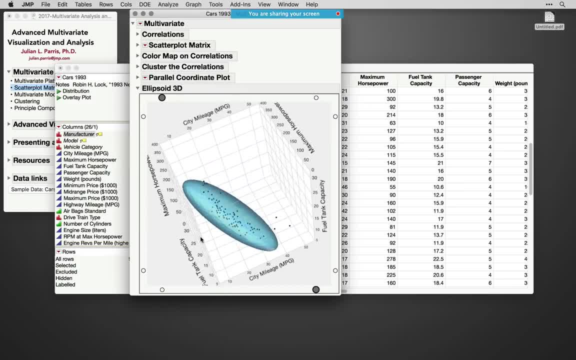 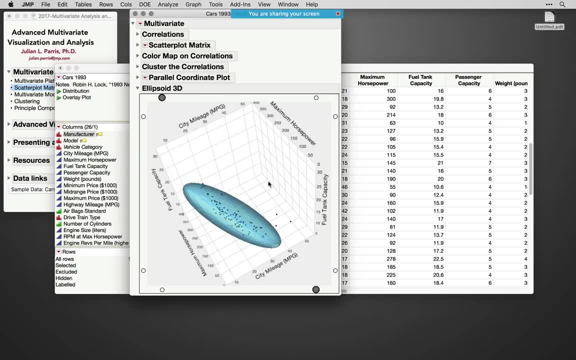 and allows you to look at that variable, those variables rather in three dimensions. And then the ellipsoid is sort of a generalization, or is a generalization of that ellipse we saw in the correlation scatterplot matrix. This is showing in three dimensions the ellipsoid. now 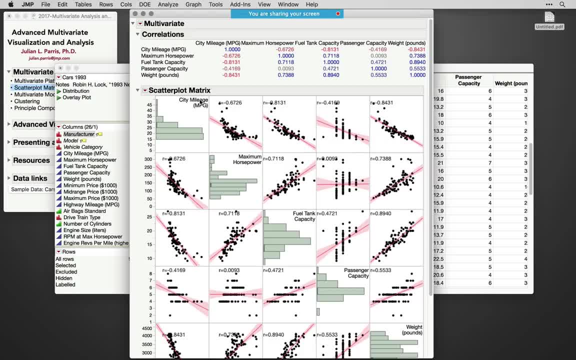 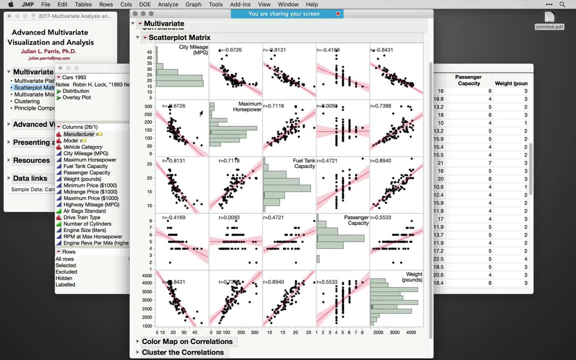 So that's multivariate: A lot of options and even beyond just the basic ones, a lot of ways that give you nice ideas of thinking through what variables are really relating to each other in your dataset. And so, before we start fitting any models, 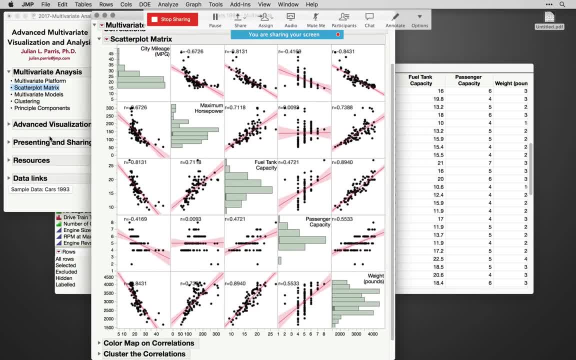 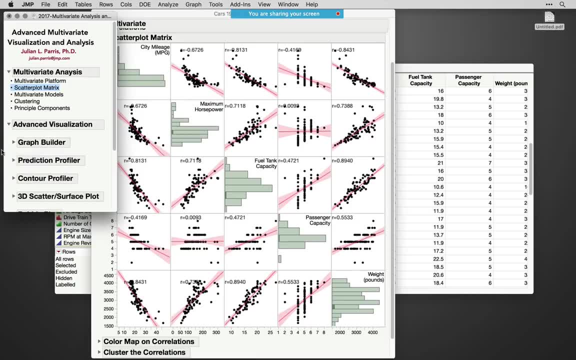 let's think about how we might display some of the relationships we've seen, but using other graphing platforms and maybe invoking things you haven't seen before in jump. And so I'm gonna start with graph builder, probably my favorite graphing platform. 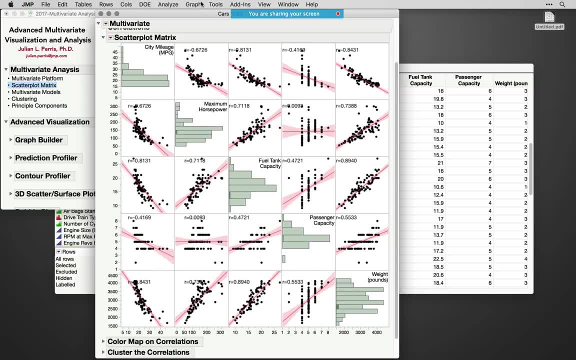 And one, it's simple, gives you the ability to construct some very advanced graphics that tell a great story about relationships you see in your data, And so graph builder is available under the graph menu. I'll invoke graph builder here, And I'm gonna keep the multivariate platform open. 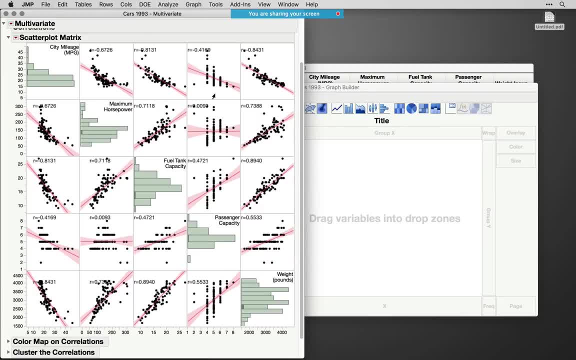 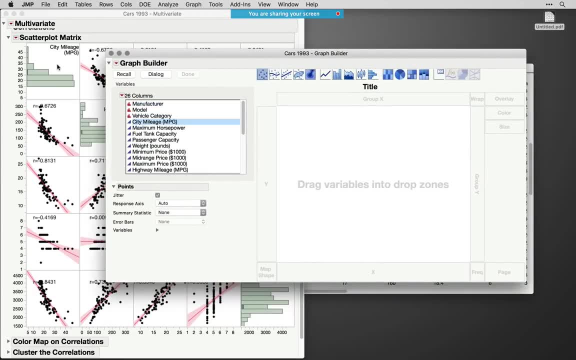 because let's investigate or look at some of these relationships, but maybe let's see how they relate to each other, And so I'll start by looking at city mileage. That was the first variable that I mentioned, or I even put in, And so maybe one we're interested in understanding. 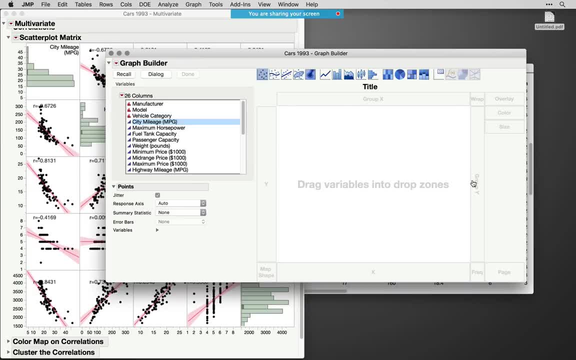 Now, the way graph builder works- if you've never seen it before- is it's built around drop zones, And there are drop zones for data like Y and X, and drop zones that group your data or group your visual group, X, group Y and wrap. 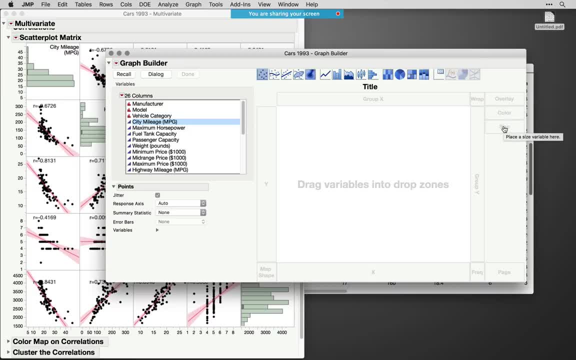 Then there are drop zones that modify the points, like coloring and sizing, or put multiple visuals on top of each other, which is what overlay will do, based on the levels of a particular variable. This is all made more clear once you see it happen. 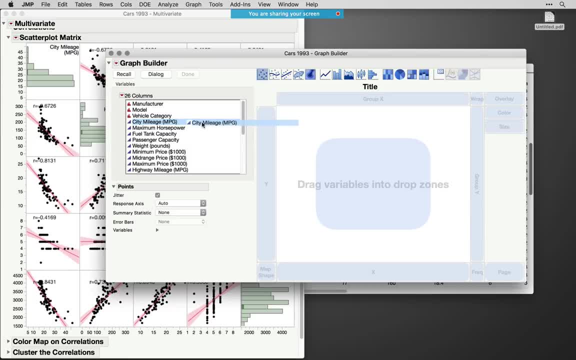 I'll take city mileage. the drop zones where I could drop that are highlighted If I hover over Y jump will add it to the Y axis. One brilliant thing about graph builder is I don't have to drop a variable. I can simply move it to different spaces. 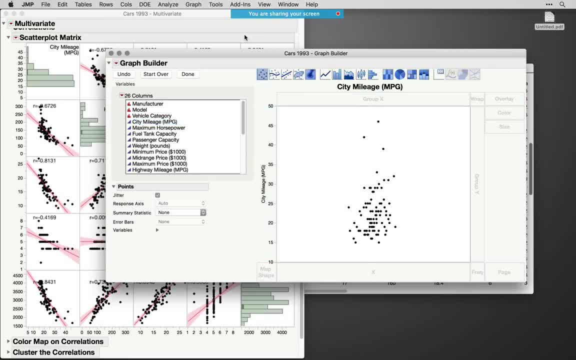 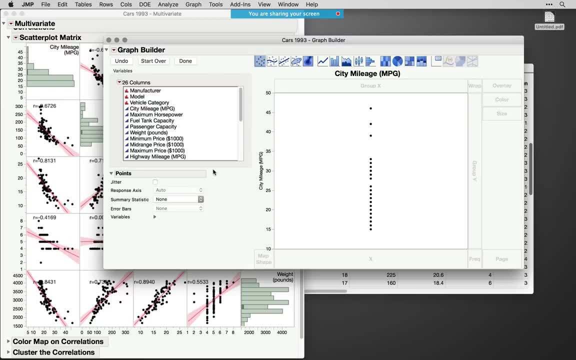 and see the effect it has on the visual, And so I'm actually gonna drop it in the Y drop zone. So I'm gonna treat this as my outcome. variable Jump is jittering the points. by default I can uncheck jitter. The control panel here gives me controls. 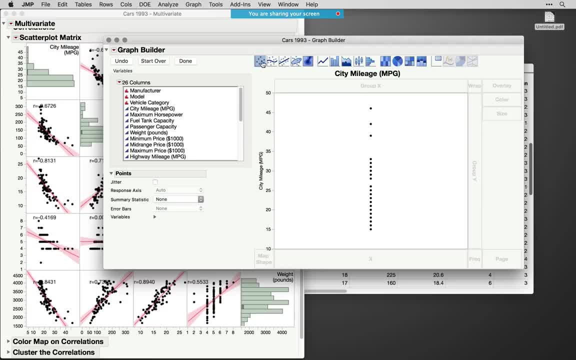 over the elements that are in the visual. The only element here right now is the points I can toggle between different elements like a box, plot, bar, chart, contour, plots, right. These are all elements that can display data in one dimension. 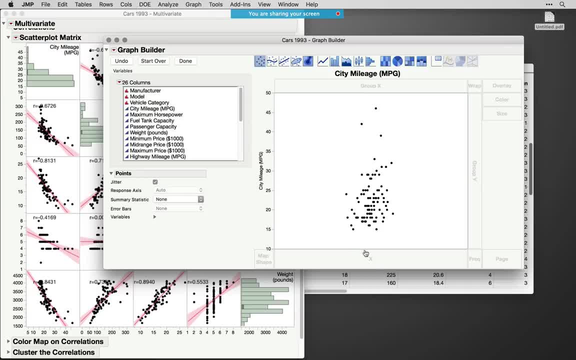 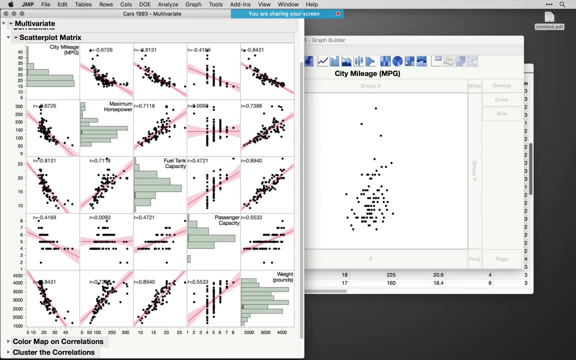 So I've left jitter on. I have left the points on. Let's now define an X axis. Let's consider horsepower. We know that- something based on the scatter plot over here- there's a negative relationship between horsepower and city mileage. but let's see if we can clarify how that happens. 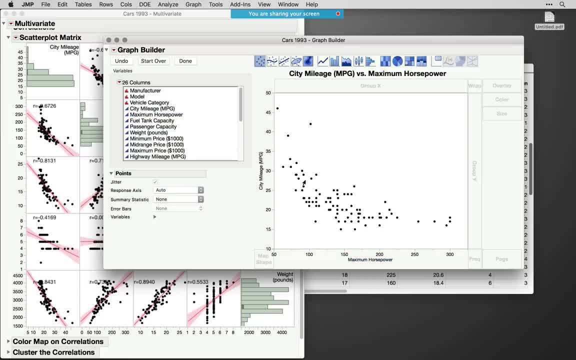 And so I'm gonna drag horsepower down to the X axis. Again. jump creates a visual as I drop. I drop the variable or even hover the variable over that axis role. We have a number of things we could put on this visual So I could put on a smoother 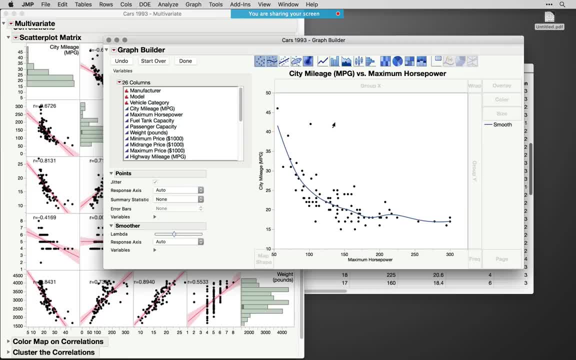 This is actually the default If you were to drop those variables in at the same time. the smoother is sort of like a moving average As you move lambda up the stiffness of the line. rather, you get towards the linear regression of Y onto X. 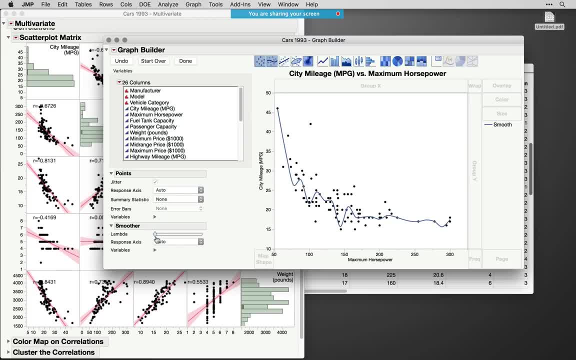 As you move to the left, you're allowing the line to be more smooth, to pick up more irregularities relative to a linear fit. There's sort of a point where you're probably fitting noise and a point where you're probably imposing too much linearity. 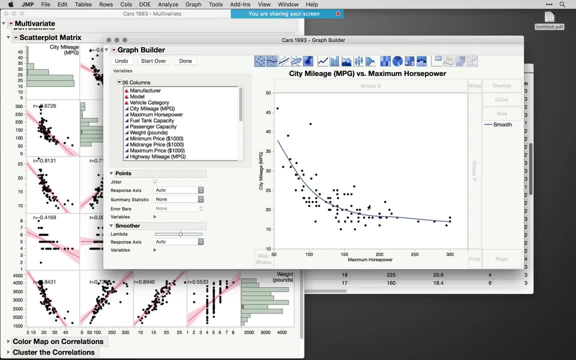 So the smoother gives you an ability to sort of play around with how the data are fit. So I'll leave the smoother on. We could have had a linear fit if we liked, or we could have connected the points, if there was some reason for that, based on the row order. 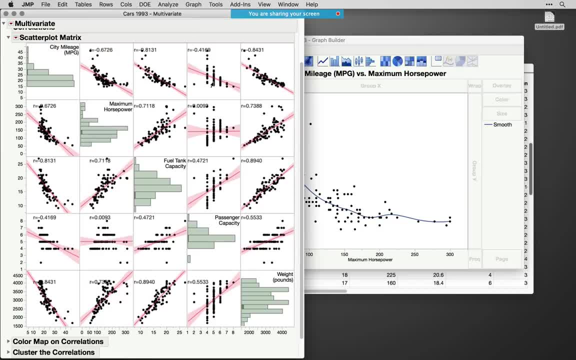 but I'll put back on the points with the smoother, All right, remember, we noticed that the weight of a car was related to city mileage as well, And when I actually use the scatter plot, I can see that the weight of the car was related to city mileage as well. And when I actually use the scatter plot, 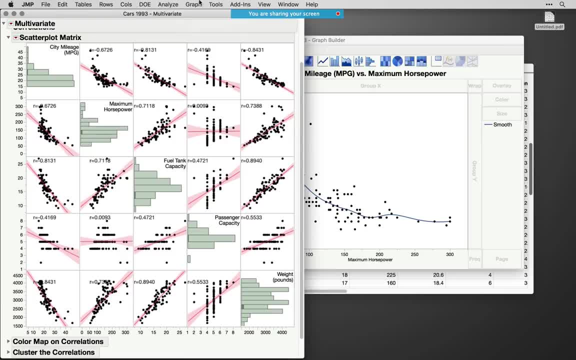 I can see that the weight of the car was related to city mileage as well, And when I actually use the scatter plot in matrix, we even looked at things like whether our car is domestic or not and whether we didn't look at it yet. 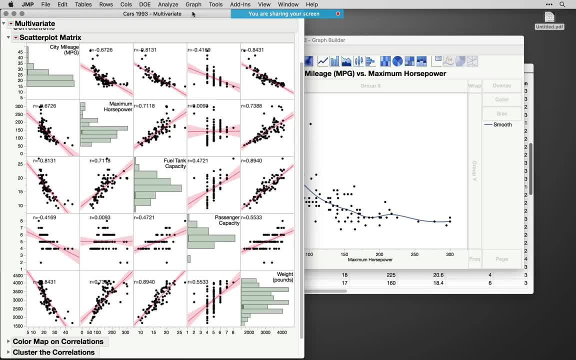 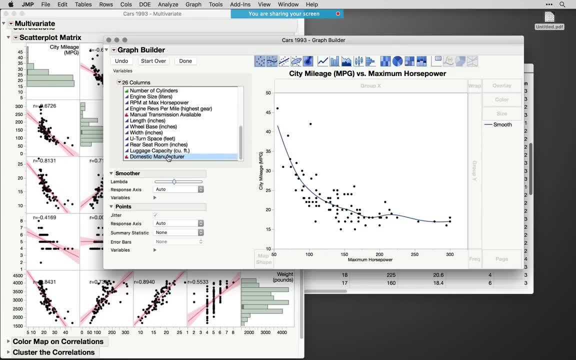 but whether a car is a small, medium, sporty, how it's classified, And so we can invoke those other variables in a number of different ways, And so domestic manufacturer is a simple one to start with. You know what, if we wanted to look at the relationship here, 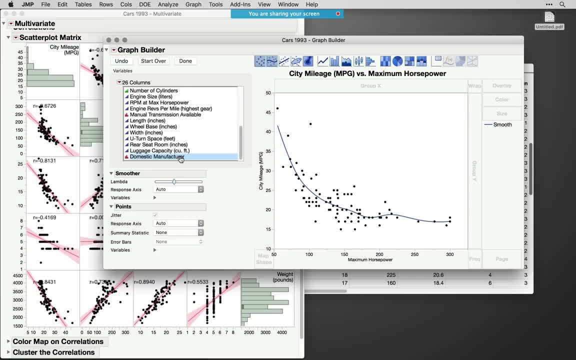 city mileage and horsepower, but across domestic and foreign cars. And so if I drag domestic and foreign to this group for X section, notice what jump does. It's now split up the X axis where on the left hand side we have just for the domestic cars. 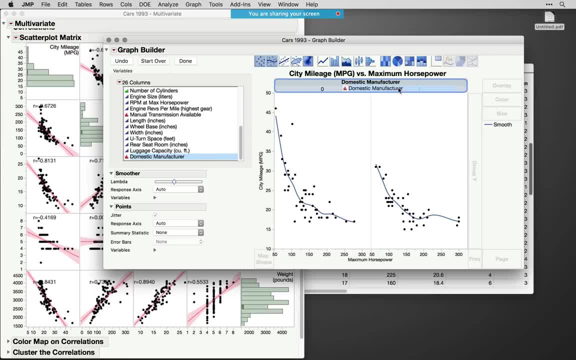 or sorry, non-domestic cars, And on the right hand side the domestic cars Group for Y does a similar operation: breaks up the Y axis. Wrapping seems to do the same thing as group for X. Notice I can move between the two of them. 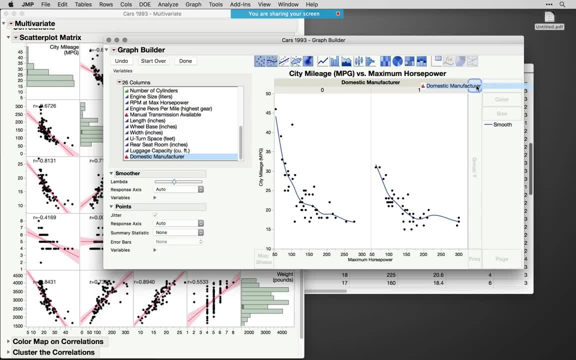 The reason why that's not differing is because I only have two levels here. You'll see, when we work with a variable that has more than two, perhaps I use number of cylinders, And so if I do number of cylinders, notice that breaks it up as a trellis plot. 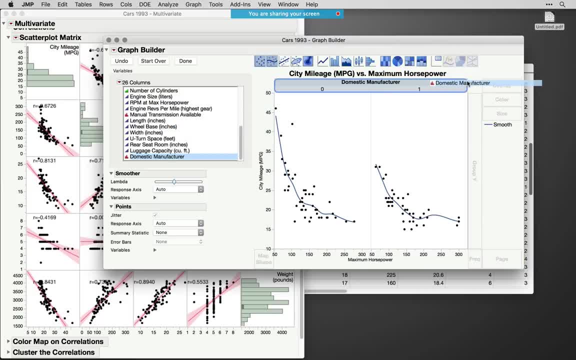 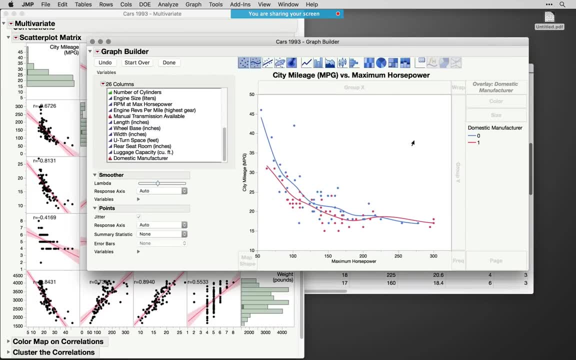 I'll go back to domestic manufacturer, So group for X and wrap with two variables or two levels of a variable. excuse me, we'll do the same. And then finally, overlay does, something I quite like too, And so overlay will take instead of having the axis split. 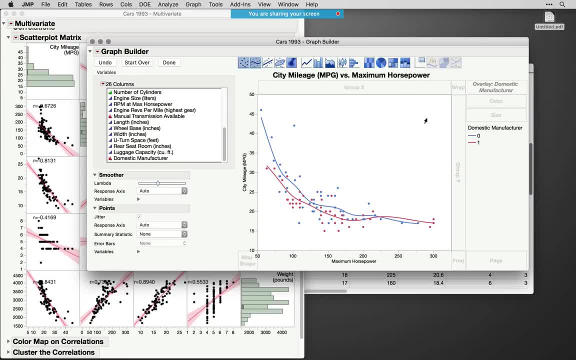 across the levels of domestic manufacturer. it takes whatever visual we've defined, in this case the smoother, and displays it separately for the levels of that variable. And so we have the domestic manufacturer zero and domestic manufacturer one as separate points and separate lines. 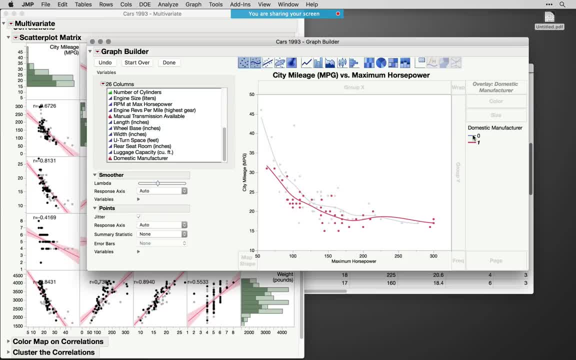 And not only are the points colored, but the lines here are different colors as well, And you'll notice something. there's sort of a mean shift here. So the non-domestic cars are just getting higher mileage overall, even for the same horsepower. 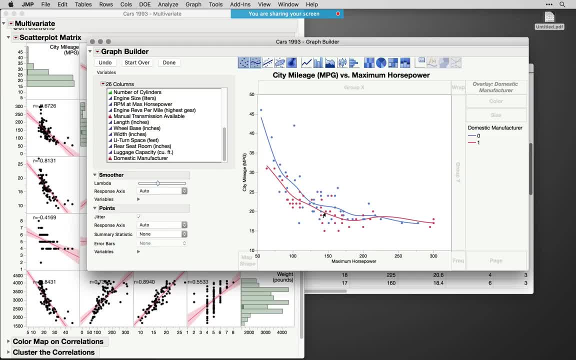 And so even for a car at 150 horsepower, we're actually getting better mileage. if we happen to have a foreign car, You may have noticed, it's maybe a little hard without any grid lines. Let me make some modifications to this graph because maybe we want to make this easier. 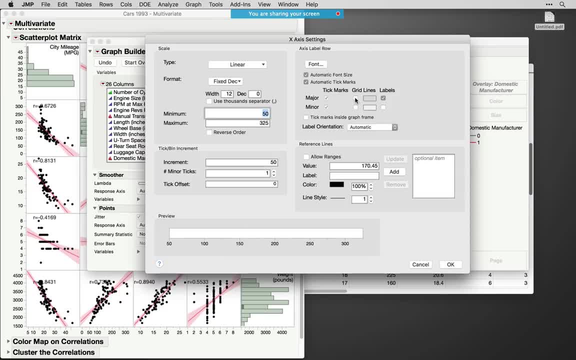 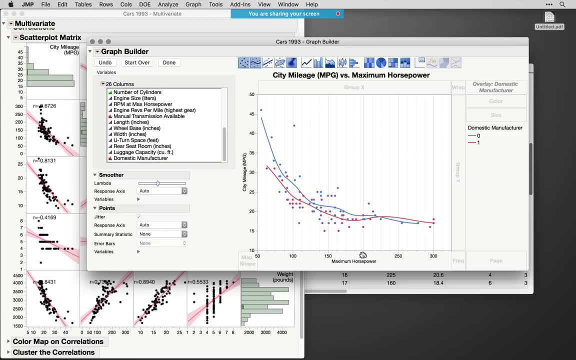 for our visual users, And so I just double clicked the axis and I can turn on grid lines. I'm gonna turn on grid lines with three minor ticks. I just happen to like three. So there's our graph with three minor ticks for horsepower. 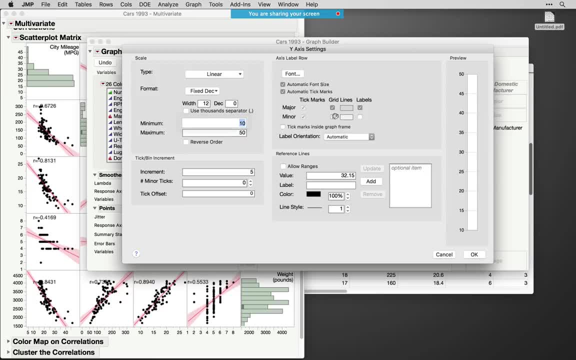 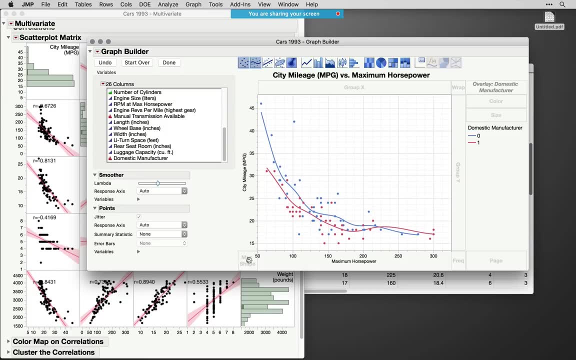 I'll do the same thing for mileage. Let me double click the axis, turn on grid lines and turn on three minor ticks, And so now we have. it looks a little bit like graph paper, which I always loved, And so now we have a graph where we can look at. 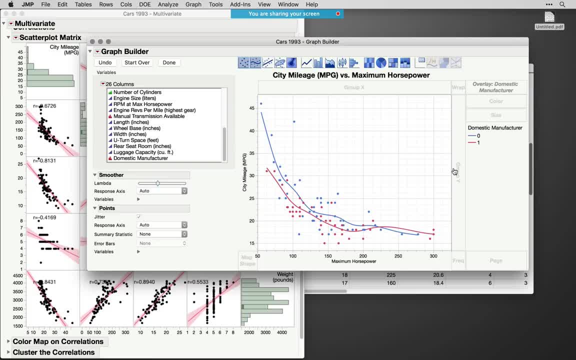 you know a particular mileage here or a particular horsepower. So notice, by using overlay we were able to break apart that visual and really see how those differences really fleshed out. I'm gonna take out domestic manufacturer and let's try a different way. 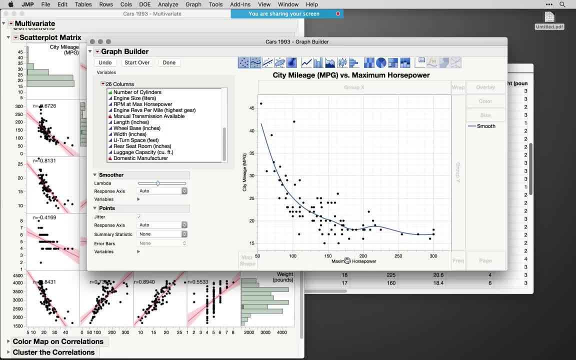 of involving another variable. I suppose we wanted to look at the horsepower differences, let's say by the type of car. So vehicle category. Vehicle category is small, compact, van sporty, midsize or large. So I could use this in an overlay role. 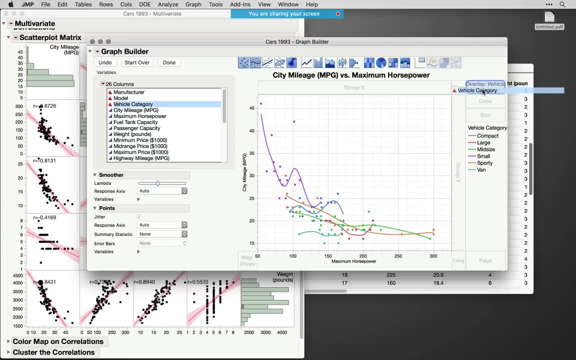 It's gonna be pretty messy And notice. what it's doing is showing the differences in the relationship. But what if I only want to show differences in horsepower among these different classes? Well, if I don't wanna involve mileage, I can use one of the drop zones above or below mileage. 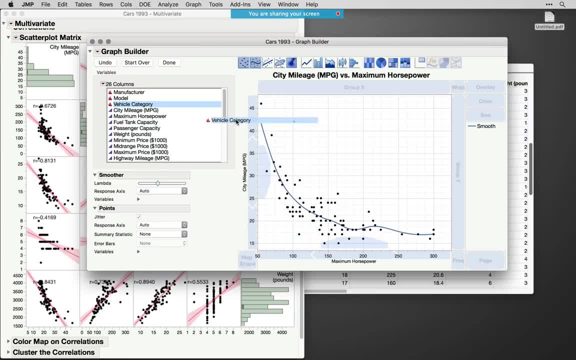 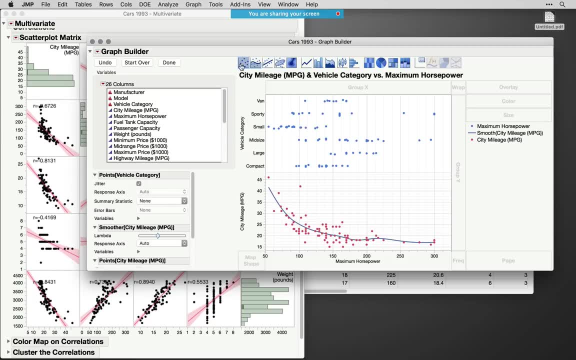 This is a way of doing a separate plot, adding into the current plot, And so I'm gonna drop it right above mileage. Now jump starts off by using the same element. That is the point that I had used before. Jump is smart enough to know that a smoother 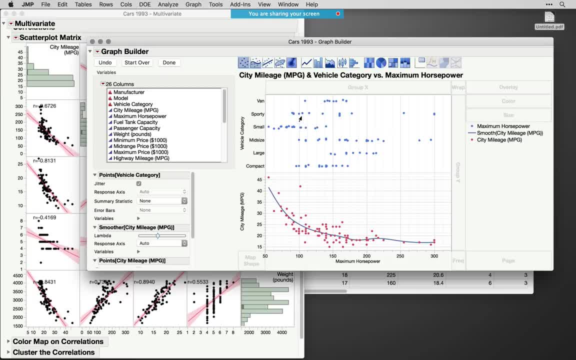 doesn't really make sense for categorical. We're not trying to connect the lines between these two. But maybe I want something different than the points. Maybe I wanna turn on the box plots or a bar chart, An easy way to do this and the way I typically do. 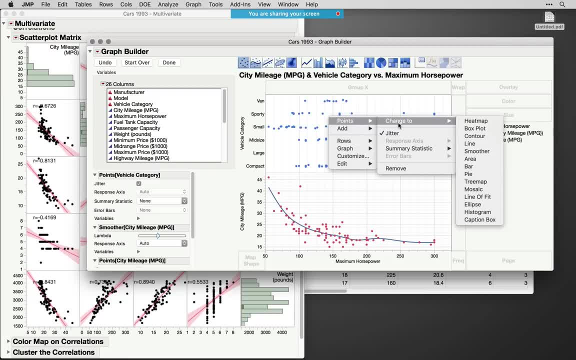 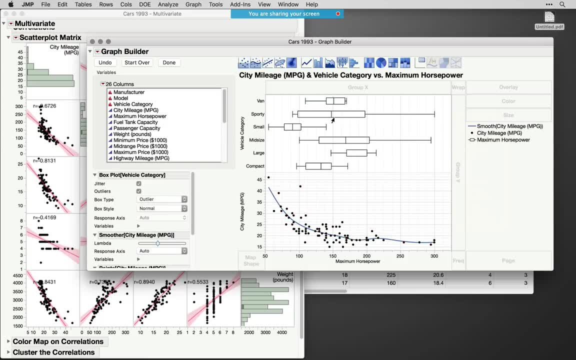 is I right click, hover over the point section And I say change that element. And then I'm gonna drag and drop it into this sub graph, into let's do a- actually let's do a- box plot. That's a great way of looking at these. 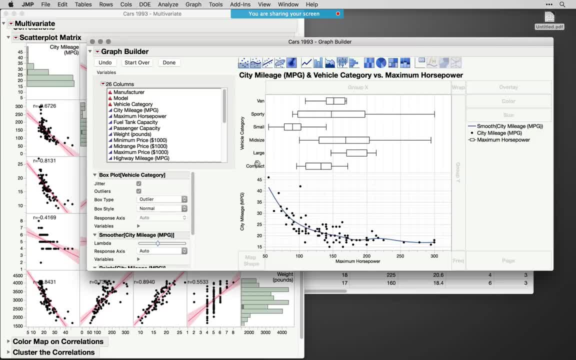 And so we have a box plots now looking at just the differences among horsepower for the different vehicle categories. So we're looking at the medians, the quartiles and the fences. Now we can make lots of customizations. I can right click on the box plot in the legend. 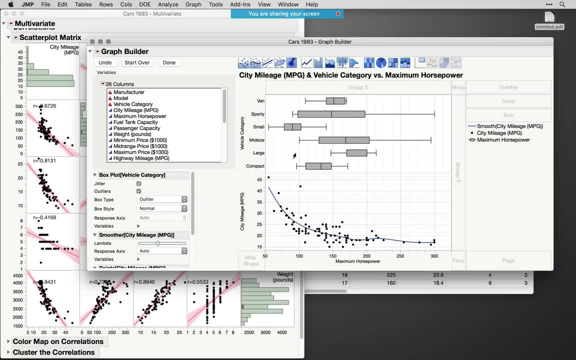 Maybe I wanna fill it with a color. I quite like box plots that have a little fill. We can resize Right here. if I hover right below compact notice, I can grab just that section, And so I can make this a little bit smaller. 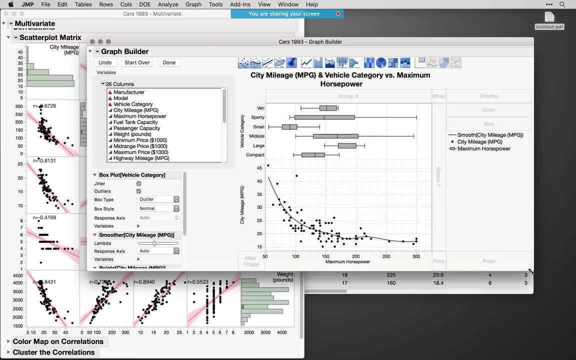 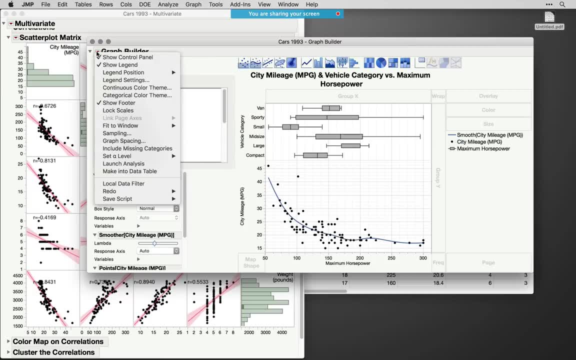 And so I'll do it like this, Right. so now we have a visual that maybe tells a bit more of a story, And I can change all the axes just by dragging. If I don't want the legend, I can go to the red triangle. 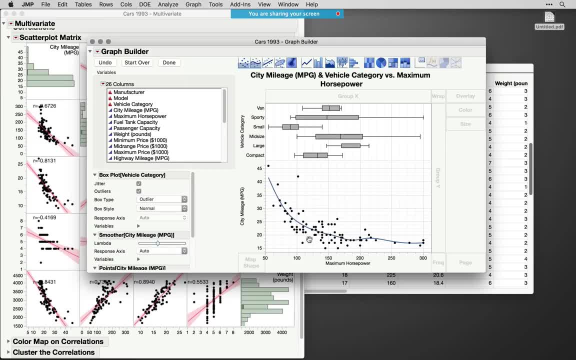 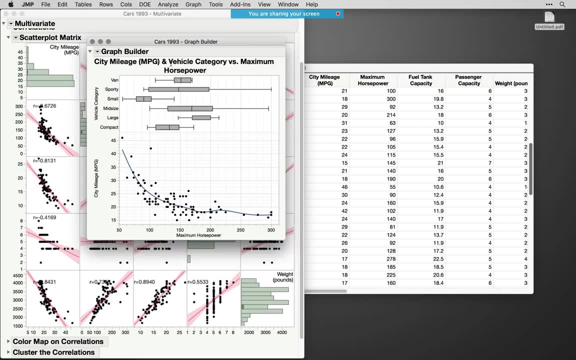 turn off that legend Probably isn't adding too much additional, since we already know which each of the variables are and which sections they're in, And notice when I don't need all the controls anymore, I can click done and it closes all the controls. 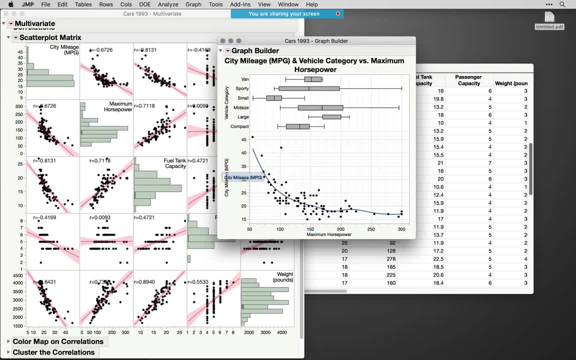 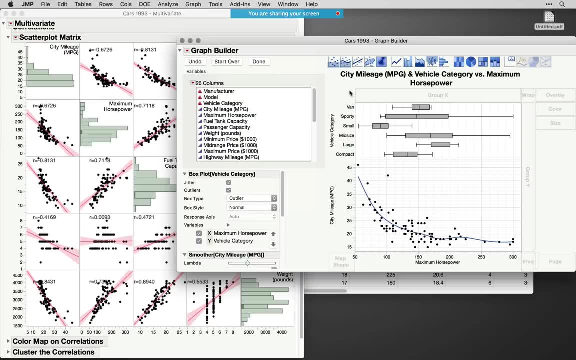 You can still make changes to things like the titles, the axes. those are all still editable. But if you need to change which variables are used, go back to your red triangle and turn back on your control panel And that'll give you your graph builder controls back. 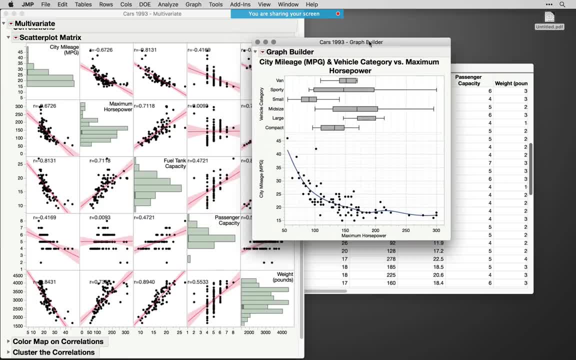 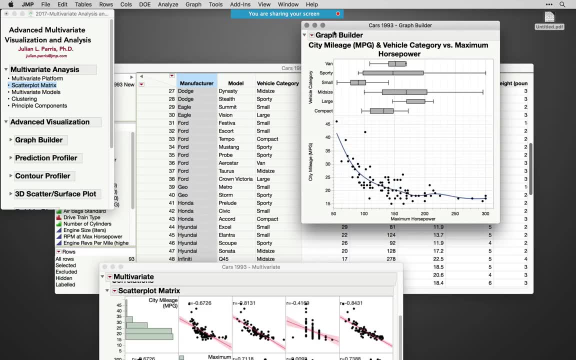 But I'll click done and leave this. This is a graph maybe I want to save for later. Speaking of saving, maybe this is a graph you'll want to remake multiple times And if you add more data, that took me a number of steps. 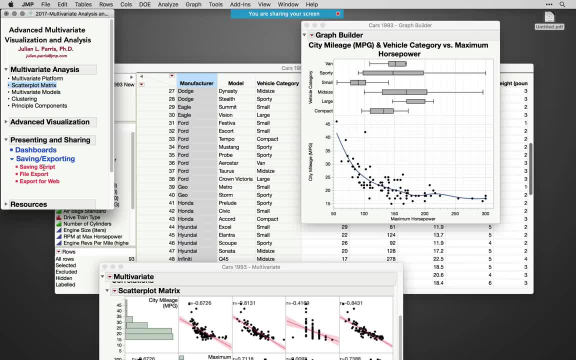 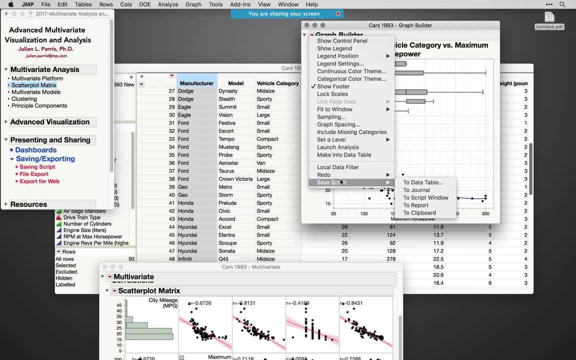 So maybe I want to save it in a way that lets me recreate it, And so I want to touch briefly on saving to a script. Under your red triangle, for any graph or any analysis, there's a save script section, And so, since this is one maybe I'm going to make again, 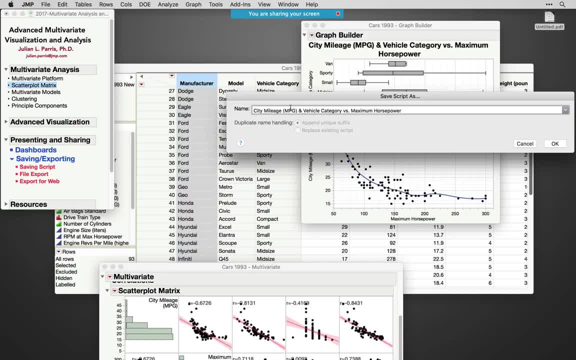 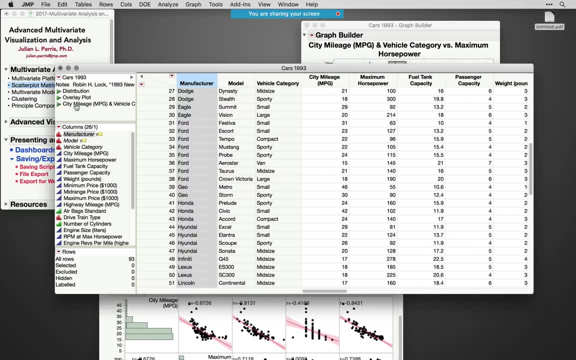 I'm going to select saved to data table And I'll give this a reasonable title. That's actually fine. It just picked it up from the title of my graph. I'll hit OK And notice that in my data table now there's this little script: saved over here. 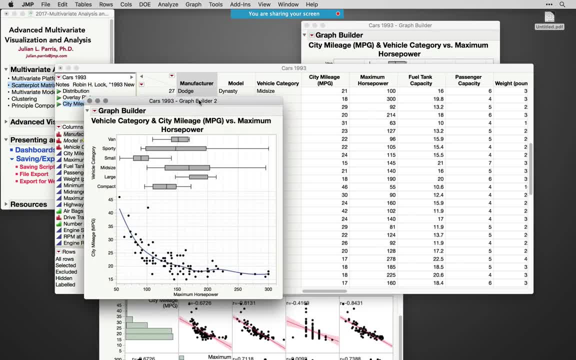 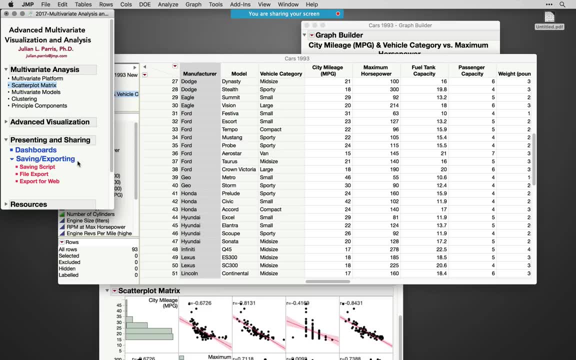 I can click this play button and Jumbo will recreate that graph using whatever new data I have, And so saving a script is a really valuable way of saving your analyses, not just for recreating But when you're presenting. I highly encourage you, whether it's in your classes. 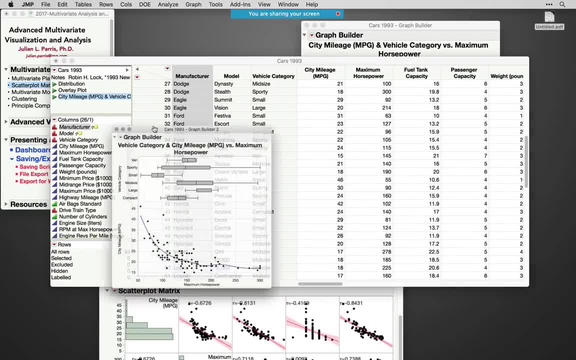 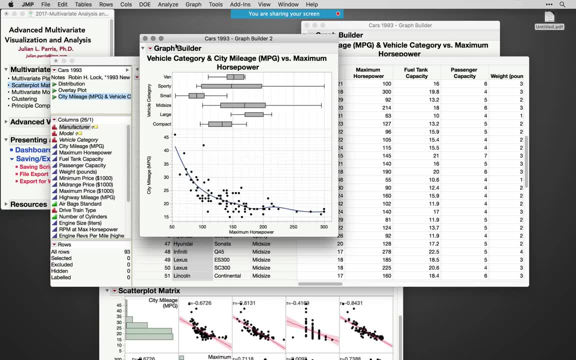 or during research presentations, have your data set open and work with the live data. There's nothing more impressive than actually being able to select points, to create graphs, to make modifications in real time, And Jumbo gives you a great ability to do that. 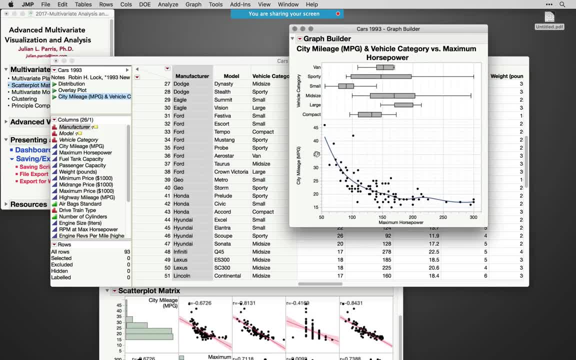 But saving your scripts. It means you don't have to subject your audience to the two or three minutes it took to set up this graph. So remember, under the red triangles, save script. All right, so that's a nice graph. I'll minimize that. 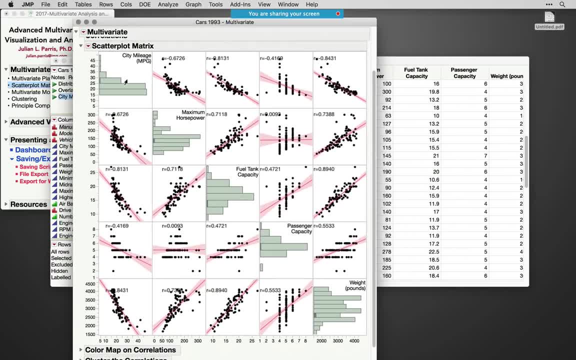 I want to show you a useful trick in Graph Builder if you wanted to create something like this. Notice: this graph really is just adding multiple variables to each axis and then using the same variables on each axis over and over. Just to prove that point to you, let's go back to Graph Builder. 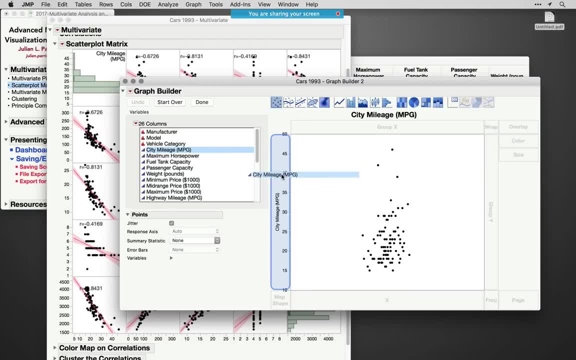 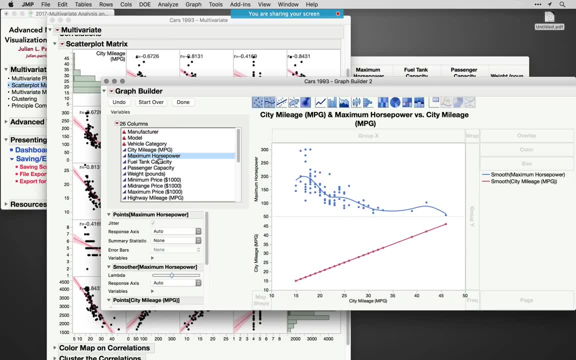 Let's do it for just two of these. Let's do it for just two of the levels. If I wanted city mileage on the Y and then I wanted maximum horsepower on the Y and then I put city mileage on the X and maximum horsepower to the right on the X. 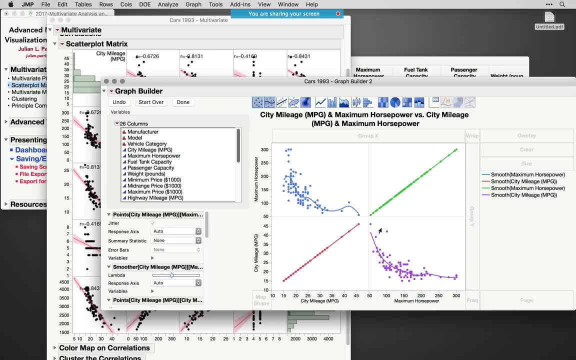 Notice. I'm dropping them to the right-hand side or to the above sections. We are pretty close. We have to right-click in one side. change that smoother. I'm gonna change it to a histogram And I'll turn the points off. 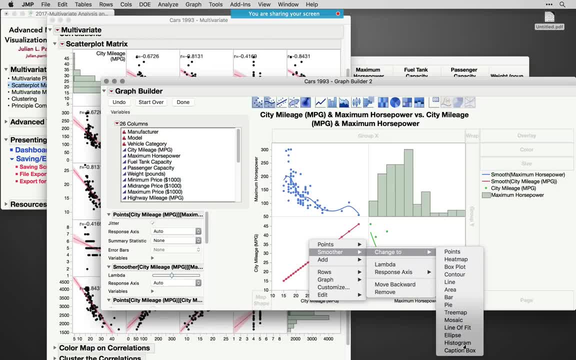 And I'll change this one to a histogram And turn the points off. So I basically just recreated a scatterplot matrix with histograms on the diagonal, But that took too long. even though it took a few seconds In jump time, that's still too long. 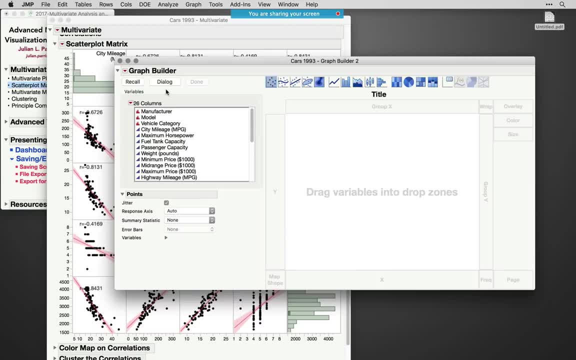 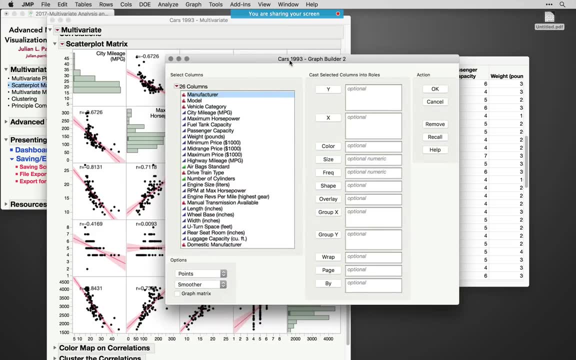 So the trick is- and this is a very useful thing to know- you can do in Graph Builder: click on the dialogue button And there actually is a dialogue version of Graph Builder. I quite love the interactive version, but if you're creating certain visuals, 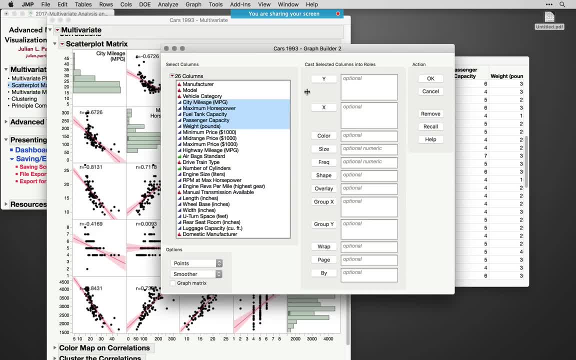 dialogue works very well To do this. you can actually grab those four variables. I'll click them into both Y and X And then I'll tell jump, I wanna create down here a graph matrix And I'll turn off the smoothers even. 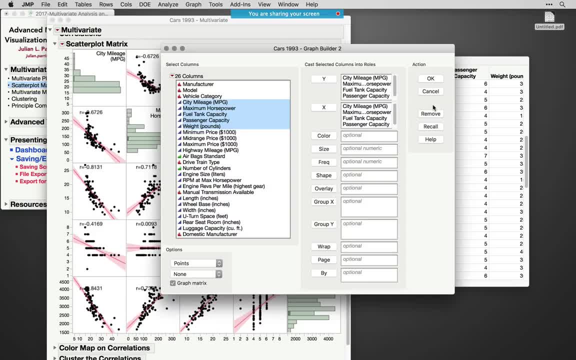 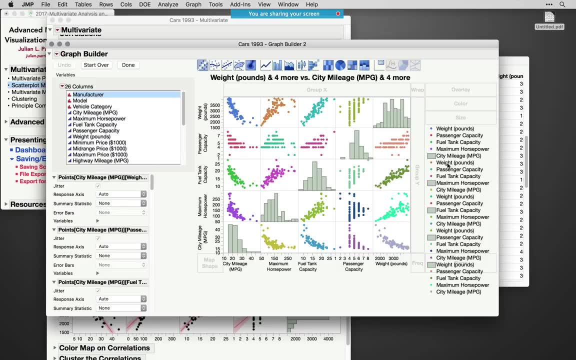 I'll just say none. So I'm only gonna look at the points, and I'm asking for a graph matrix. Jump will, when I click okay, create that graph matrix. Now there's a lot of coloration here that I'm not totally fond of. 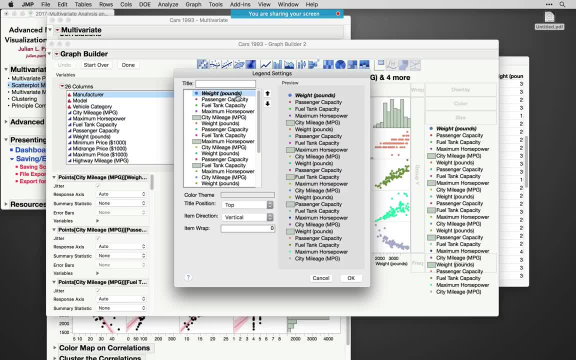 An easy way to fix this is double-click on one of the points, select all of the points here, And all I'm gonna do is right-click and I'm gonna say: make them all black. And, knowing that you can double-click an axis, 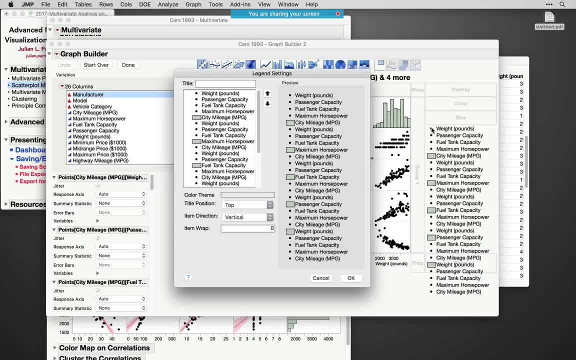 to get to the axis settings is really important Again. I just double-clicked one of the points: select everything. command A works if you're on a Mac, or control A if you're on the PC. click the point and then set the color. 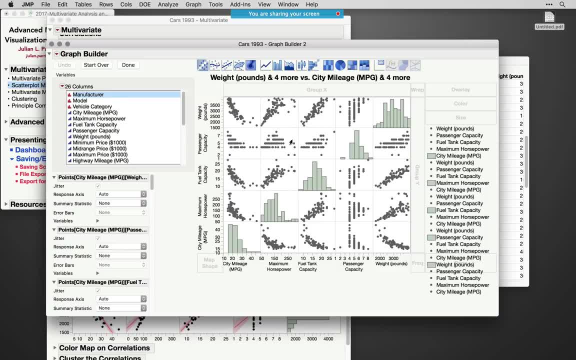 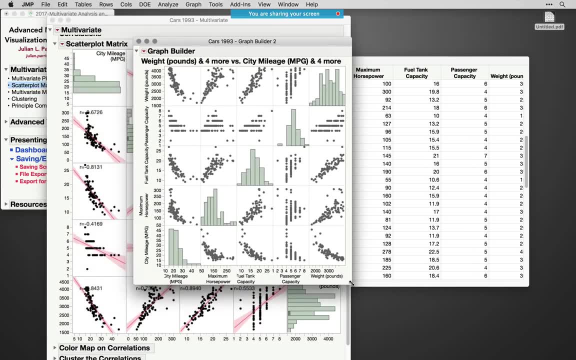 So maybe you don't want it to be black, maybe you just want dark gray, Right. so that's a nice way of setting those all. And remember I turned off the legend before. If I do that now and click done, I've gotten pretty close to the visual I made before. 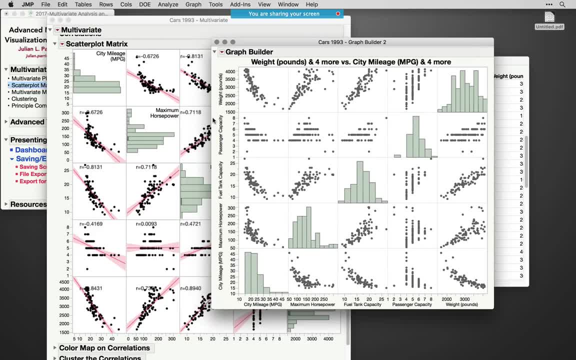 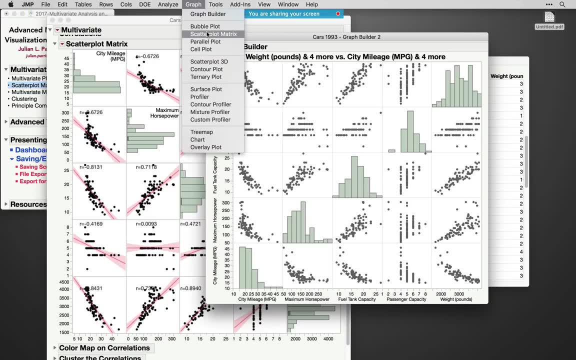 And so an easy way to use Graph Builder to even make your scatterplot matrices So a very useful thing that you can do. Now, just like we were able to using scatterplot matrix, we can do even more advanced things using Graph Builder. 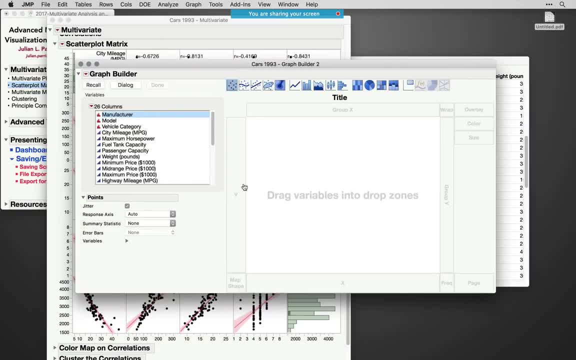 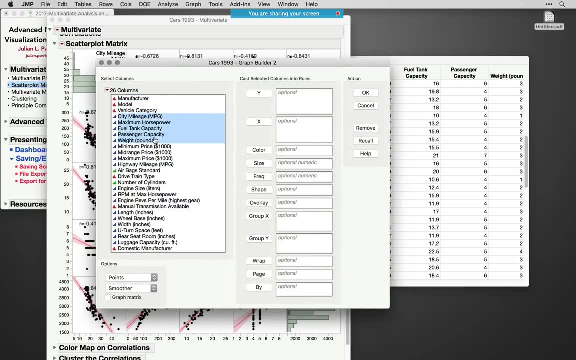 Again, because Graph Builder knows how to operate on not just continuous variables but also on categorical variables. Let's go into that dialog. I'll put in those four variables again, but actually this time let's add one additional. Remember vehicle category. 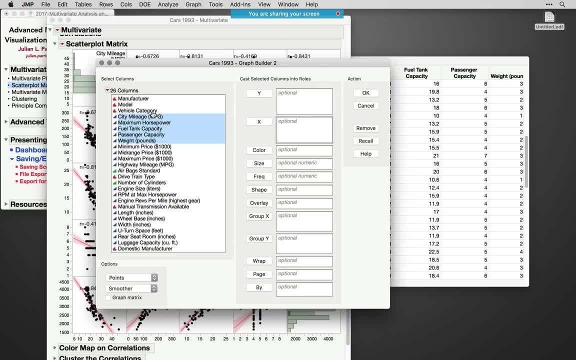 Let's- actually I'll even just- remove these, Let's just add them all at once. I'll take vehicle category, including the rest of those, and click them into the Y and X Now, if I ask for a graph matrix now, 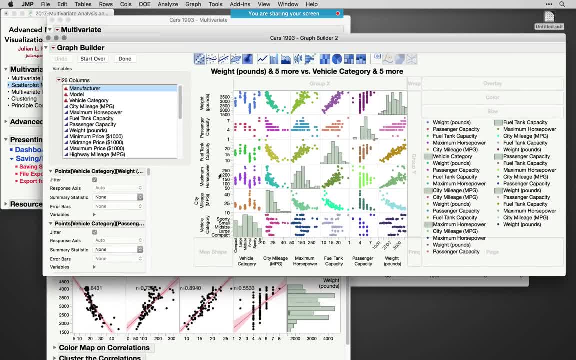 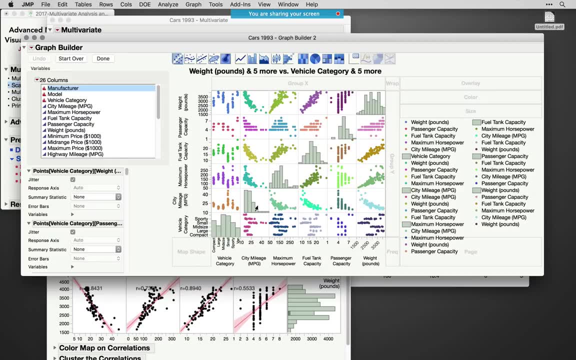 and I'll turn off the smoother Jump will do something very similar to what it did using scatterplot matrix. It grabs those points and sticks them sort of in their locations, jittered, But like we did before, I can right click and change those points to something else. 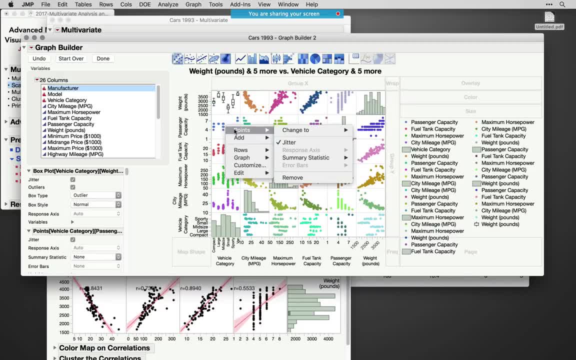 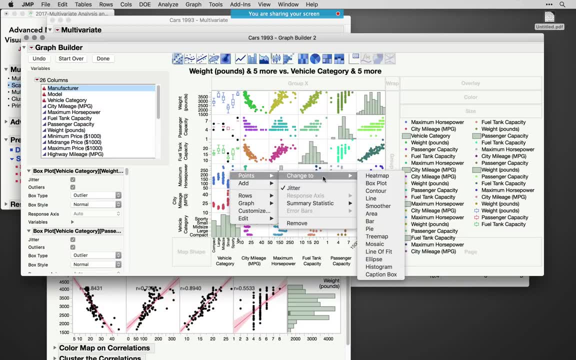 I'm gonna change them now to, let's use a box plot. I think that'll look nice for each of these, And so I'll do points changes to the box plot, And so I'll do this rather quickly, just to make the point that, if you 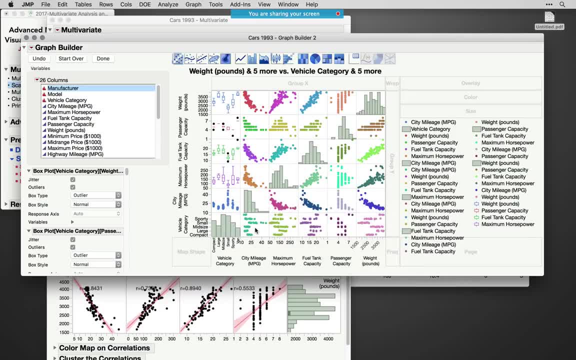 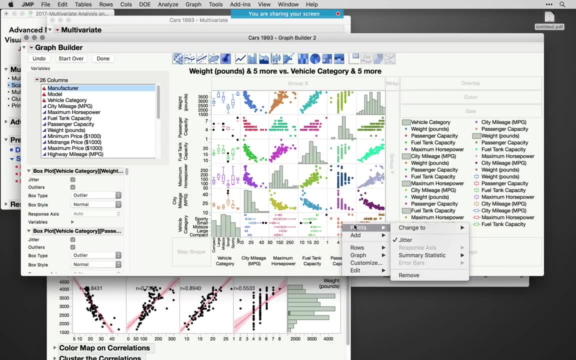 especially when you get used to Jump, you can do all these things rather quickly and create visuals that tell quite a bit in a small amount of space. And just remember that Graph Builder is one of these platforms and we have other webinars that'll go through a lot of this. 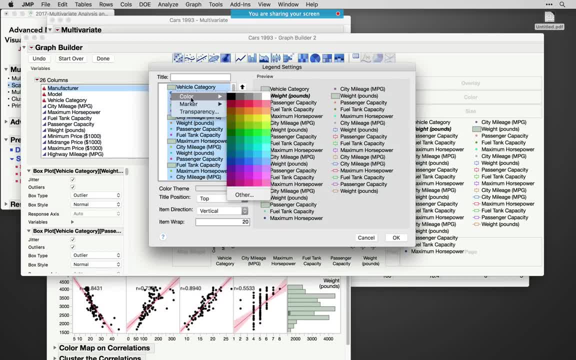 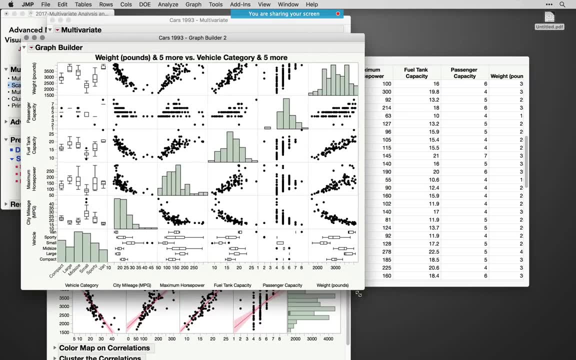 one of these platforms that once you've used quite a bit, and I'll just change the colors to black here and click done and turn off that legend and now we have kind of a neat visual that I really love. So involving a categorical variable. 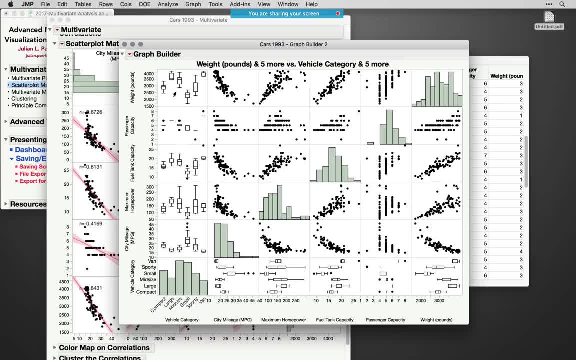 gives us the histogram for that, plus also the box plots as it relates to every other variable. So we get a lot of information density here rather quickly. And again, if this is something you're gonna make again, go to the red triangle: save script. 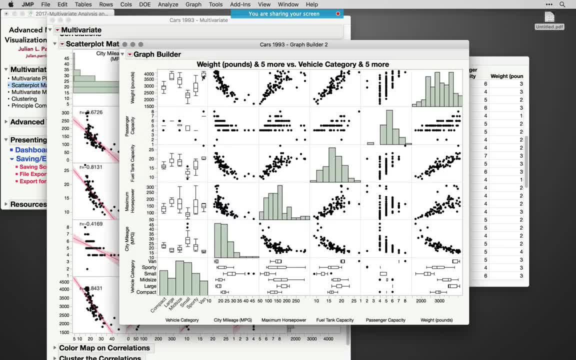 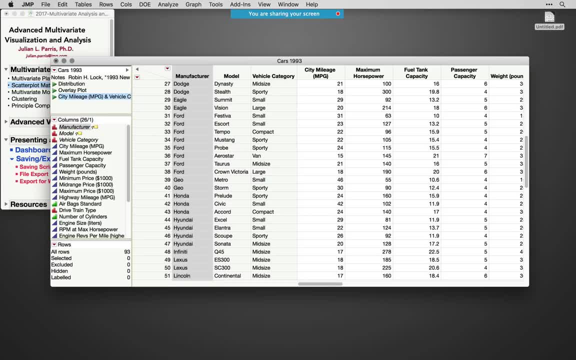 and drop that to your data table. And so a lot of flexibility in Graph Builder. Okay, so let's look at a different way. I'm gonna minimize the multivariate. We're not gonna use that anymore. Just to show you another way: Graph Builder. 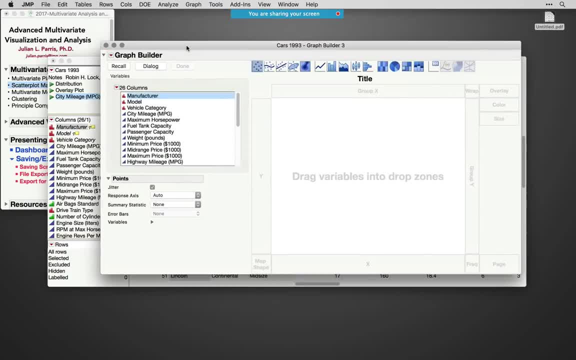 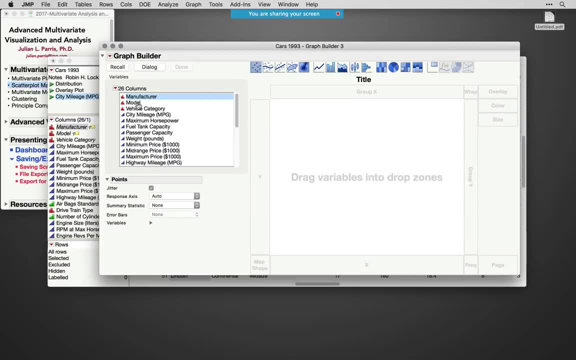 lets you invoke multiple variables. Of course, this is a visualization for multivariate data talk, so we wanna look at that Another way we can do it. let's start off with something categorical. Perhaps let's use manufacture on the X, And so this is the type of car we have. 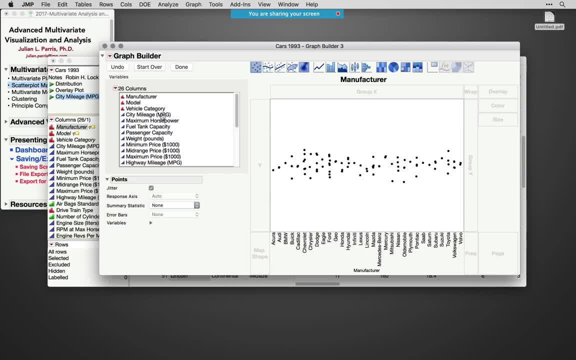 And let's say we're interested in city mileage and highway mileage, how those two relate to each other. So if I put city mileage in the Y and let's turn on, let's just do bars here to keep this low density- If I put in highway mileage, 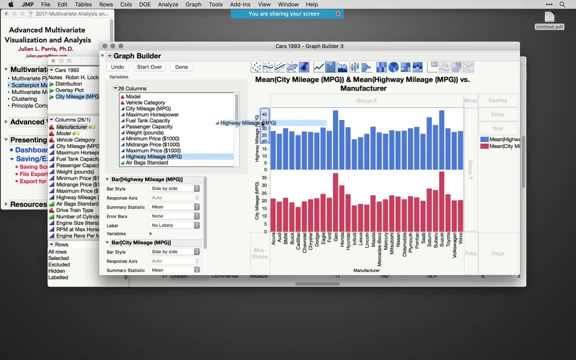 let's look at different places. I can drop this If I drop this above city mileage. although I can make a comparison, I can read off where Acura is on each. it doesn't do a great job of showing me at an instant. 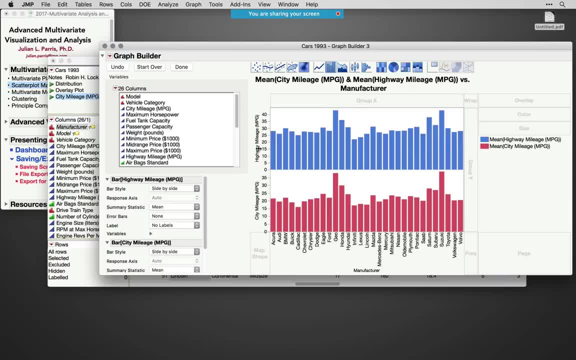 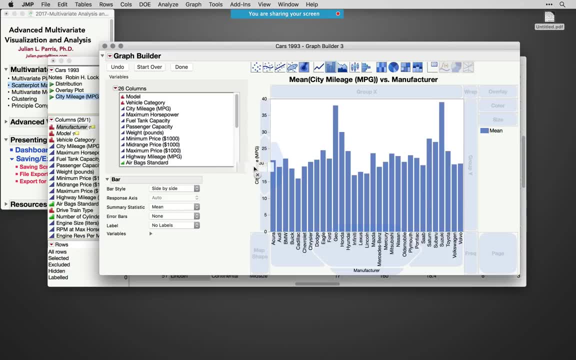 whether a manufacturer has a wide variety between highway and city mileage. So dropping the variable there- I'm just gonna drag it out- isn't particularly useful to me, But there is a drop zone right inside of the graph. Notice what happens when I drop inside. 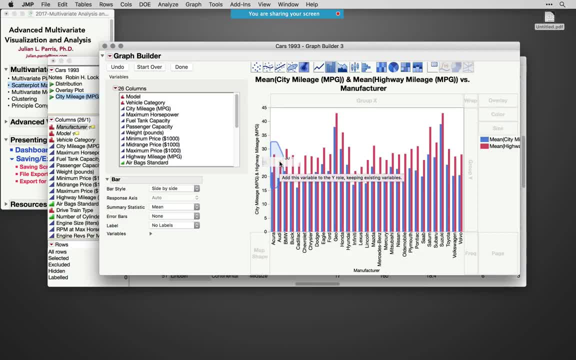 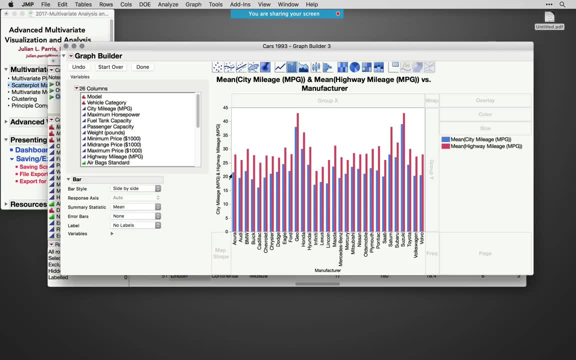 I'm adding this variable, keeping the existing variable, but adding it inside, And so for each of the manufacturers, I actually now have one of each. So what it is for highway and what it is for city And under the bar style is how I control. 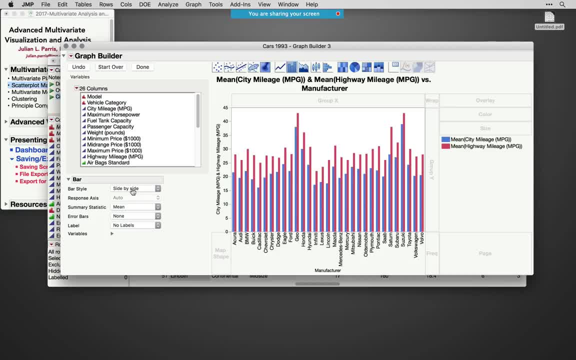 how this is displayed, Because what we're actually looking at here is side by side. There's a great option called nested, which I quite like, because notice what nested will do is take one of those variables, In this case, the first one we entered. 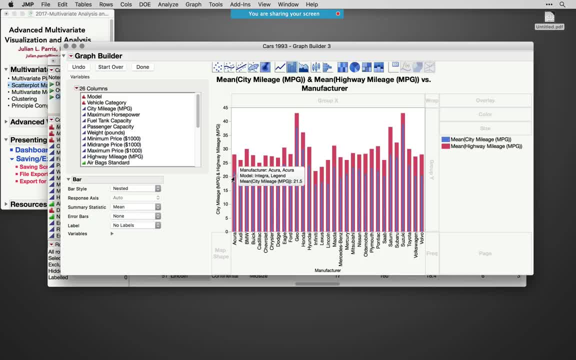 So the mean for the city mileage and it's going to nest it inside of highway mileage And that ends up being exactly what we want, because city mileage is always lower than highway mileage on average. We can look across the different manufacturers and actually see that difference. 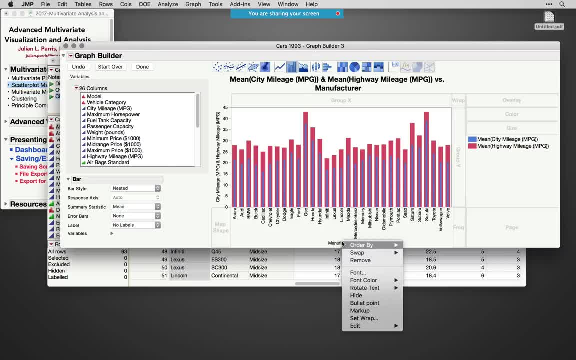 And we can do some clever things with it. Let's look at this. You may not notice it, but if you right click, there's an order by option, So I can actually order these manufacturers by one of the variables in the data set. 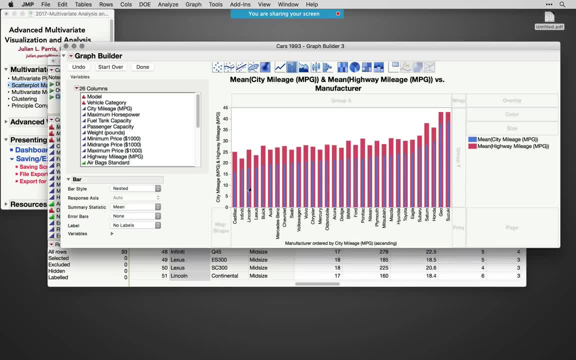 Perhaps I wanted to order by city mileage ascending, And so we're looking at the blue bars will always be ascending and we can see how that changes with the highway mileage. You know, maybe we also wanna. let's order by something even more clever. 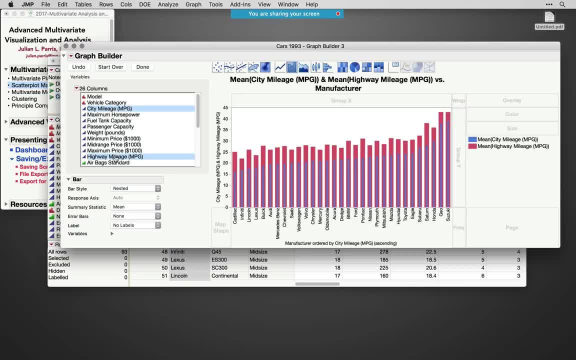 What about the difference between city and highway mileage on average? So which manufacturer has the biggest difference between those two? So I can actually write inside of graph builder: right click, I'll do combine and make a difference. So I'm making a difference score. 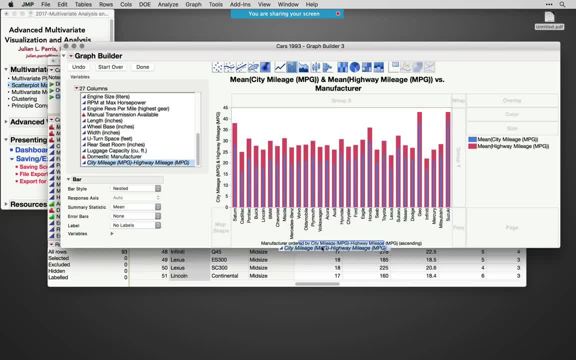 between city mileage and highway mileage, And now I'm gonna drop this into the drop zone just below the graph. So notice there's places I can drop this. It's a manufactured ordered by that ascending, And so we're actually looking at here. 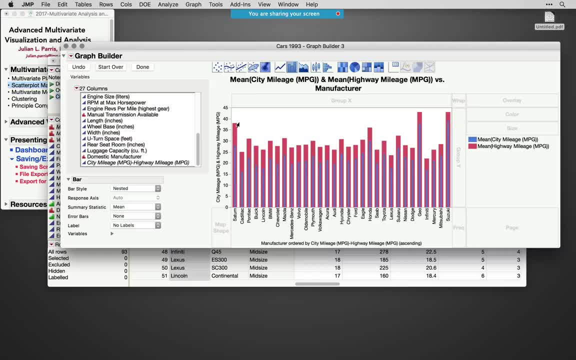 which are the ones with the largest difference, And so Saturn's. for some reason, they just. they may do well in city, but they do poorly on highway, Whereas Suzuki and Mitsubishi tend to have a very small difference between those, And so notice that ordering gives us even ability. 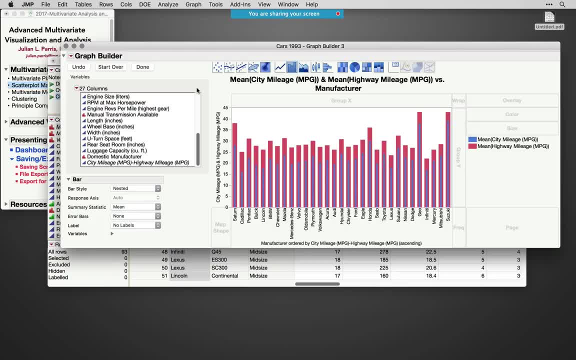 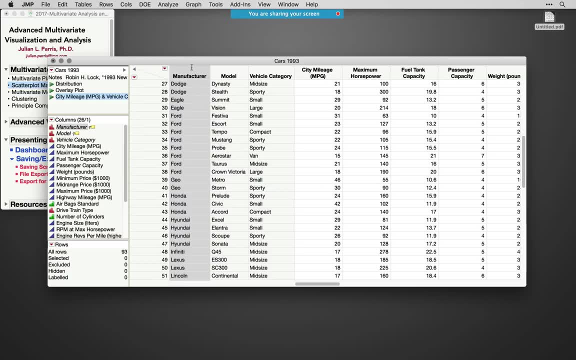 to tell a story nice and conveniently with our data here. All right, so I'll hit done. Let me minimize this. All right, so let's look at a couple multivariate ways we might work with two numeric variables, And I'll start this with graph builder. 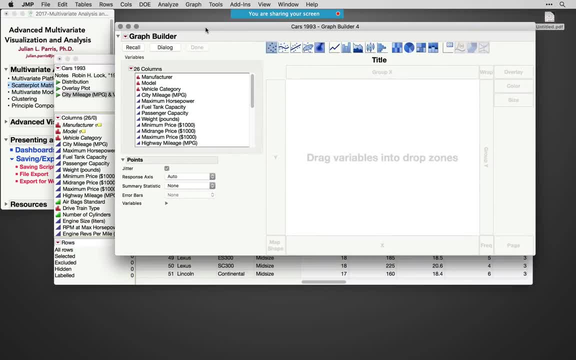 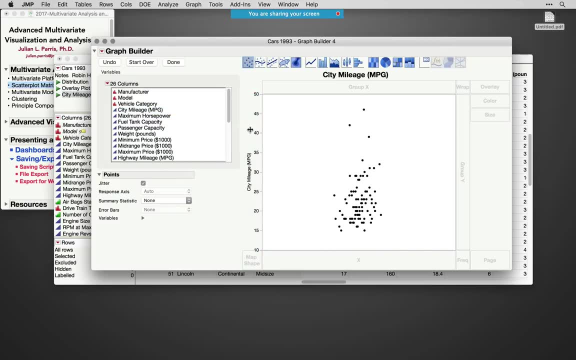 but we're very quickly gonna go into a multivariate, a platform called fit model. And to preface this, let's look or think back to a relationship we saw. We saw city mileage versus horsepower And we saw that there was this relationship. 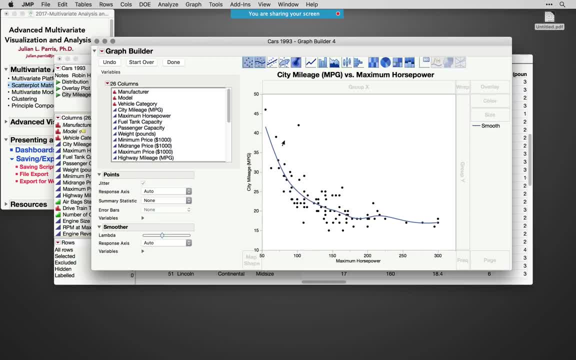 where cars with higher horsepowers tended to have lower city mileage And there's a bit of curvature to that. This is telling me, probably, that a transformation might linearize this. So, looking at horsepower, maybe the log of horsepower might be interesting to us. 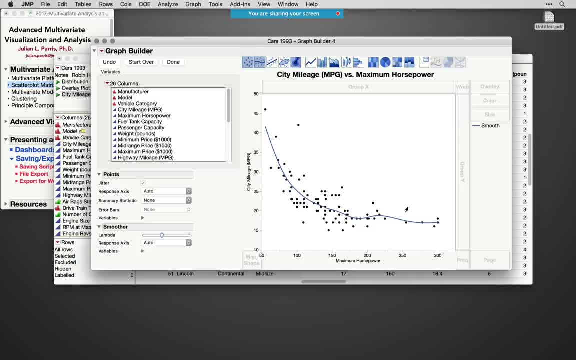 We don't have to get too advanced with that yet. But let's start off with the idea of thinking how this relationship maybe relates to the weight of a car, And we know that as we get cars with larger weights, their mileage went down as well. 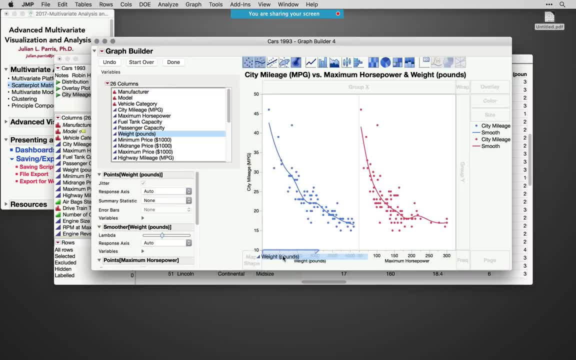 In fact I can double plot that here. I'll just put it to the left: So cars that are heavier have worse city mileage and cars that are more horsepower have worse city mileage. But what's gonna happen if I use this variable, the weight variable, and then I multiply it by a car? 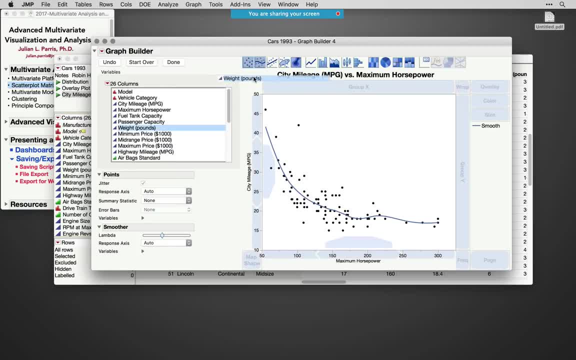 and then I multiply it by a car and then I multiply it by a car in one of the other roles, the roles that breaks up the relationship, So I can do group for x And notice what jump does is breaks our weight. 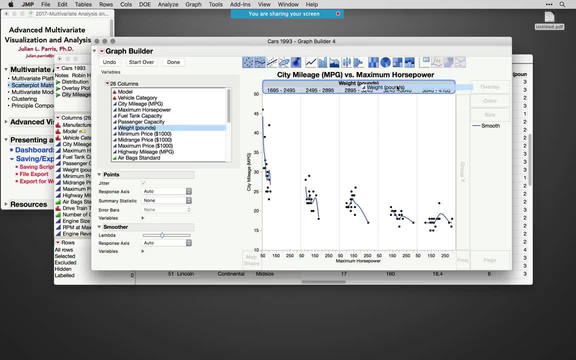 It's a numeric classification. It breaks it up into five sections for us, So five sections with an equal number of points. I can do group y. It breaks it up that way too. I can do wrap And I can do overlay. 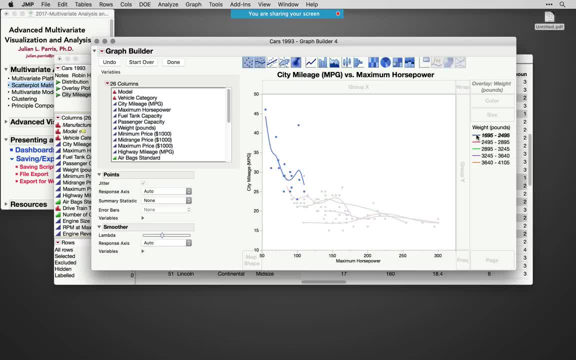 So I'm gonna stop here on overlay for a second. And I want you to notice something: If I click on the lowest weight class, it looks like there's a pretty sizable negative relationship. for very light cars, A little bit of extra horsepower is really hitting their gas mileage. 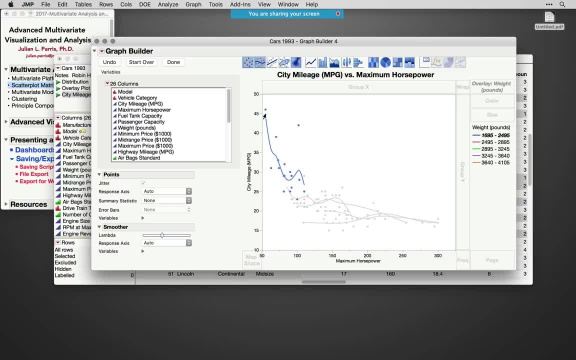 which maybe makes sense. If your car is very light, you're gonna get really great gas mileage. if you have very little horsepower, There's not much drawing on that, But even if you add a little bit it's going to really dig into that city mileage. 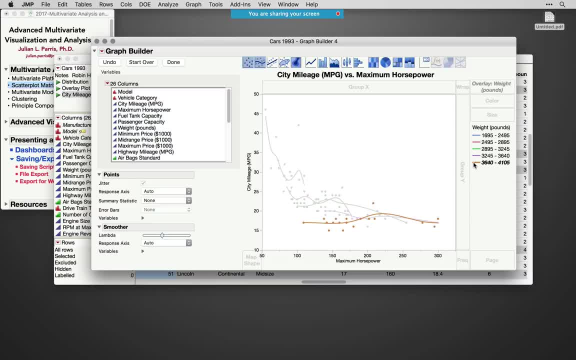 As I get to very heavy cars. there's almost no relationship Among the heaviest cars. horsepower didn't seem to relate at all to city mileage. They're already so heavy, They're so worthless for mileage That your horsepower doesn't really matter too much. 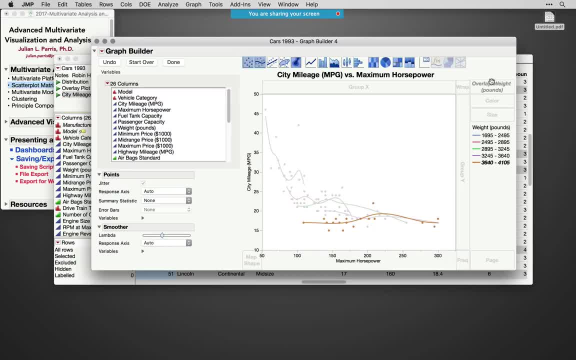 So we're looking at an interaction here between two quantitative variables. But I want to show you something as far as visualizing this, because I think this visual does not tell that story clearly at all. There's too much noise happening What's actually quite useful in Jump. 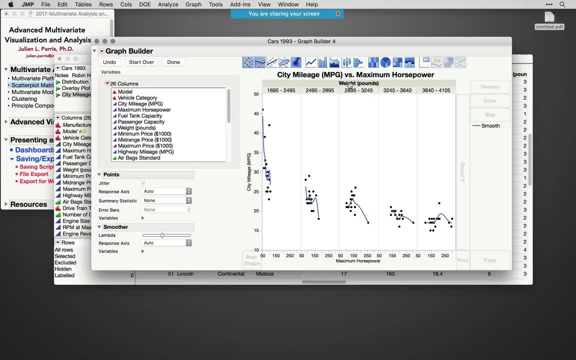 let me go to the group for X. You may not have known this. even if you're a Jump user, If you right click the group X axis, you can tell Jump how many levels you want it to use for that grouping. So it's creating the groupings for us. 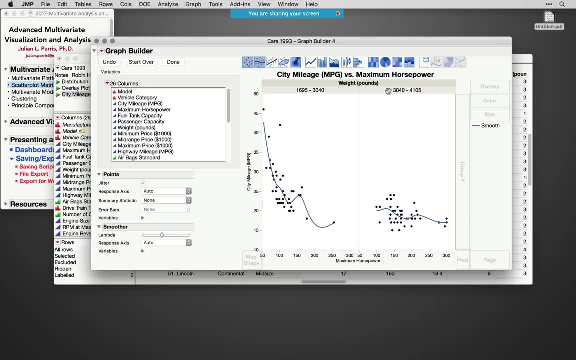 And I'm going to tell Jump just to make two. So I want a low and a high. So the low weight goes from 1695 to 3040.. And then the high weight goes 3040 to 4105.. If I now drag that variable to overlay. 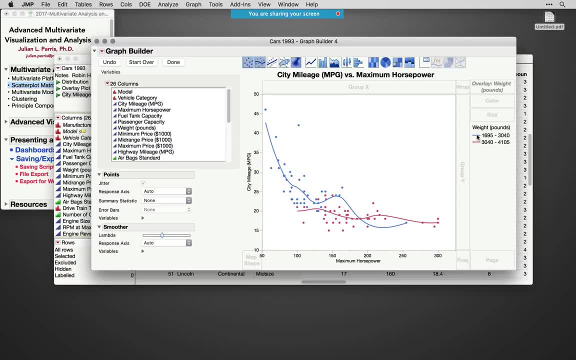 Jump honors the fact that I told it to use only two levels, to now have a two level grouping, And so weight in pounds, without me having to make my own binning formula, which is actually very straightforward to do as well, but just doing it graphically. 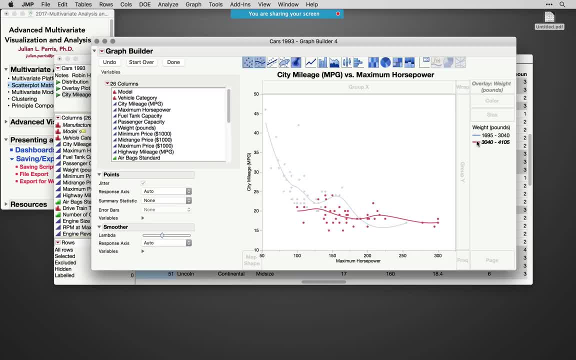 I can create this right inside of Graph Builder. So this is the binning relationship that we just observed before but now shown more clearly. Among the heaviest cars, very little relationship between horsepower and mileage, And along the lighter cars, quite a bit of relationship. 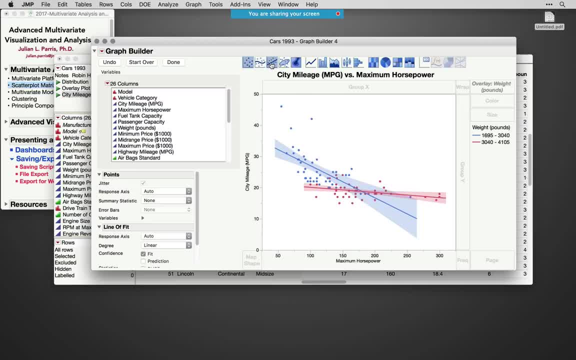 Now this distinction we can look at even as linear regressions, So I can turn on the linear regression line Again. this is doing it on a subset of each of the variables, And so this gives us a nice way of exploring that relationship. 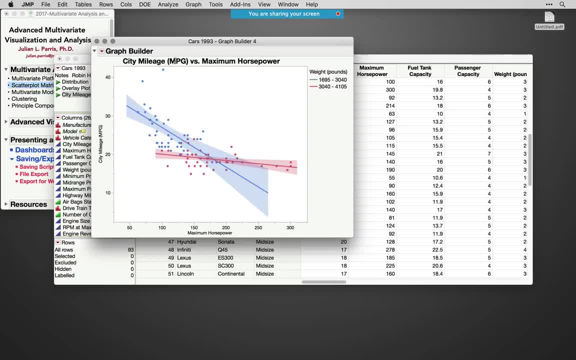 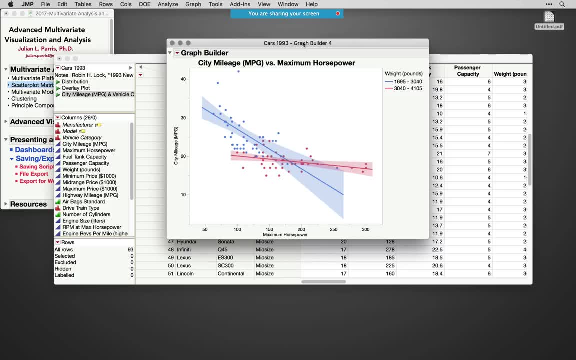 without having to make the binnings or do the proper modeling yet. But let's do the proper modeling, because this becomes a very interesting way to teach multivariate regression and to talk about interactions between variables, which is actually a very difficult thing traditionally to visualize. 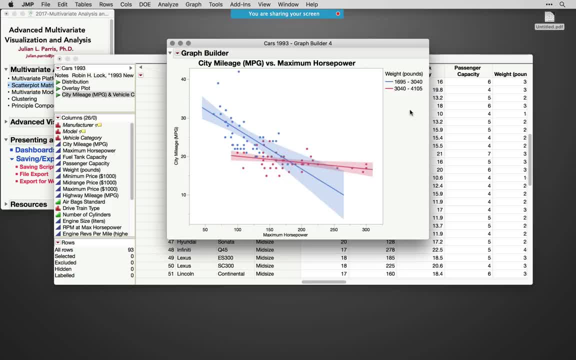 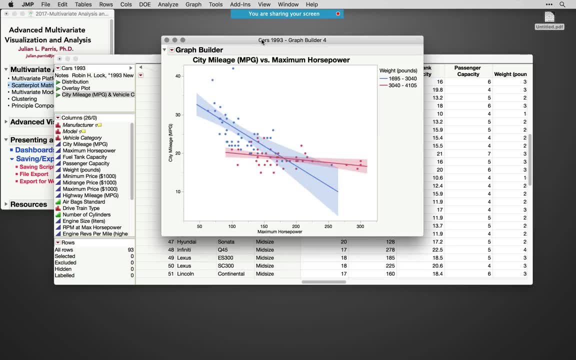 especially the interaction between quantitative variables. So a bilinear interaction term is one of the more mysterious things, especially when teaching new students. It's a hard thing to grasp. So let's start by talking about how we would get into that analysis And that's gonna take us into. 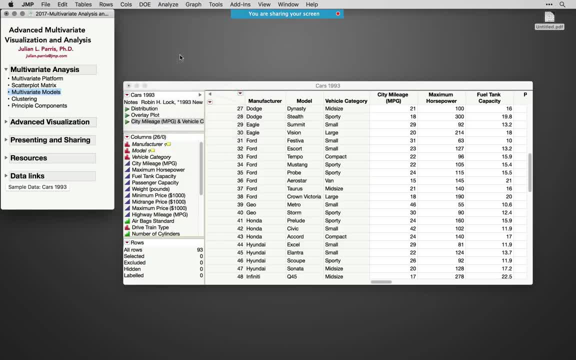 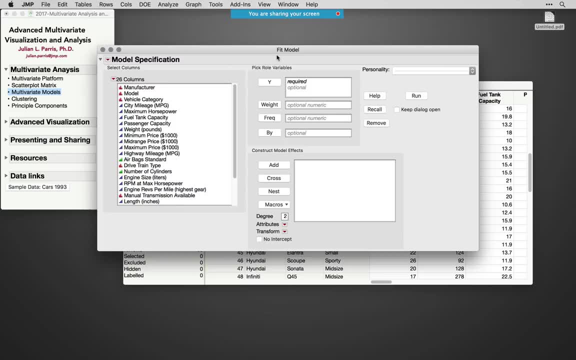 the fit model platform, And fit model is useful any time we're working with more than two variables. It's fine with just two, but it is a platform that's designed for working with more than two variables, So let's define those variables. 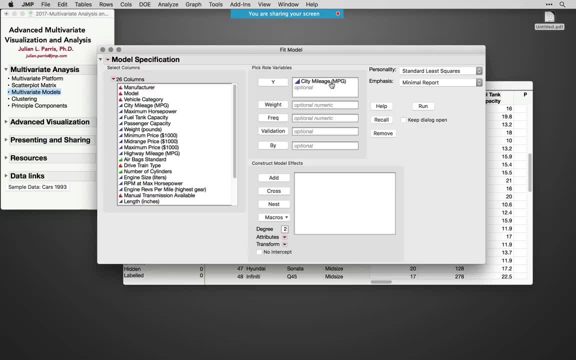 I'm gonna put city mileage as my y, so what I'm trying to predict, And I'm gonna use horsepower and weight as my x. So I've selected them both on the left hand side, And the reason I selected them both before entering them into the model effect. 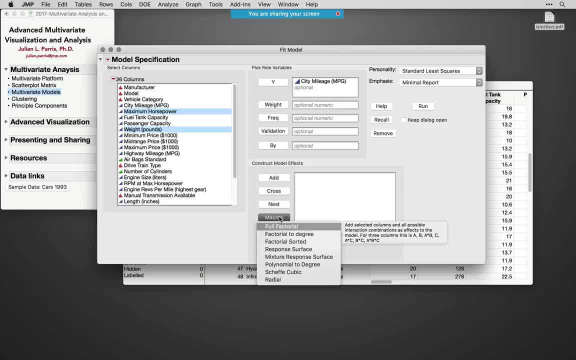 is because I want to use a macro. I want to use a macro that says: create full factorial effects using these two variables, Which means create main effects terms. So how much does maximum horsepower on average, holding everything else constant, affect city mileage? 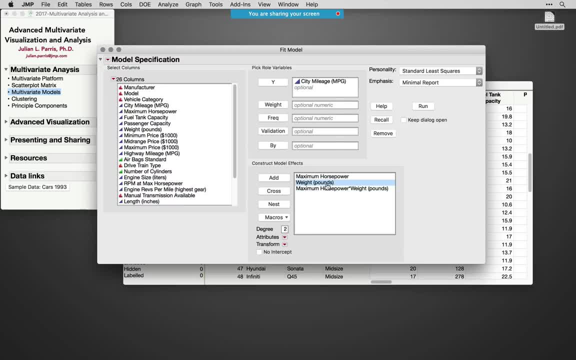 How much does weight on average, holding everything else, constant change with city mileage? And then this bilinear interaction term, which basically says how much does increases in maximum horsepower attenuate or strengthen the relationship between city mileage and weight? Or, said differently, how much do changes in weight? 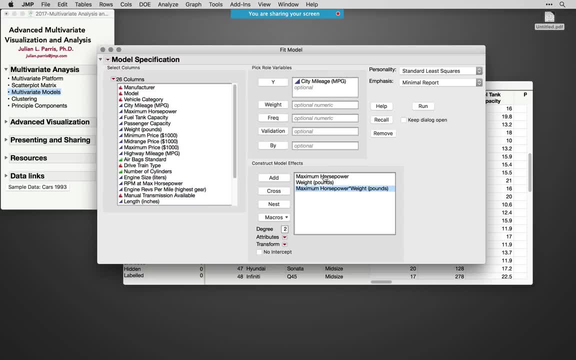 attenuate or strengthen the relationship between city mileage and horsepower. So how does one variable affect the relationship between the other two? That's what an interaction term is, But it's often a very hard interaction term to visualize or to think about, but something that Jump does quite well. 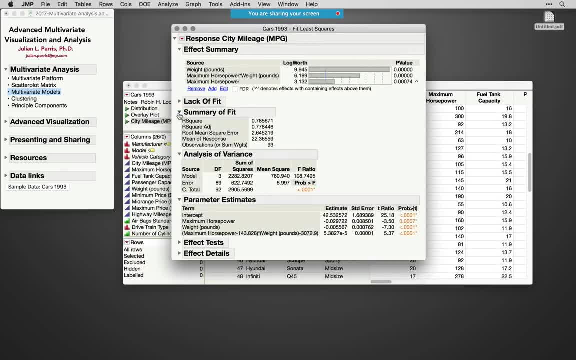 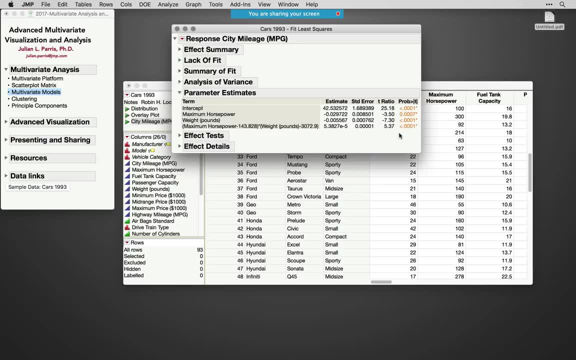 So I'm gonna click run And before we create a visual, I'm just gonna clean up our output. I'm just gonna minimize some sections And let's just look at our parameter estimate section here And if we're looking at the p-values in this data set, 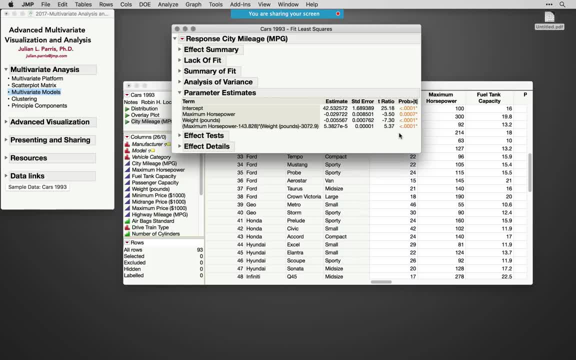 everything is statistically significant, not because it's fake data, just because these are very obvious relationships. But we are seeing the relationships we expected. As you have cars with more horsepower, they tend to be cars with lower gas mileage. As you have cars that are heavier, 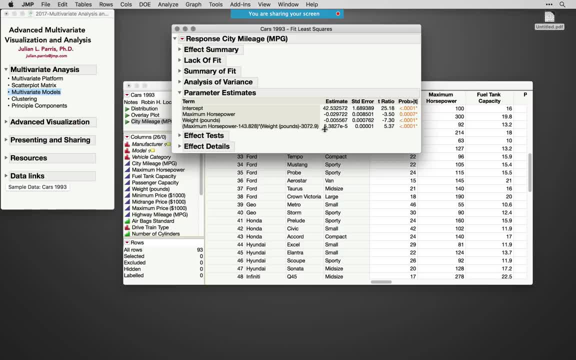 they also tend to be cars with lower weight. And then you have this estimate for the interaction term. Now it's beyond the scope of today to talk about why there's the minus here. Just know that that's because the variables are centered before the cross product is taken. 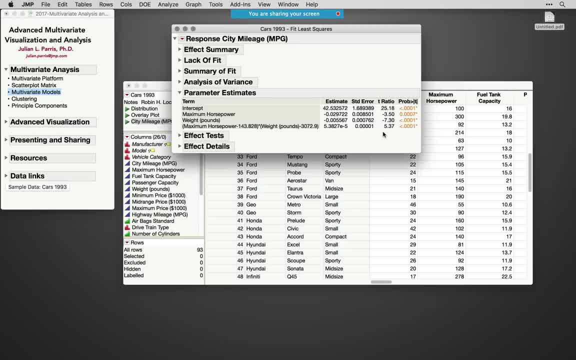 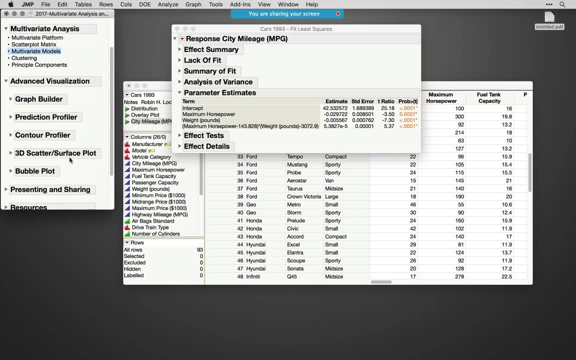 But what we're seeing here is a negative coefficient for this interaction, which basically means an attenuating relationship. As you increase one variable, the relationship between y and the other variable will get less steep. How on earth would we visualize this? And so this takes us to a couple of visuals. 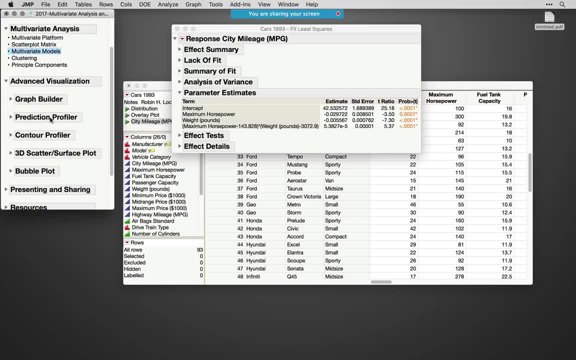 that I quite love, And the first- probably one of the things that first made me fall in love with Jump- was this prediction profiler, And the prediction profiler under the red triangle in fit model is under factor profiling and it's right here called the profiler. 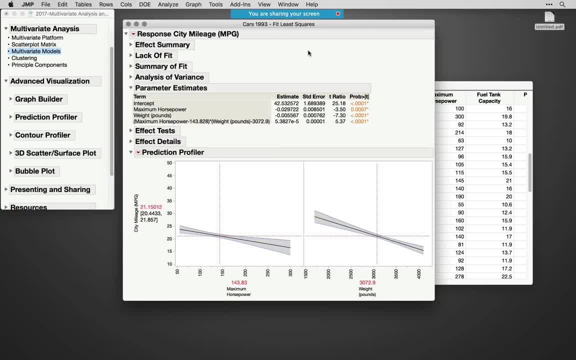 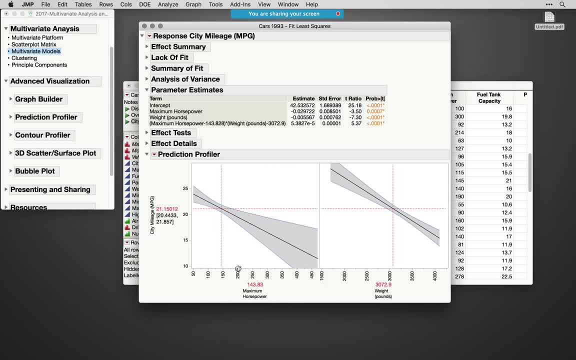 And the profiler is one of these magical things that lets you look at what the terms in this model actually mean, And I'm just gonna drag up some axes just to clean things up before I start moving things around And what you're gonna see when I move things around. 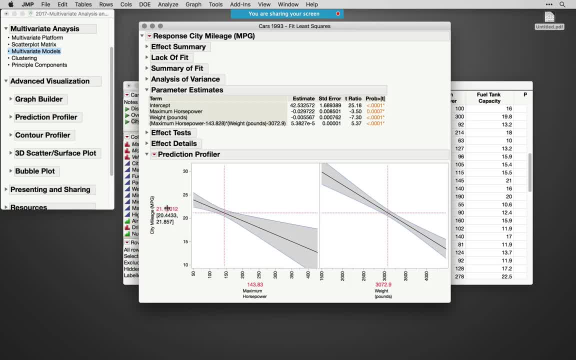 is, two things happen. First, the prediction on the y, so we're looking at predicting city mileage based on how much of each of the inputs, based on how much of each of the inputs, based on what variables we have, And so, as I drag and you can drag things around here, 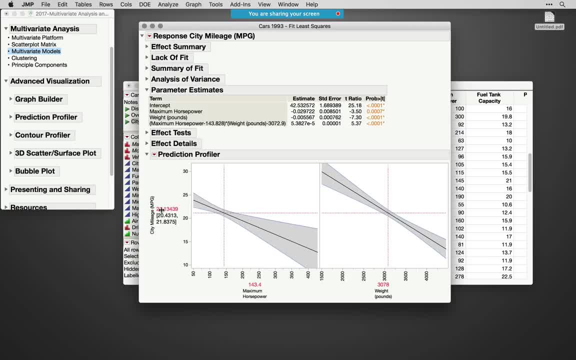 and change how much a car weighs or how much horsepower it has, you're gonna see the city mileage estimate change. So cars that have 200 horsepower and are 3,500 pounds tend to get 18 miles to the gallon on average. and there's the confidence interval. 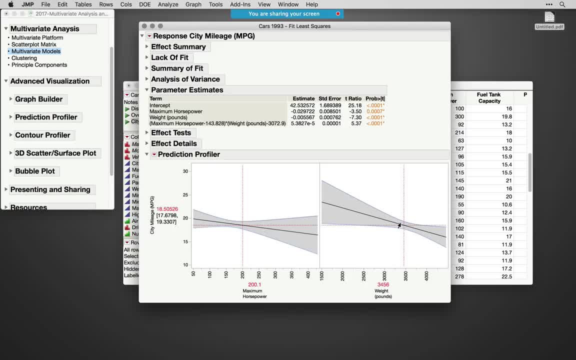 But as I did that moving, you probably spotted it because it's very obvious and I'll just point it out right now. Watch the coefficient or watch the slope between mileage and horsepower. So keep your eyes where my mouse is here, But I'm gonna move. how much our car weighs? 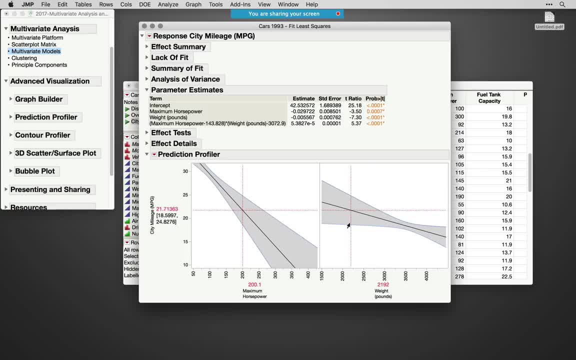 So among cars that are very light there's a very large relationship, very positive- or I should say negative slope between city mileage and horsepower. But as I get to cars that are heavier that relationship flattens out. And remember that's what we saw in graph builder. 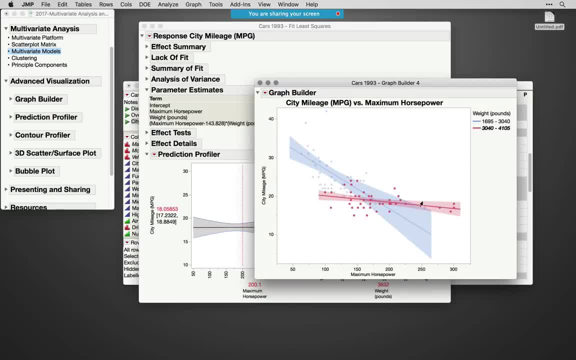 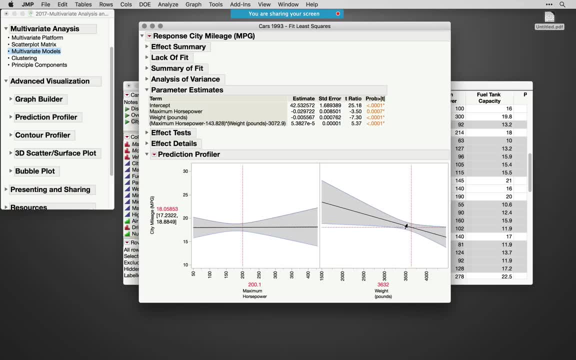 when we just made the two level split. Among cars that are heavy there's a pretty flat relationship between horsepower and city mileage, But among cars that are light there's a strong relationship. So we're now profiling this interactively. That is the continuous regressor form of that interaction. 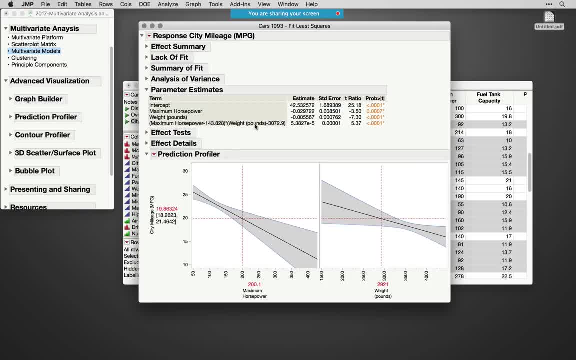 And that's what that negative coefficient means As I move literally above the mean of one variable. that's what the minuses are all about. Those are the means of each variable. As I move away from the mean and the positive direction, we're taking a little bit of the relationship. 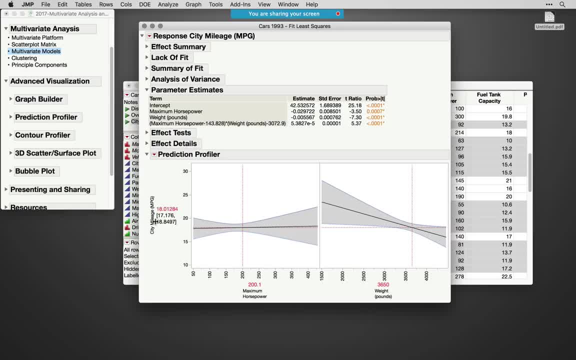 this amount away from the slope of Y city, mileage and horsepower, And there are only needs, And there only needs to be one coefficient here, because that interaction is actually symmetric. And this is another place where jumps, visualizations help. you see why. 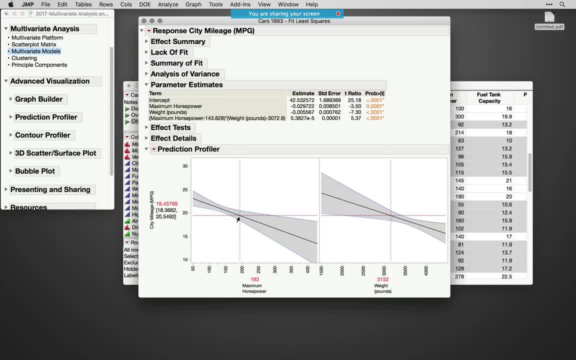 What I'm looking at here is a two-dimensional representation of the three-dimensional response plane fit through the three-dimensional points of these three variables. So there is, in three dimensions, a cloud of points. I'll go to graph scatterplot 3D. 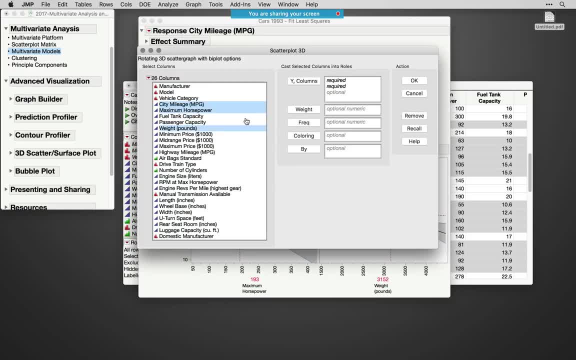 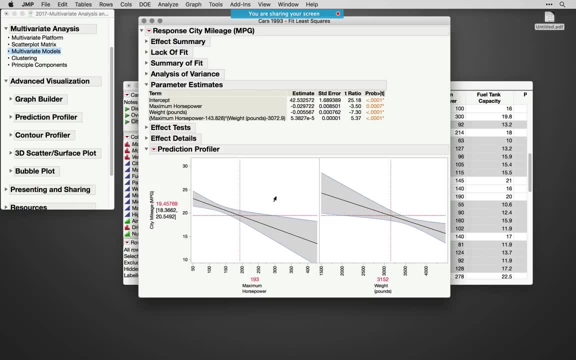 just to show you those quickly. So I'll take city mileage, horsepower and weight. So in three dimensions there is this cloud of points And what we do in multiple regression is fit a response plane through it, just like we do with two-dimensional points. 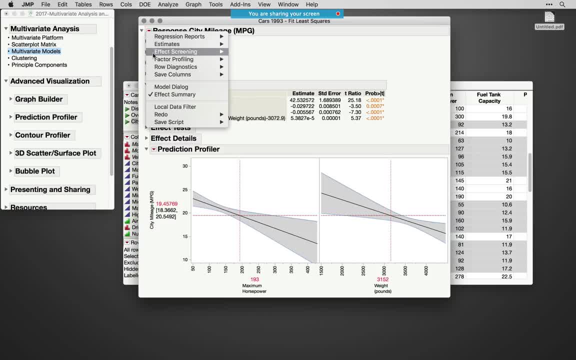 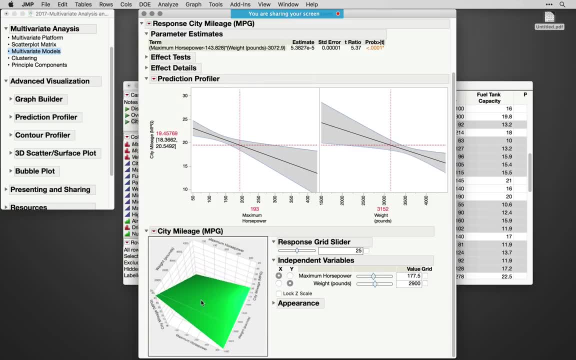 and fit a line. So let's look at that response plane. Under factor profiling there's the surface profiler, And the surface profiler lets us see the curvature of the response plane. Notice that that is not a flat plane going in three dimensions. 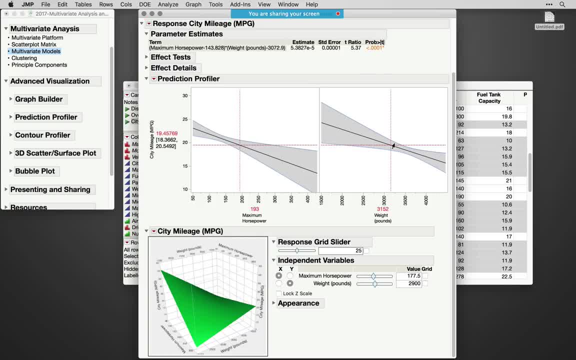 The curvature is this estimate here, that interaction term, That curvature is responsible for the response plane. It's responsible for why, as we get higher in weight, there's a flat relationship between city mileage and horsepower, or similarly and symmetrically, as we get to a high amount of horsepower. 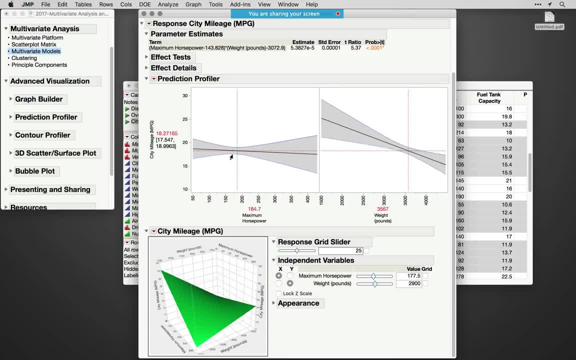 there's a flat relationship between weight and city mileage And as we get to very low horsepower there's a strong relationship in the negative direction. So the curvature of the response plane is what's accounting for that, And this is a way we can see it. 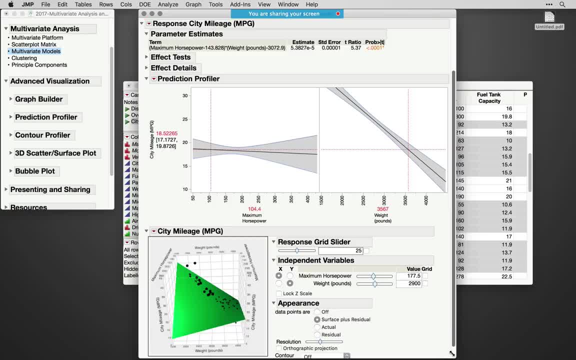 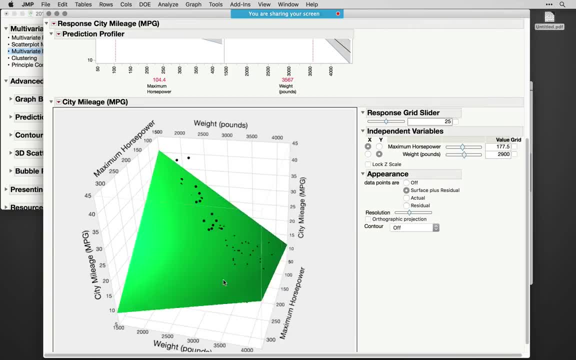 And in fact, if I click under appearance and turn on the surface plus residuals, I'll just move this up so I can make it a little bit larger for you. Let's make this nice and big And I recommend this if you're ever teaching multiple regression. 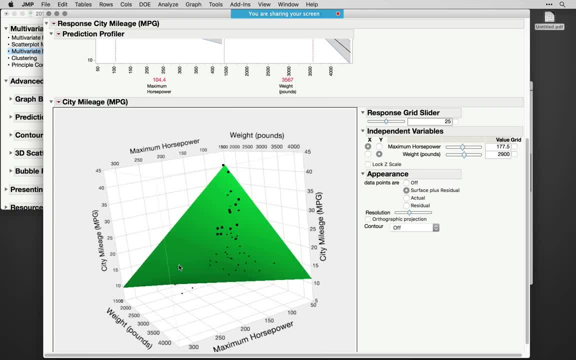 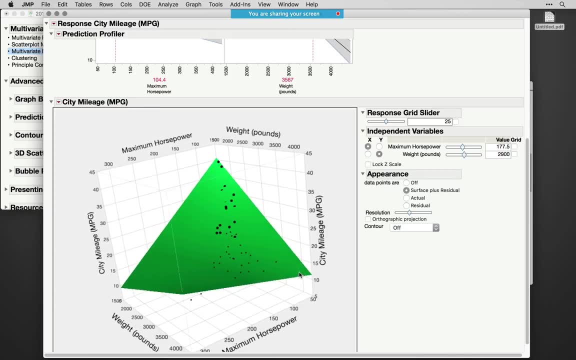 So being able to interact with the response plane, that is, the plane that minimizes the sum of the square residuals from the points to the plane, the points to the model. That's what a residual is, And so what we're looking at here is that response plane. 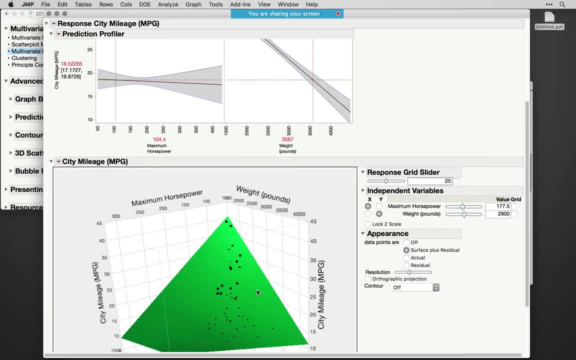 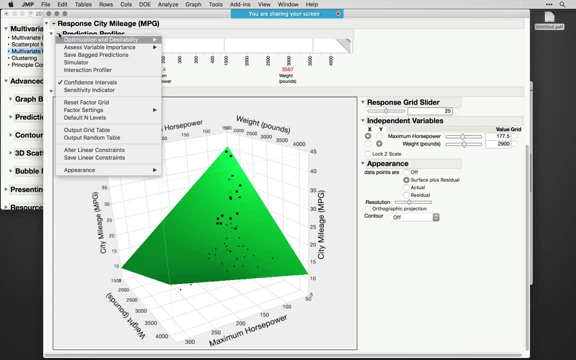 and that relationship that we observe in the profiler is really there in the response plane. So what's another way of seeing this? And this takes us to the contour profiler, another thing I love to see. So under the red triangle, under factor profiling, 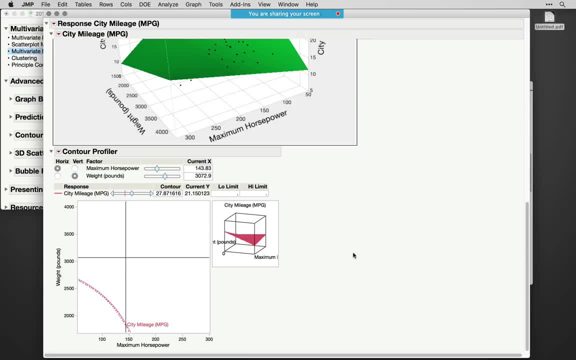 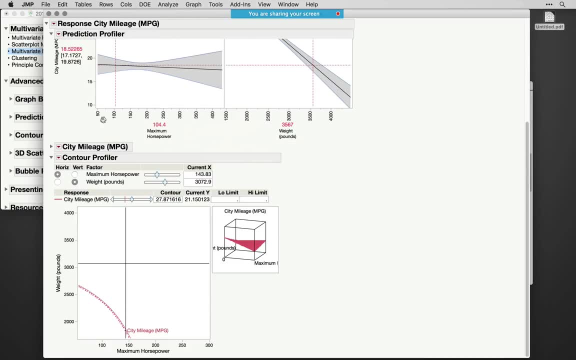 there's also this contour profiler, which is a two-dimensional way of seeing the three-dimensional response plane, And so I'll actually minimize a couple of these just so we can keep our screen somewhat clear. There's so much fun stuff to look at. 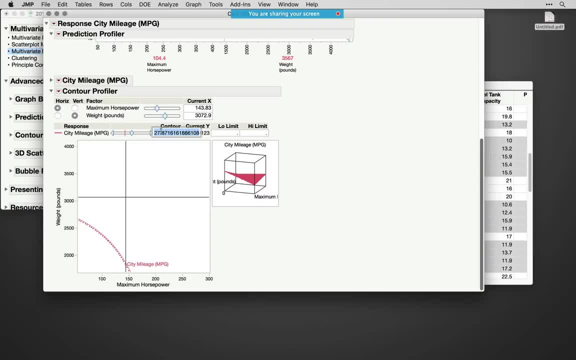 So here what we're gonna do. I'm gonna pick a particular mileage. Let's say, what do we have to have in terms of horsepower and weight to get 30 miles to the gallon? This is the contour Notice: it's not flat across. 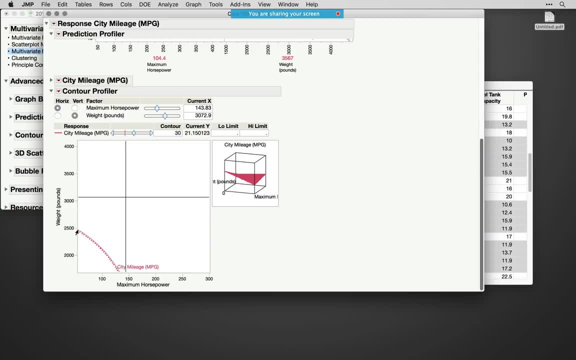 There's an interaction, so you're not gonna get straight lines here. You have to be somewhere on this curve to get 30 miles to the gallon. If you wanna get 20 miles to the gallon, you have to be along this curve. 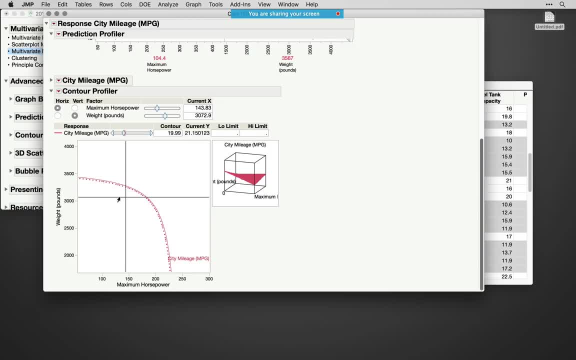 And notice that each variable there's some place or some amount of each that you can get. that'll give you 20 miles to the gallon, but you always get 20 if you're along this line, And so there's a fun thing we can do here. 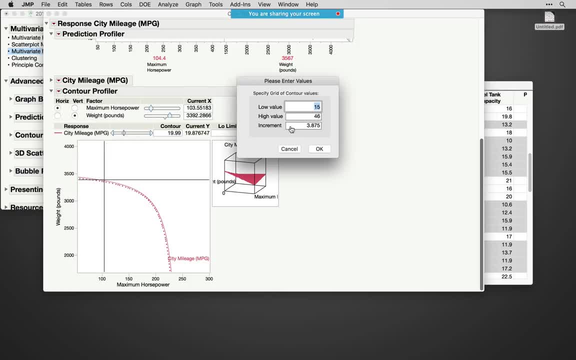 I like turning on the contour grid. If I do this, it'll give me a low value and a high value. This is for city mileage and the increments, And let's do it in five mile increments and I'll go up to 45.. 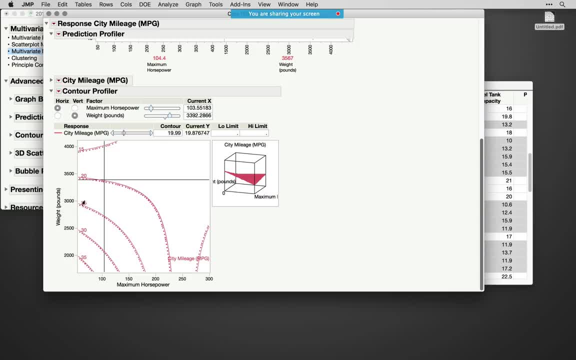 Click OK And notice what we get. here are, for each of these different mileages, what we have to have of each, And I'll just drag out the axis here Now. it's gonna look a little strange that you have these curves like this. 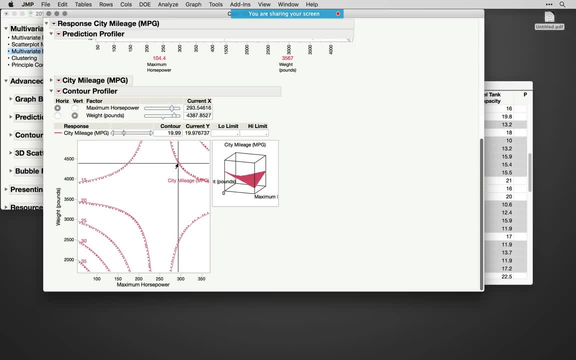 Turns out that that's not that strange. Those are also places where you can get, in this case 20 miles to the gallon. So these contour lines, just like we're looking at topography, give you a way of seeing the response plane. 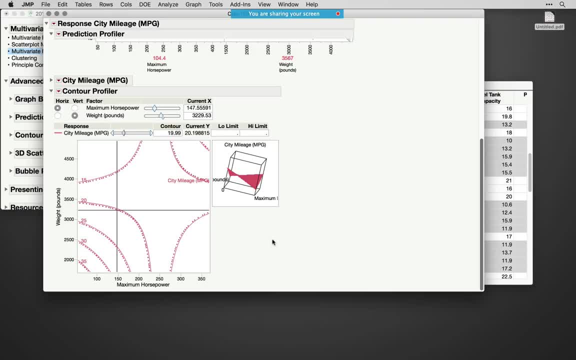 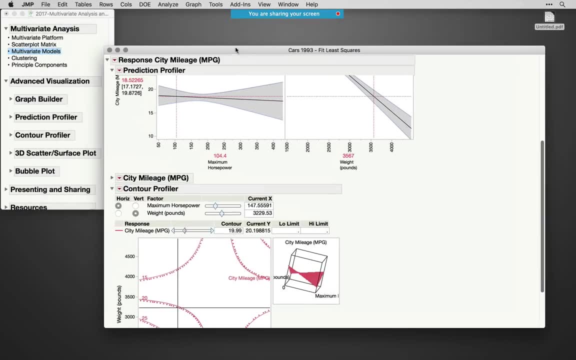 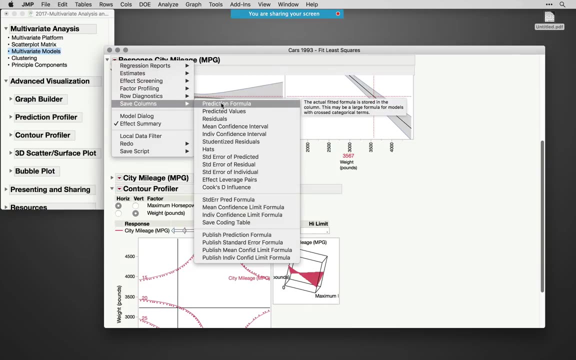 but in two dimensions, And so once you get used to seeing these, they become an excellent, excellent way of visualizing the three-dimensional relationships. Now I'll mention, under your red triangle for the fit model, under Save Columns, you can save out a prediction formula. 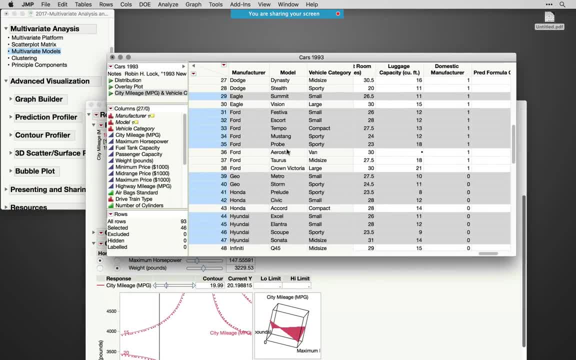 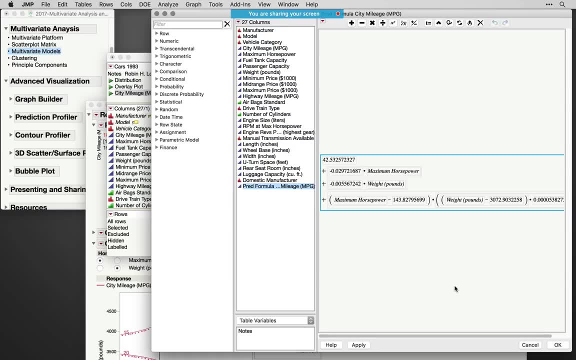 And if you do this, the prediction formula actually has enough information to be able to take into consideration what it is if I go over to it. This is actually if I right-click and go to Formula. this is the formula for predicting observations. 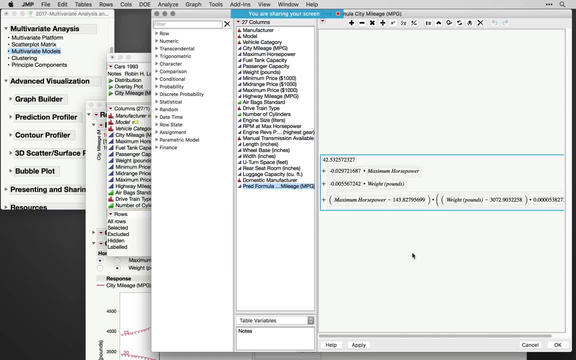 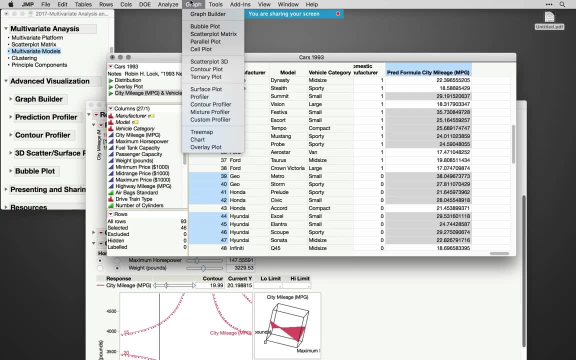 It's basically the linear regression line that we've saw before, or sorry, I should say the response plane we saw before. That prediction formula lets you invoke under the graph menu those profilers directly. So there actually is a profiler under the graph menu. 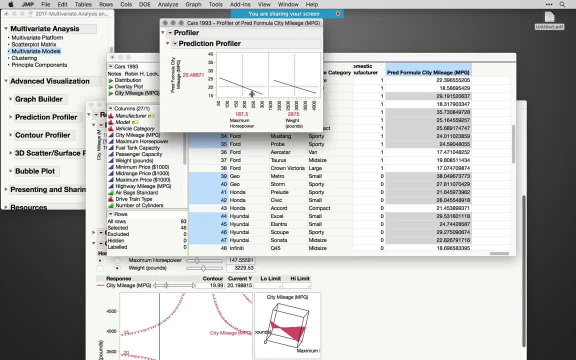 that only needs a prediction formula. When I click it in, there's your profiler, the one we saw before, And so you can profile and you can see there's a graph that's actually a profile And you can see that there's a graph that's actually a profile. 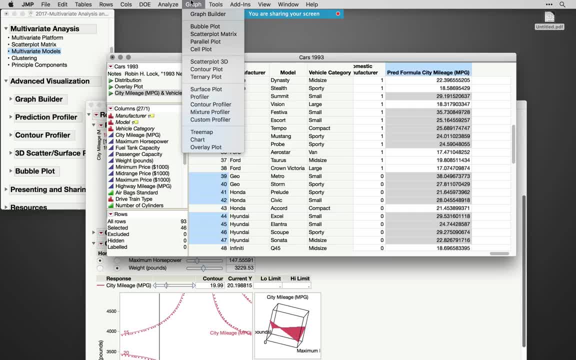 And so you can profile and you can see, and you can see that there's a graph that's actually a profile, And you can see that there's a graph that's actually a profile. Any formula, as long as you have those columns in your data set. 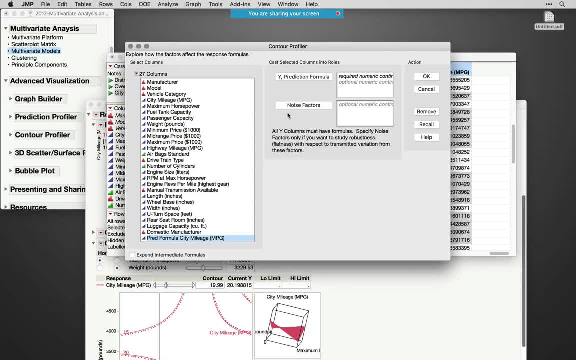 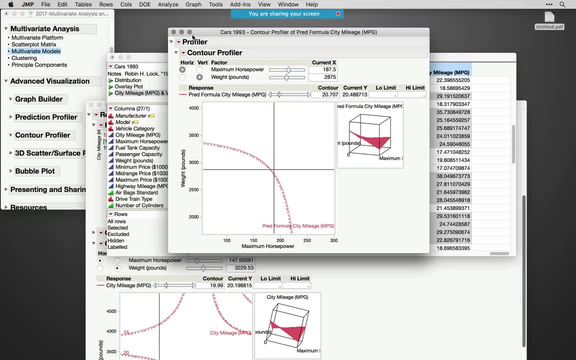 Similarly, we can go to the contour profiler. I can click that in with my predicted Y-score And this is the same contour profiler. So these profilers exist for any models you have, So it doesn't have to simply come from the Fit Model platform. 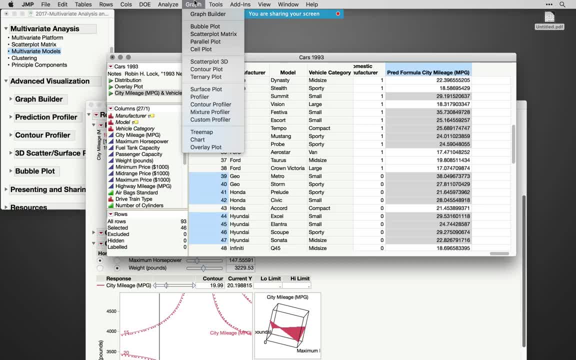 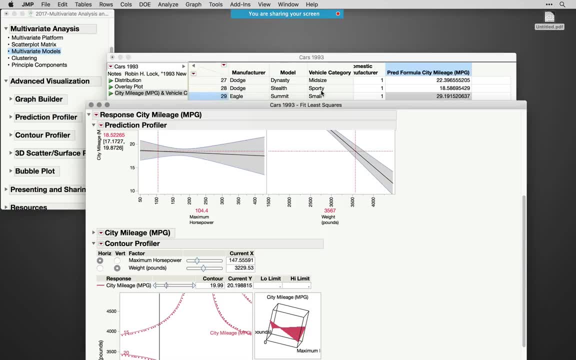 any time you have a model that you can profile and you want to understand the surface of, Similarly, the surface plot, the same thing we saw before- you can simply access directly from the menu. So these are great ways of understanding those multivariate relationships. 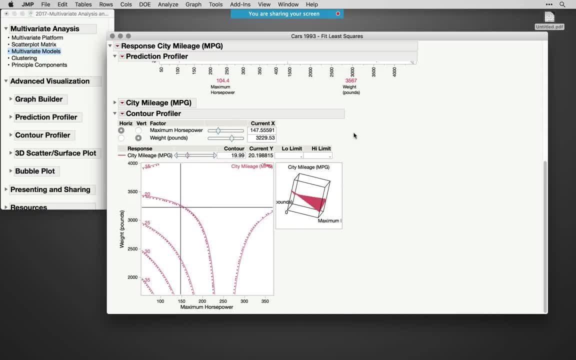 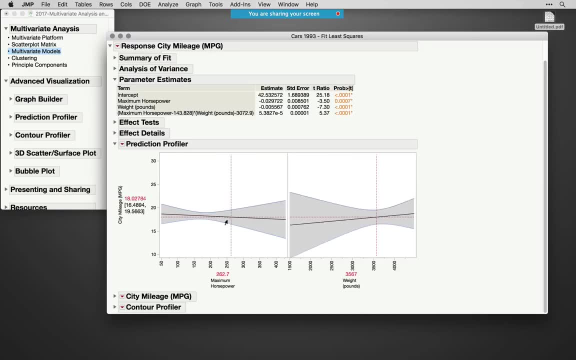 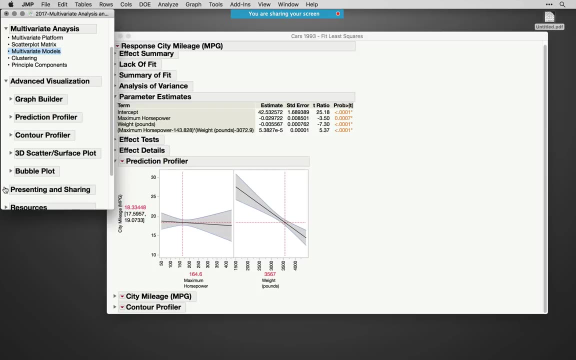 And certainly if you've never seen a contour plot before, or even the surface plot, they might look a little mysterious. but I certainly invite you to play with them, because especially the prediction profiler gives you an incredible way of understanding these relationships. Now again, we're not always doing this just for ourselves. 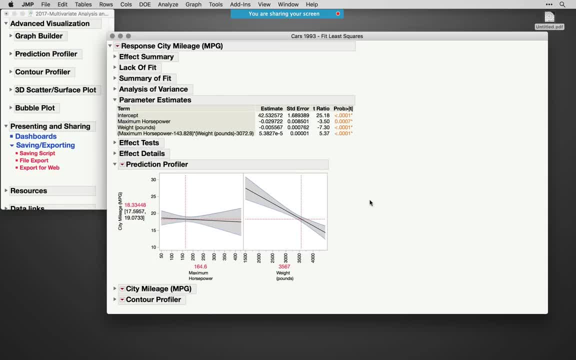 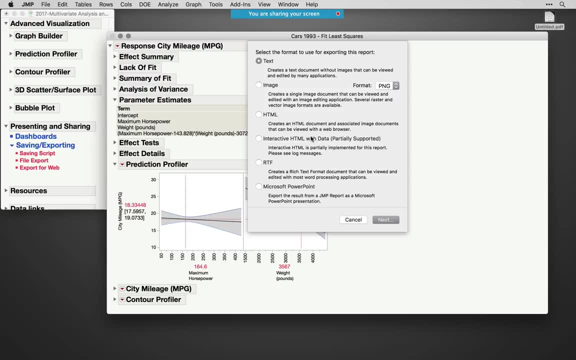 We want to share these things and we want to make them available to others. I always like to mention exporting your Fit Model output or using File Save, As on the PC, you can save this out as interactive HTML. Now, of course, the 3D plots aren't going to be able. 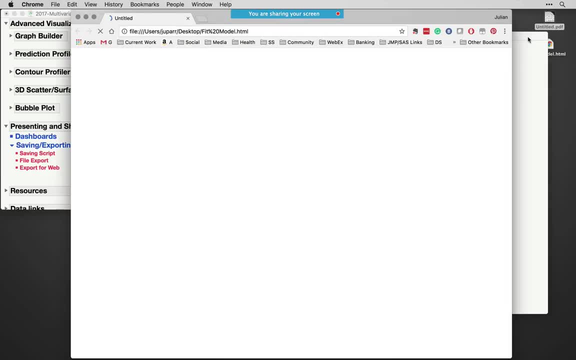 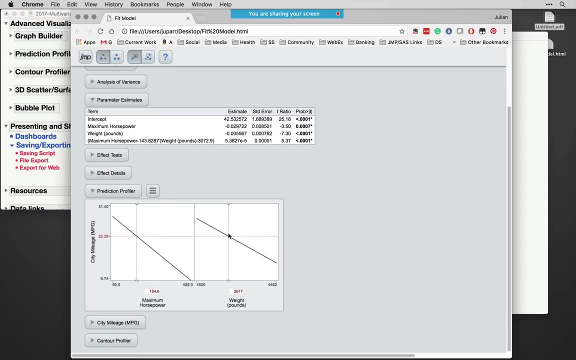 to be saved out as interactive. Unfortunately, those are very difficult to render on a web browser, but your profilers are, And so this is a profiler that you can share, especially if you're publishing a journal article or if you simply need to share it with those people. 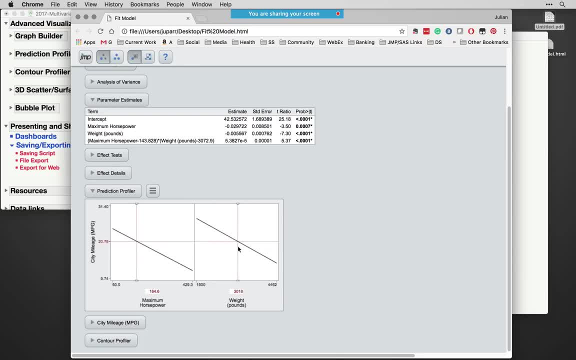 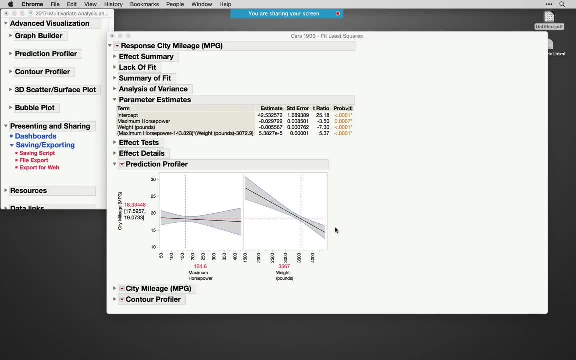 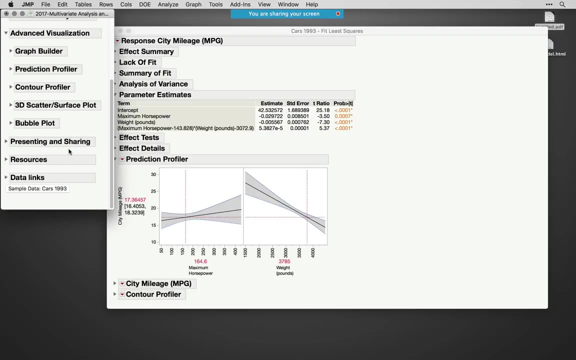 who don't have Jump. If you need to explain what a interaction term is in a multiple regression, I highly encourage the use of that profiler. It's probably the single best way of communicating that result. So be aware that that is there. So there were a few other things we didn't get to. 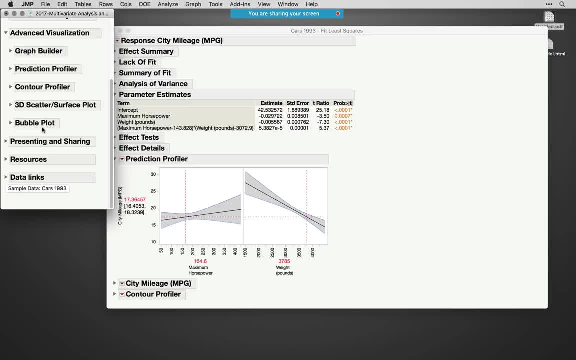 unfortunately, We're coming up on the end of time and I want to make sure I stop and take some questions. But bubble plots, I'll just mention, are another way of visualizing high-dimensional data And we're not going to be able to talk through. 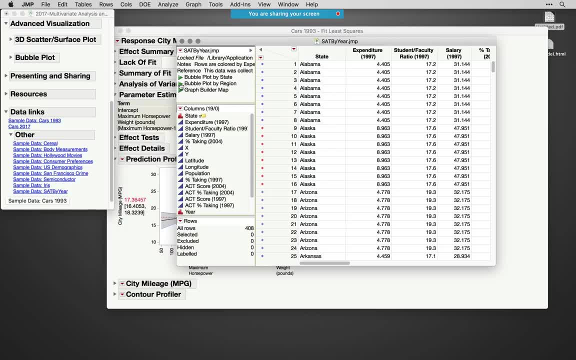 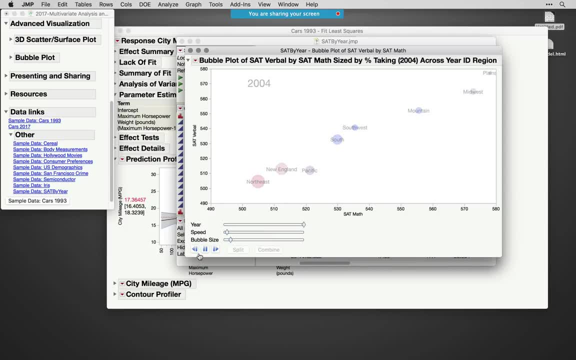 how to set it up. but just to whet your appetite, I'll pull open. what a bubble plot is. These are looking at SAT scores. These are looking at SAT scores by year, And so these are for the different regions of the country. 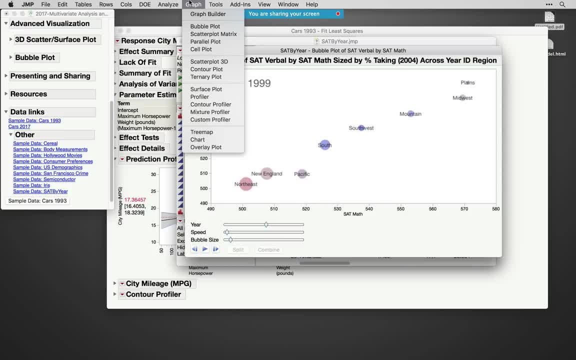 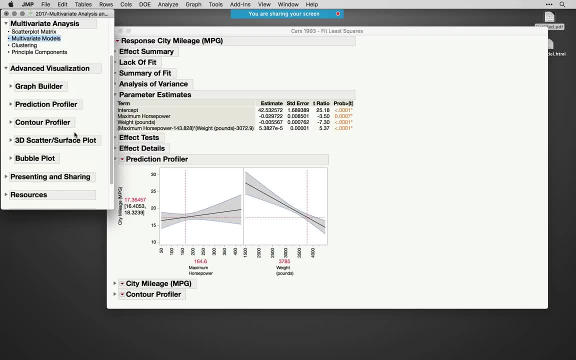 Bubble plots basically let you look at changes over time, And so they're a great option under graph bubble plot, And so we have other webinars which cover some of those things. But certainly be aware that there's beautiful visuals in Jump, well beyond the ones that are simply shown. 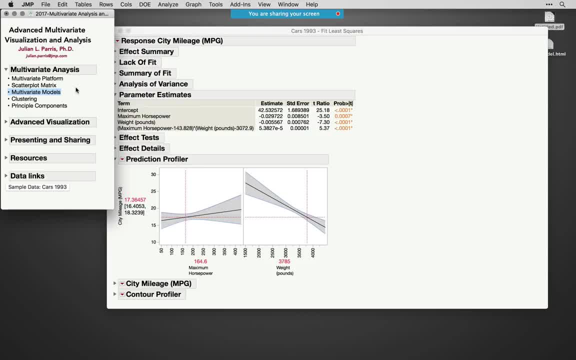 when you do analysis output. So I'm going to pause here and see if, Mia, any questions have come in with anything I've shown thus far. Hi there, Can you hear me? Yeah, Great job, Lots of very exciting visuals there. 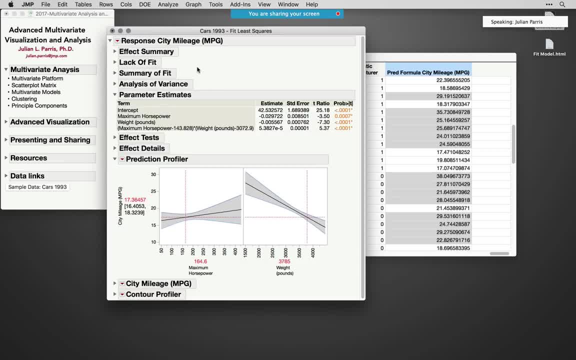 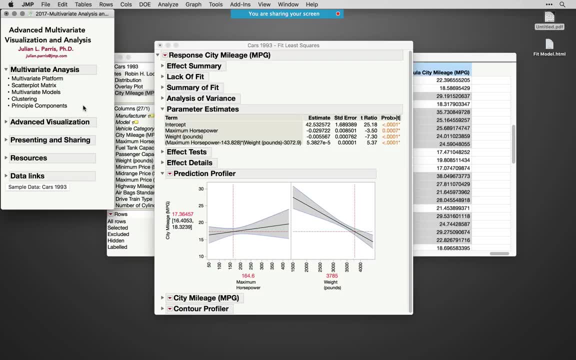 Just a quick question on other multivariate procedures for multivariate analysis. So in the dimension reduction sort of realm, can you really just show, like PCA and factor analysis and clustering, at least just how to access them? Absolutely So under multivariate methods, the principal components? 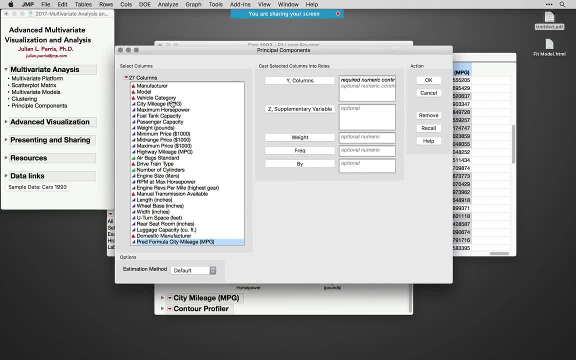 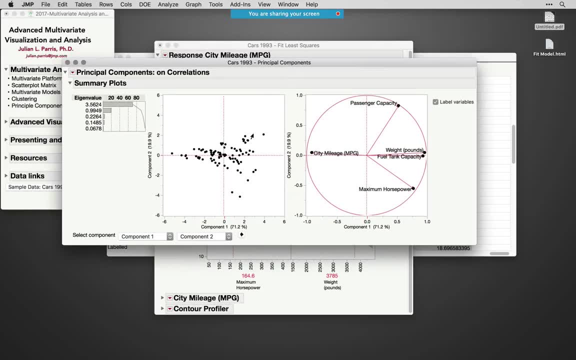 is the second option. PCA is very useful when you have a space of variables that share correlations, And so I'll take those variables that we used before, and of course, they're correlated. What PCA lets us do is reduce the dimensionality to independent principal components. 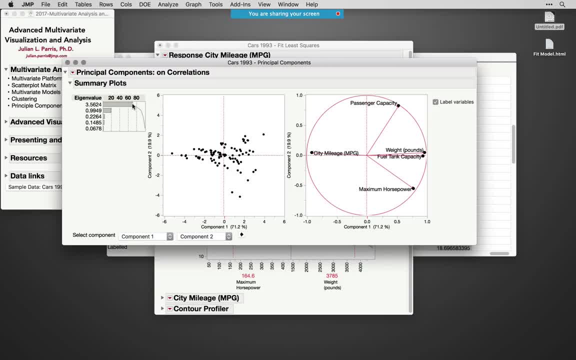 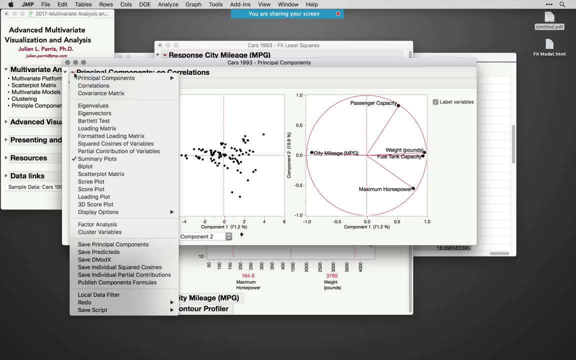 And so what we're looking at very briefly here is the proportion of the total variation in those five variables that get captured in the first component, and then the proportion in the second component And the way you might use these. there's plenty of options you can see. 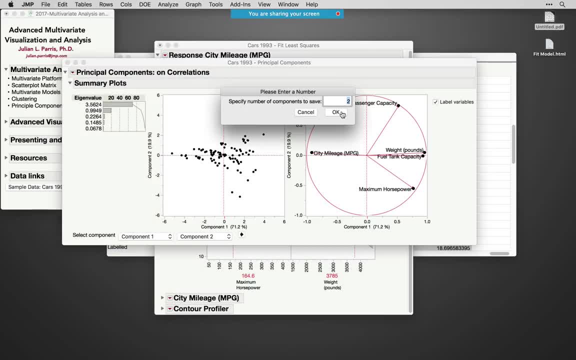 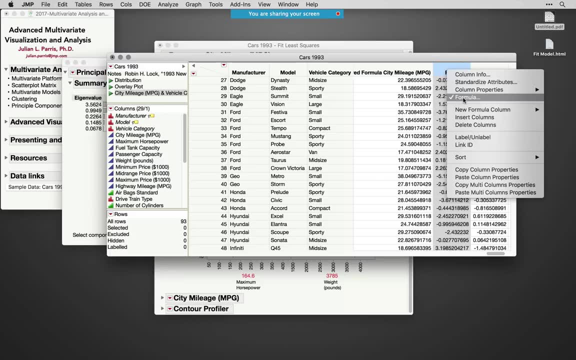 is saving your principal components, And I'll say I want to save two to the data set And you can see what these literally are are, for each row in the table, the value on each component, And the component is simply a linear combination. 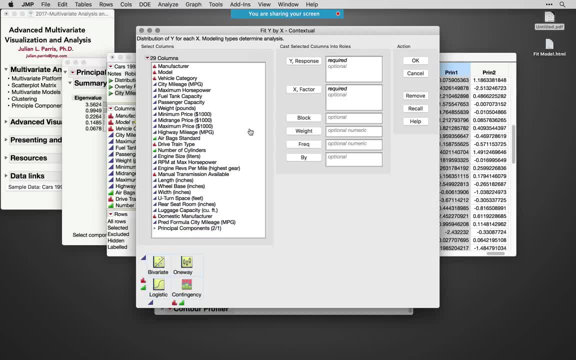 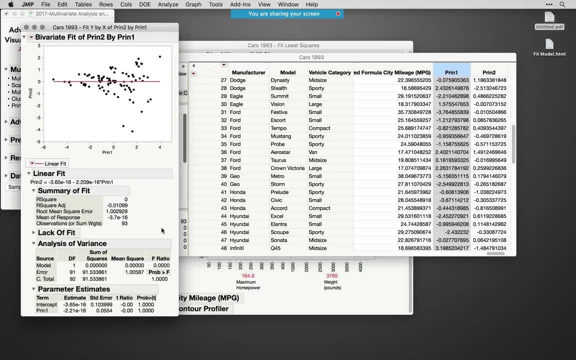 of the input variables And, as I mentioned, these are actual independent linear components. So if I take them in a fit Y by X, they actually won't have any relationship straight across zero. So independent components of variation. Now you can also go into factor analysis. 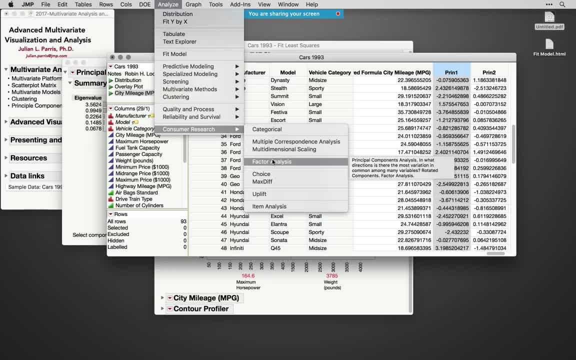 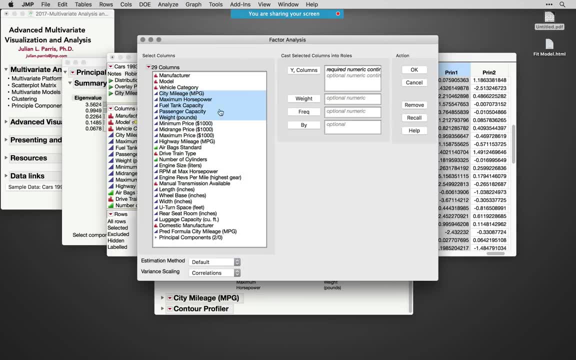 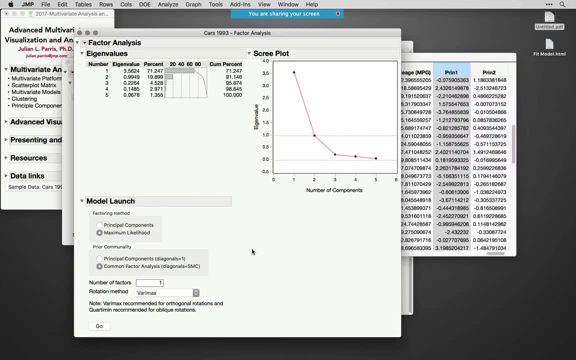 that's under consumer research, Factor analysis. Factor analysis, like principal components, works on extracting variation. It does it on the basis of shared variance And the idea with factor analysis is typically trying to understand or extract underlying factors that contribute to these observations. 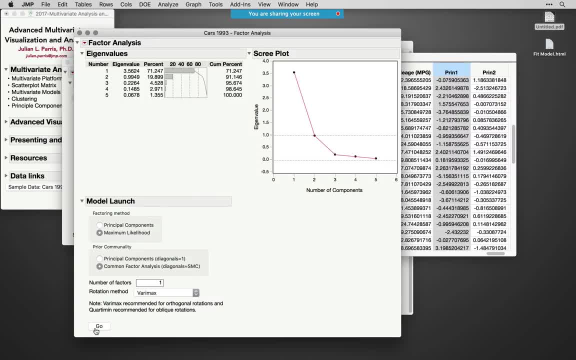 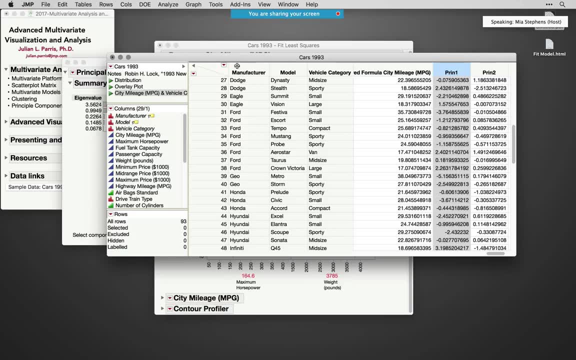 So not simply reducing the dimensionality, but finding something latent in the structure, And so lots of different options there And as far as- Oh yeah, Before you go on to clustering- Yeah, So I encourage you if you have any questions. 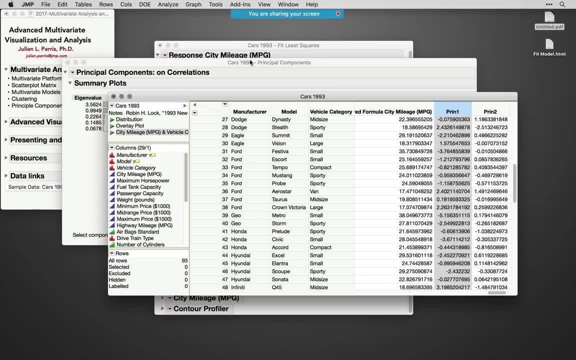 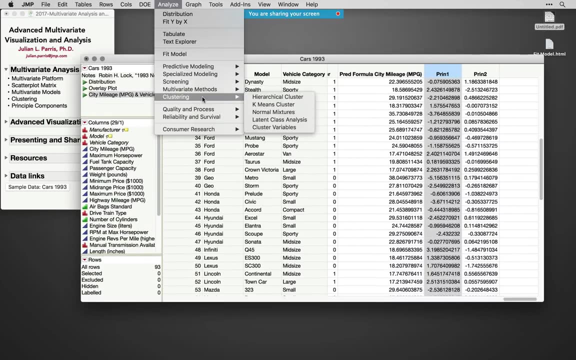 Julian will address the question about clustering in a moment. Please record in either the chat panel or the Q&A panel. Yep, excellent, And so clustering. one of the other ones I was going to show is a slightly different approach, So this is taking the rows in your table. 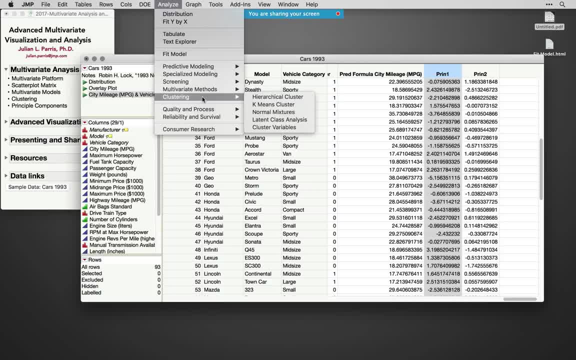 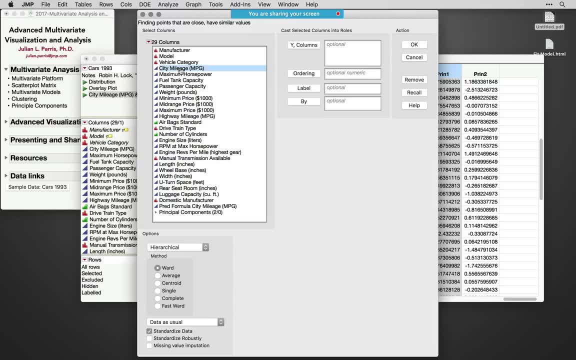 and finding out which ones you believe are similar on the basis of some criterion. And so there's a number of different clustering methods. I'll just show one so you get the idea. We'll start off with hierarchical clustering and we provide which variables we wish to identify similarity. 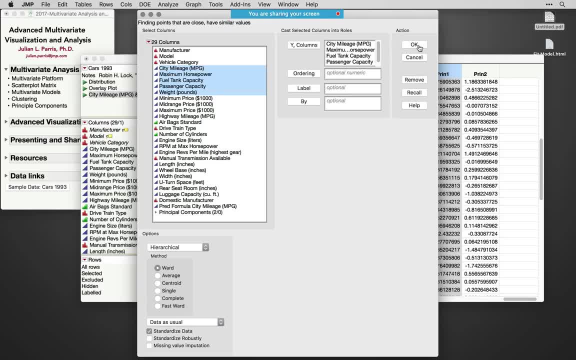 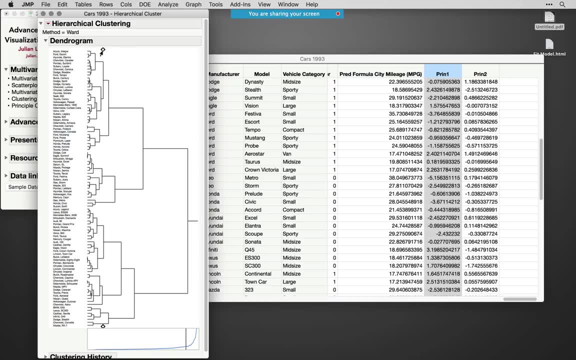 among the rows on the basis of: I'll click this into Y, I'll click OK. The rows in the table now are all here And the dendrogram is showing the closeness based on that iterative clustering. And so if I take some number of clusters, 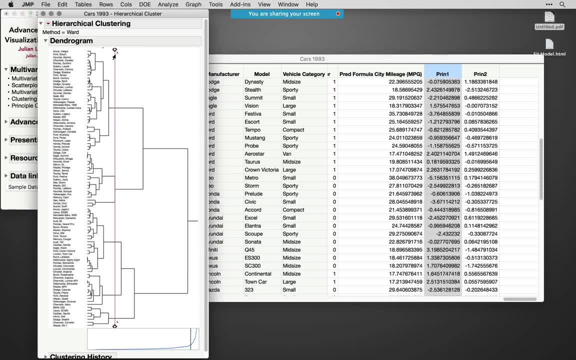 let's say five, and I did that by just dragging this little diamond around. I'm going to color the rows by their cluster, And so there's a big group of them here that are similar on the basis of those variables, And so you might add a number of them. 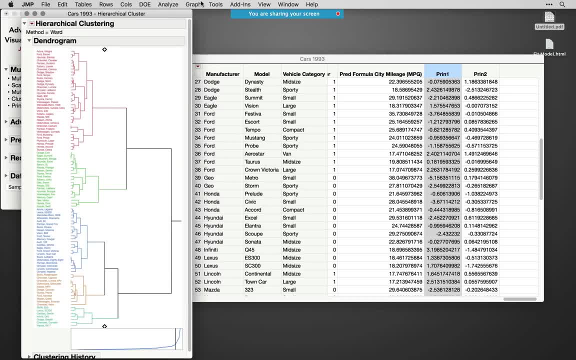 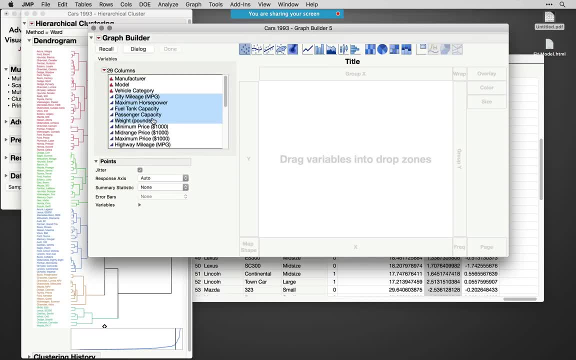 and you might ask what is similar on the basis of: So in your graph builder, here's a great way of visualizing that similarity. You remember those parallel plots I showed before. We can make them in graph builder just by dragging the variables we want to the x-axis. 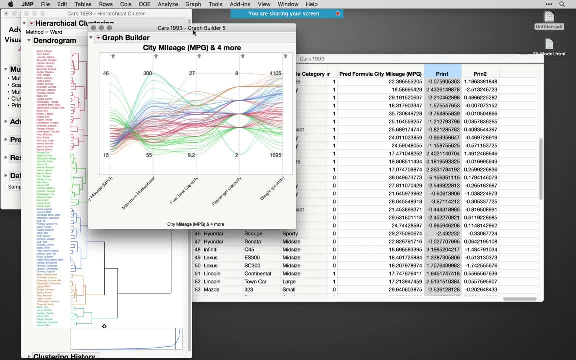 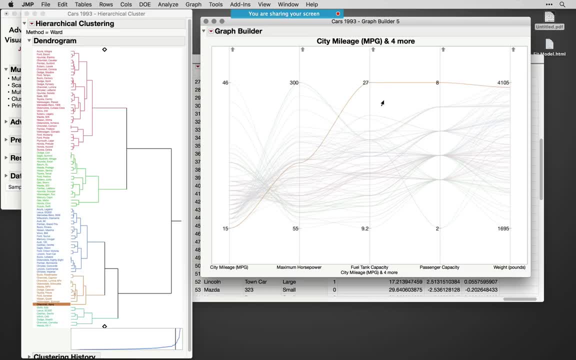 and clicking on the final option, the parallel coordinates, And just like I showed you before, each one of these lines is a particular car. So that's the Chevy Astro again, And we're looking at how high or low each car is on those variables. 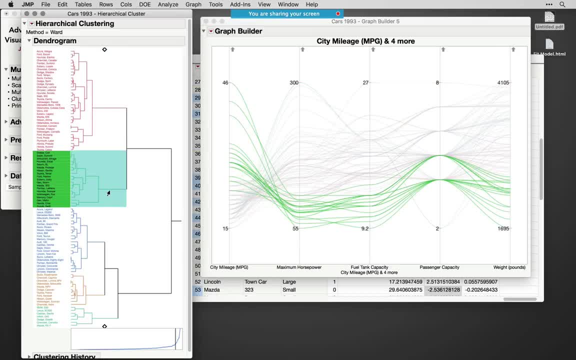 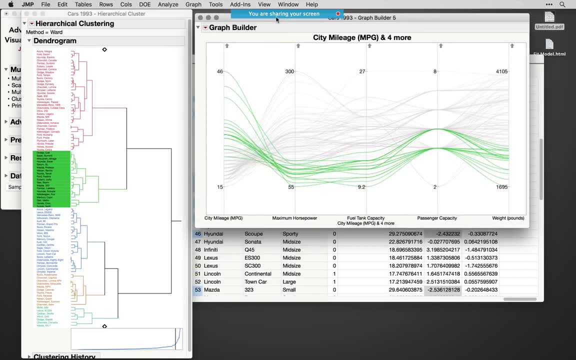 But now if I grab a cluster notice, they share the profile, And so if I grab one of those clusters here, you can identify what the attributes are, And so that's clustering. That's cool, Okay, so we do have a couple of other questions. 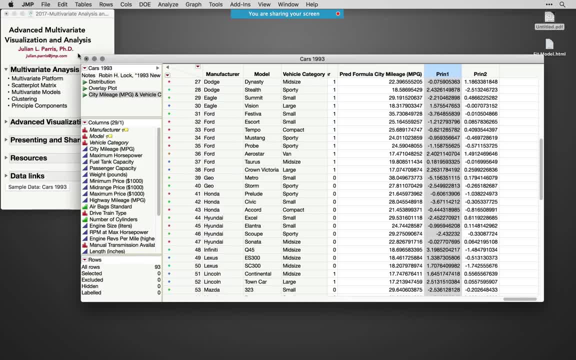 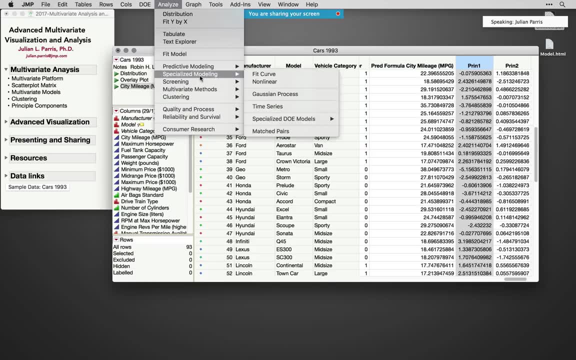 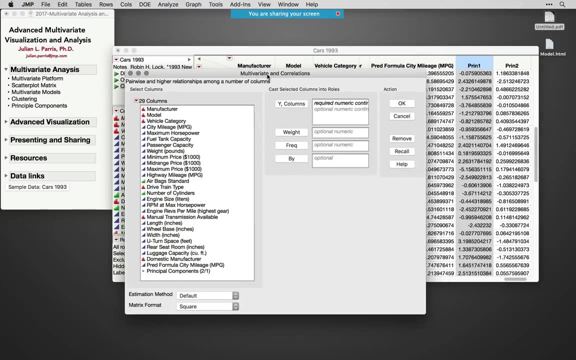 Absolutely. One question is: how do you include categorical variables in the multivariate platform? Good question. So multivariate- right here, under multivariate methods, is only appropriate for numeric, So it's not going to be appropriate for categorical variables. Now, that isn't to say there aren't analyses in JMP. 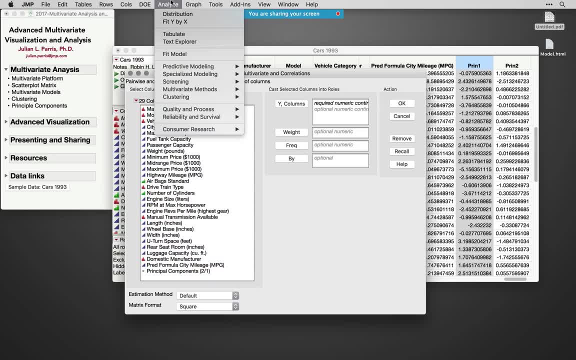 that are multivariate analyses that are situated for categorical outcomes And so under clustering, even hierarchical, is a good example that can take any variable type or latent class analysis, which is a type of clustering that specifically, is about looking at clusters based on categorical outcomes. 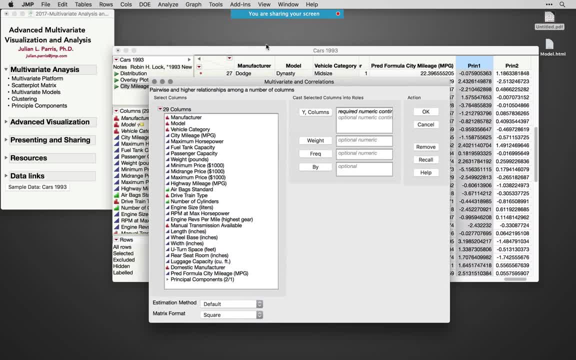 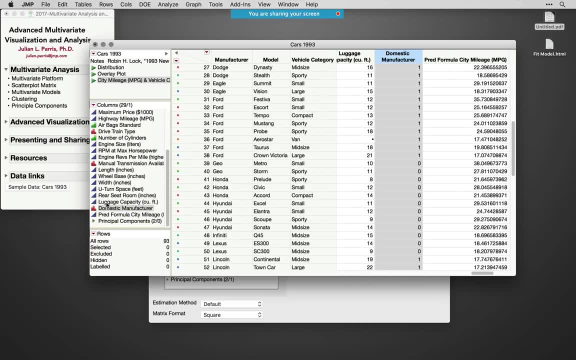 But, that said, multivariate is not built for that type of analysis. Now that isn't to say you can't trick it. Sometimes, if you notice in my dataset- domestic manufacture- even though we were treating it as categories, it actually is a numeric variable. 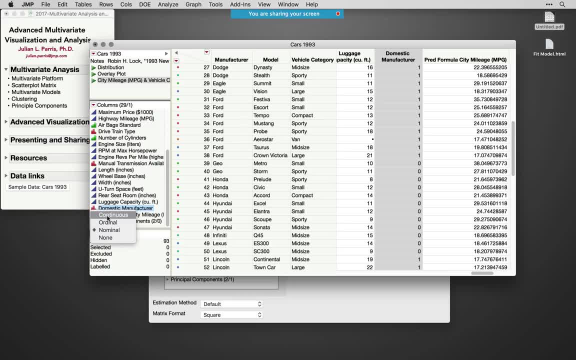 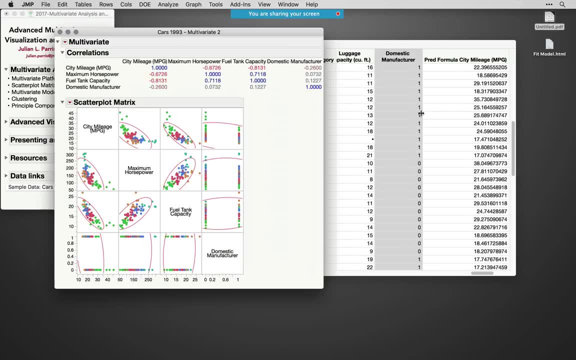 So if I click on that red triangle and tell JMP, even though this is categorical, treat that as continuous. I can then use it in the output. So I'll take some of my variables and click it in So you can trick JMP. 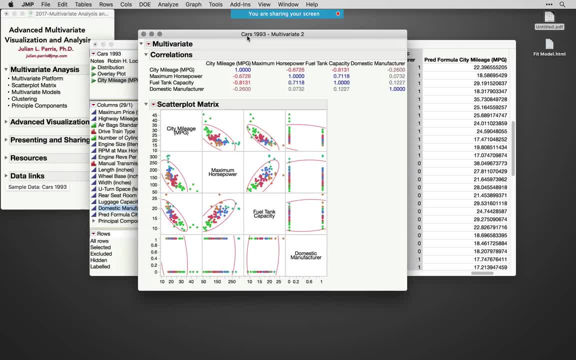 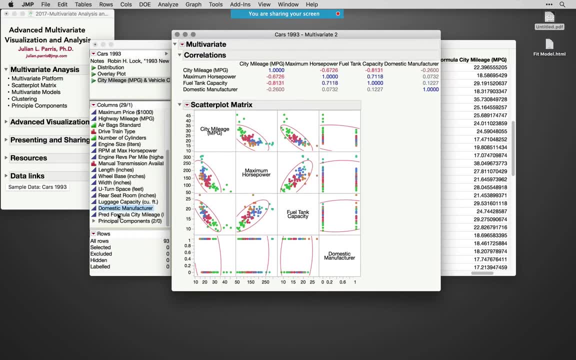 I don't recommend typically doing that. Sometimes things will be okay based on sort of symmetries among analyses, But I wouldn't recommend doing that Sure And for an ordinal variable. so there's a question about good, very good, moderate, then you can do the same thing. 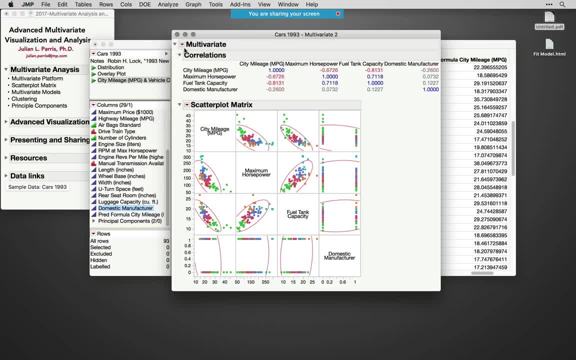 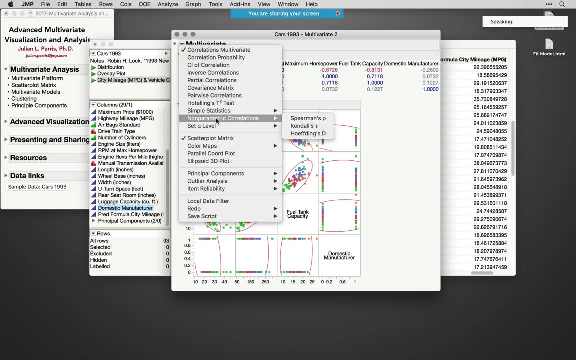 And then there are other correlations that are appropriate under the top-net triangle. Correct, That's right. So you'll notice there is the non-parametric correlations here. Great, That's right. All right, So I know we're running low on time. 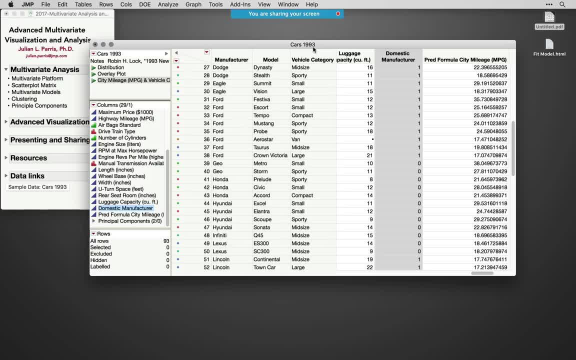 And we've got one more question: Can you once again very quickly show how to save the fit model results as an interactive model, As an interactive HTML? Absolutely Yeah. So I'll just recall what I had done before And I'll produce that factor: profiling profiler. 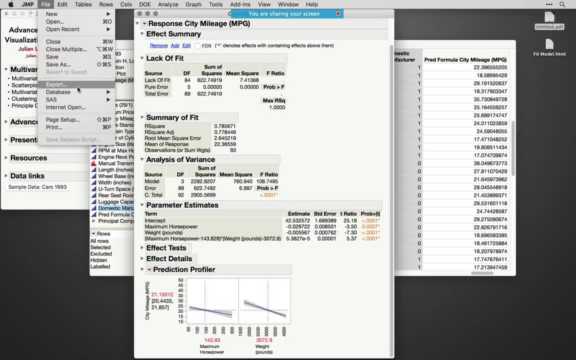 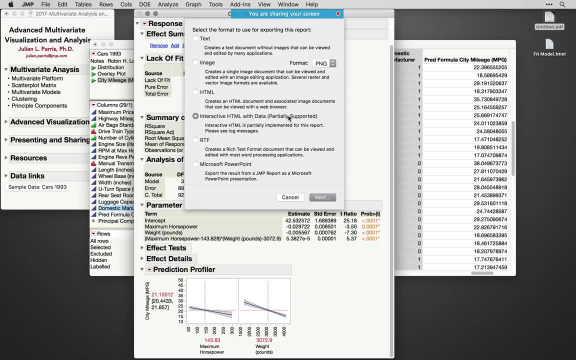 So on the Mac it's going to be File Export. On the PC you'll do File Save As Once you invoke either of those, there is the interactive HTML with data option. So when you select that and save it, what that saves for JMP is an interactive HTML. 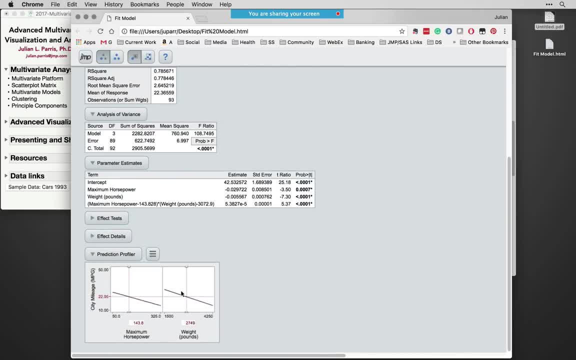 It actually does contain your data, So we always just like to caution you if there are sensitive data that you shouldn't be sharing with others. be aware that for this to be interactive, the JavaScript here has to access the data, And the data is actually a part of this page. source. 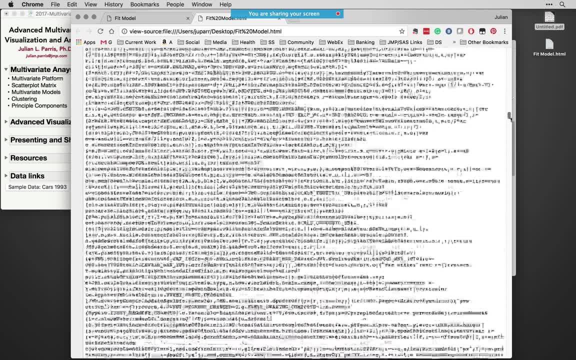 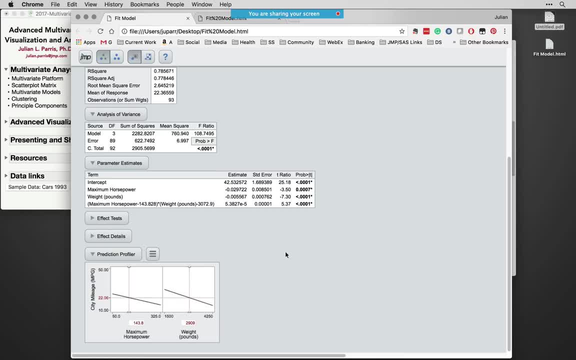 It's cryptic And it's probably not easy for people to recover, But it's in there, So just be aware. if it's very sensitive, interactive HTML is not the right method for you. Great, Can we take this a step further and just very quickly talk about saving a web report? 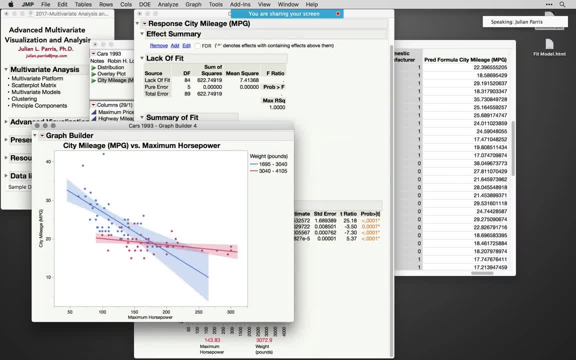 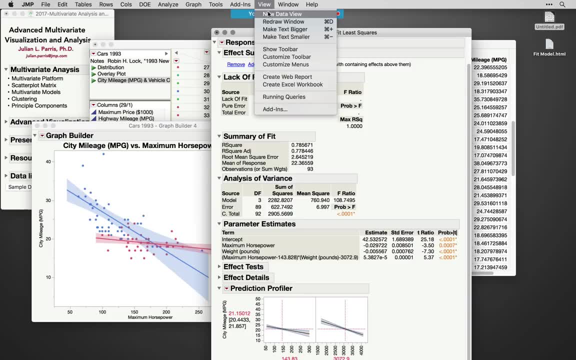 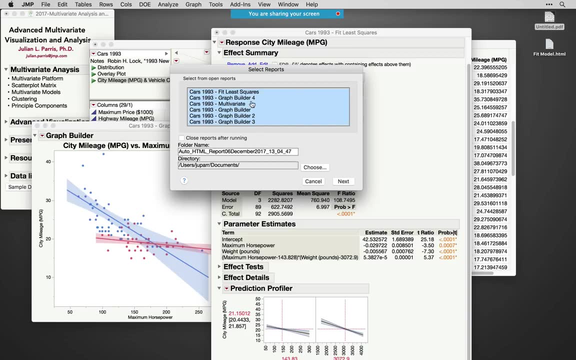 Absolutely Yeah. So we had a number of things that we created here, even, And. so what, if I wanted to, We package these together in a single place, And so under the View menu, there is this Create Web Report option, And what this asks is for us to grab whatever outputs we created. 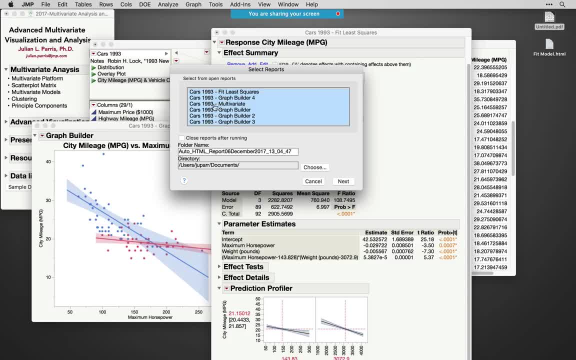 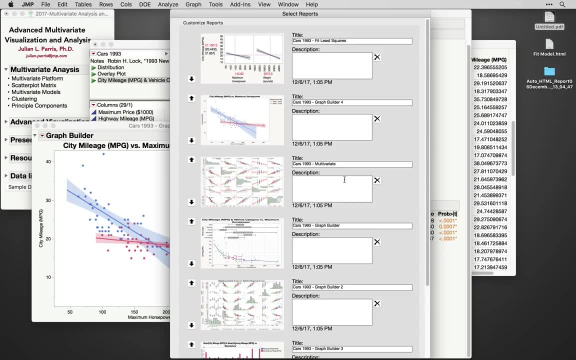 Those are all the reports, including multivariate and least squares, And what we're going to do is build a package And I'm going to tell JMP to stick that package directly on my desktop. I'll click Next. JMP gives me the option to title these specific things. 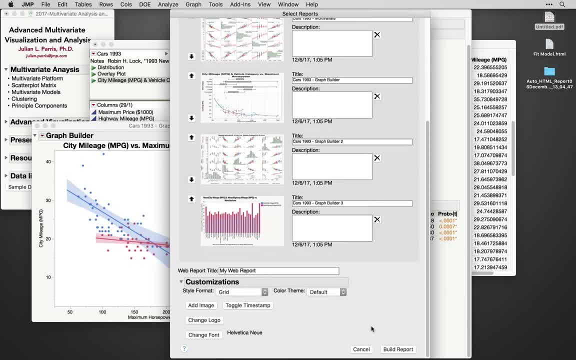 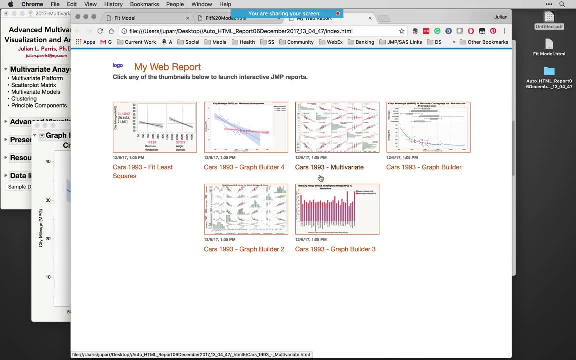 I'll just leave them as the defaults. Lots of customizations in terms of how you want to do it. But I'll click Build Report And what JMP does is assemble all of these outputs together, all the interactive HTML versions of them, and makes a web report. 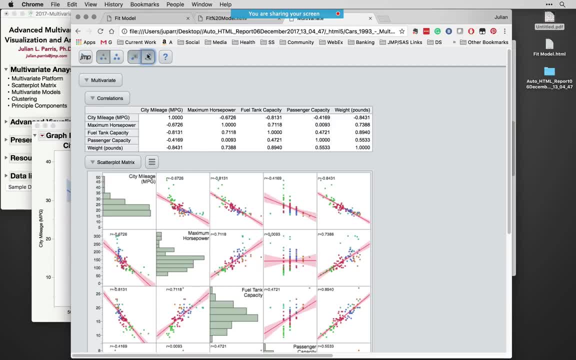 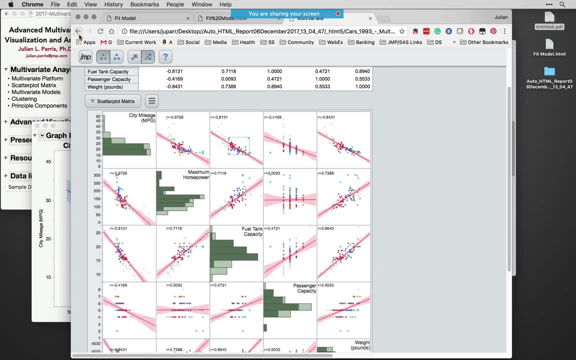 And so I can click through this title slide And everything, just like we've seen before, is still interactive, And so I love these multivariate outputs when they're interactive online. So the web report is a really great way of capturing all of your work together.